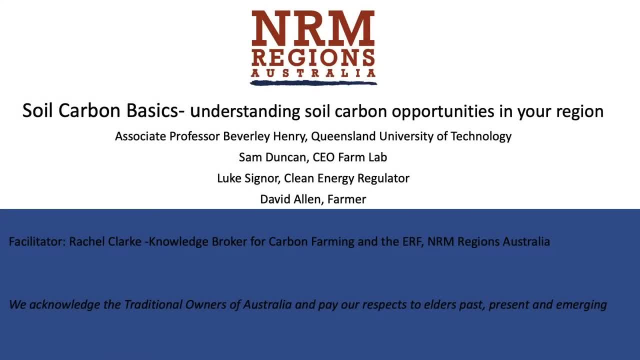 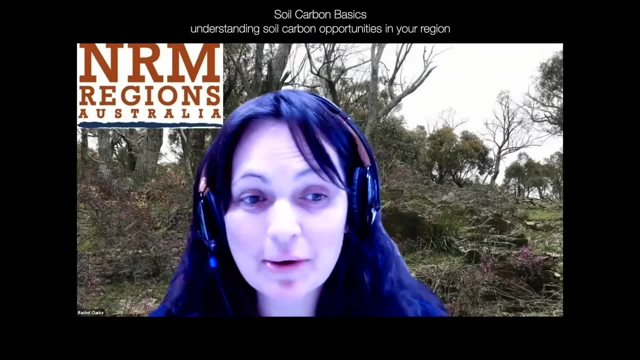 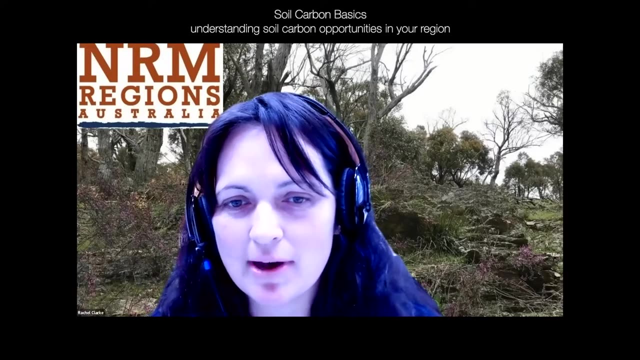 Hi everyone. I'm hoping that everyone can hear me. I'd like to welcome everyone to the NRM Regions Australia Soil Carbon Basics webinar. My name is Rachel Clarke and I'm the Knowledge Broker for Carbon Farming and the Emissions Reduction Fund with NRM Regions. 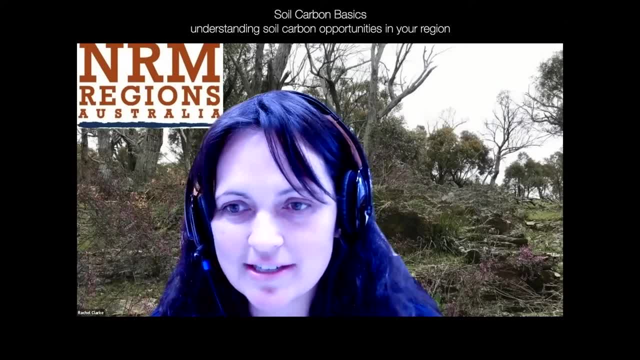 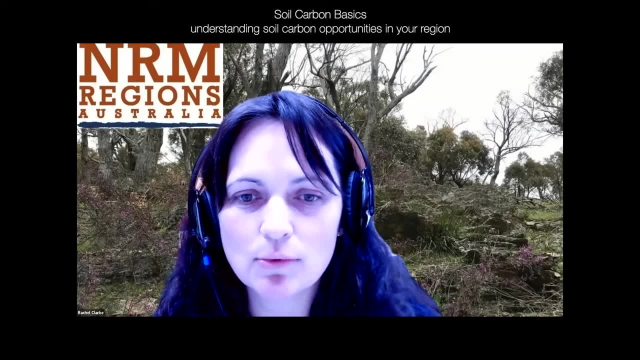 Australia, the national peak body for regional NRM organisations across the country. I'd like to start the webinar by acknowledging the traditional owners of the land where I am today. It's Ngunnawal, Ngambi and Narrago land in Canberra, and I'd like to thank the 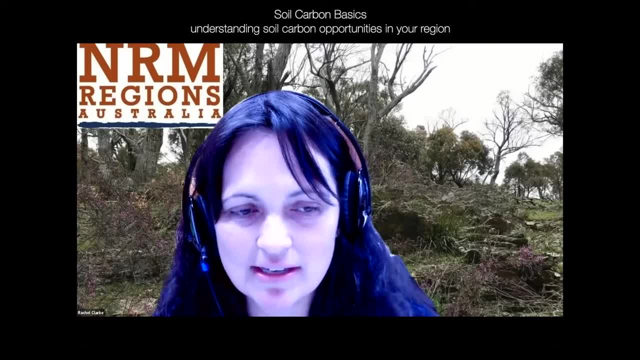 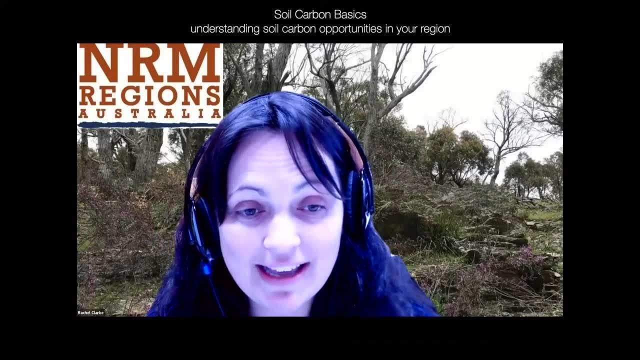 traditional owners for their careful custodianship of country for thousands of years. I'd also like to welcome any Aboriginal and Torres Strait Islander people who are joining us today. I'd also really like to welcome and thank our four fantastic speakers, who I'll 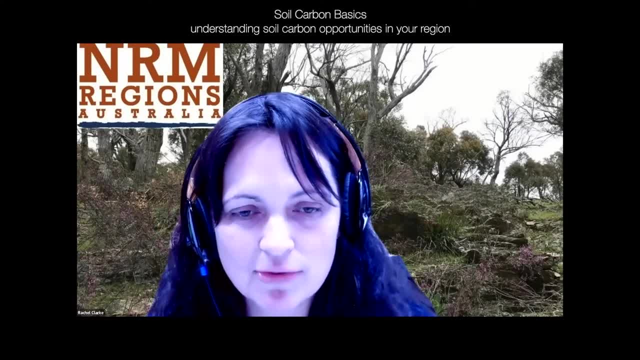 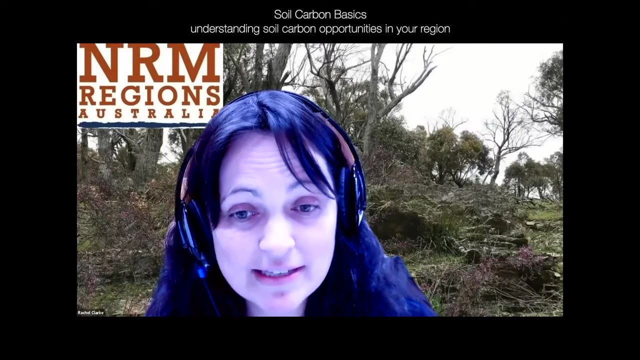 introduce properly shortly, and Rachel Morgan and Kate Forrest from NRM Regions Australia who are helping out with the webinar. Finally, I'd like to welcome everyone else, especially all the staff from regional NRM organisations across Australia, for joining us. As you all know, we're here to take part in a webinar I've called Soil Carbon Basics. 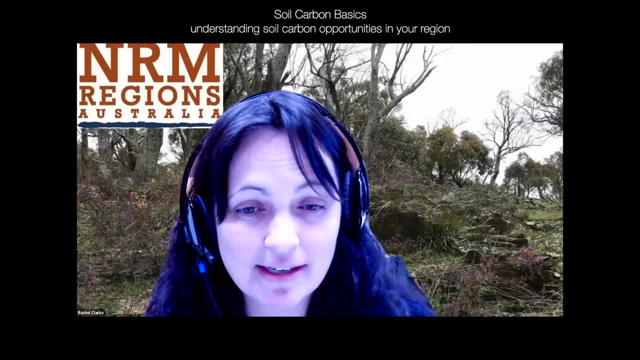 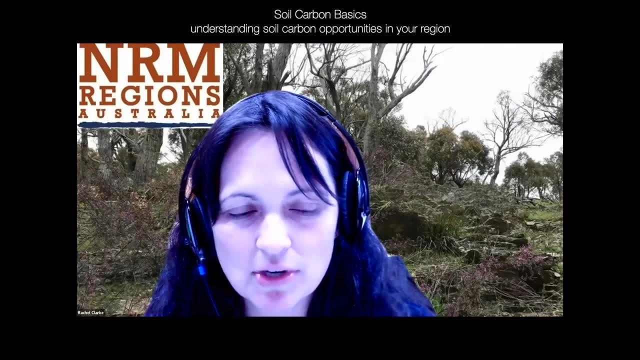 In all areas of carbon farming there's a lot of legal and technical complexity, and I think soil carbon is almost the most tricky to get across. Anyone can see, or at least imagine, the carbon that's being stored in a growing plant or a tree, but it's not nearly. 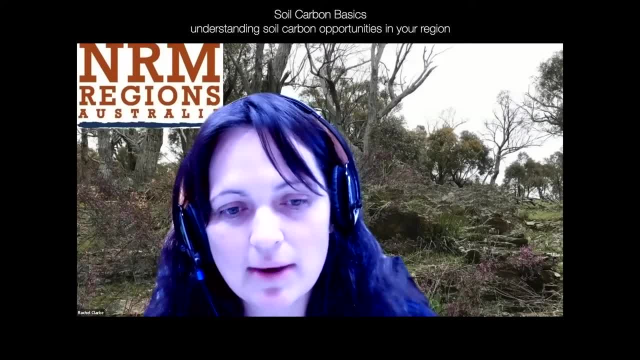 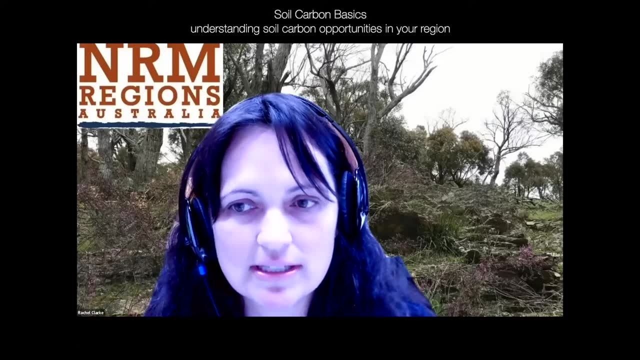 so straightforward with carbon in soil, So I'm hoping this webinar will help to demystify this process and to also help people to understand the potential opportunities for carbon sequestration in soil in different areas. And I'd also like to welcome everyone else, especially all the staff from regional NRM Regions Australia who are joining us today. I'd also like to invite everyone else, especially all the staff from regional NRM Regions Australia who are joining us today. I'd also like to welcome everyone else, especially all the staff from. 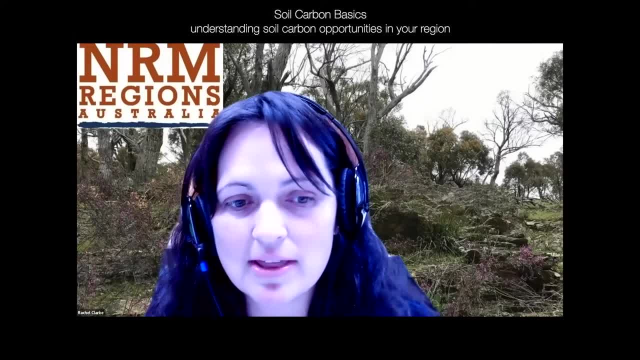 regional NRM Regions Australia who are joining us today And, I think, the potential opportunities for carbon sequestration in soil in different areas of our community and soil types across Australia. I hope you might also get a sense of the what's in it for me, whether that means. 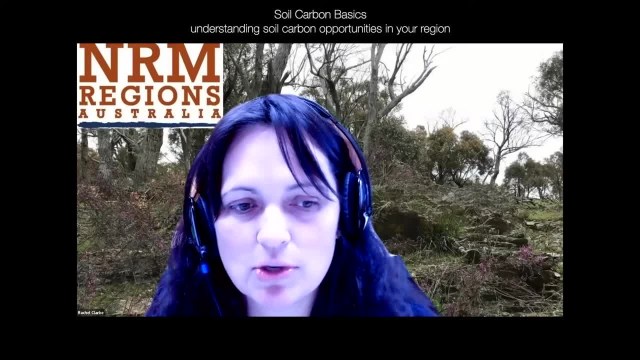 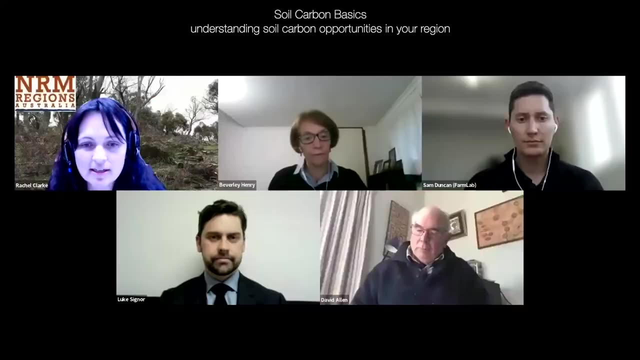 improved environmental outcomes, increased profits or a contribution to addressing climate change, to restoring more carbon in the soil. I really hope this has been an interactive webinar and I encouraged discussion, initially in the chat and then in the Q and A. So firstly to our audience, we'd like to hear from you in the chat. If you could, please tell us. 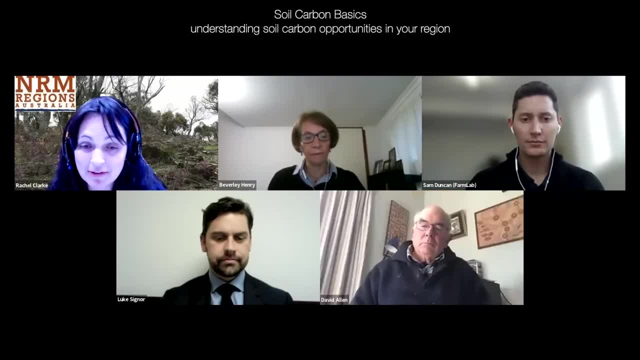 who you are and your organisation, if applicable, Where you're zooming in from today. you might like to include what people know about the landfill and what you're doing to help solve. what First Nations country you're zooming in from. You'll also find the chat at the bottom. 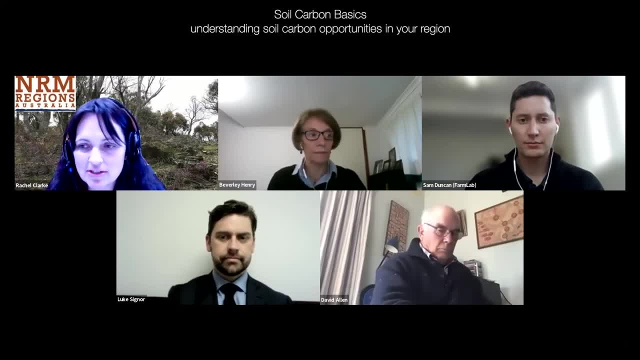 of the screen and you'll need to select all panelists and attendees to introduce yourselves. So I think Doug's mentioned his mic freezing, but um, yeah, if everyone else would like to to pop in where they're zooming in from today, then that would be fantastic. Shortly we'll also be asking: 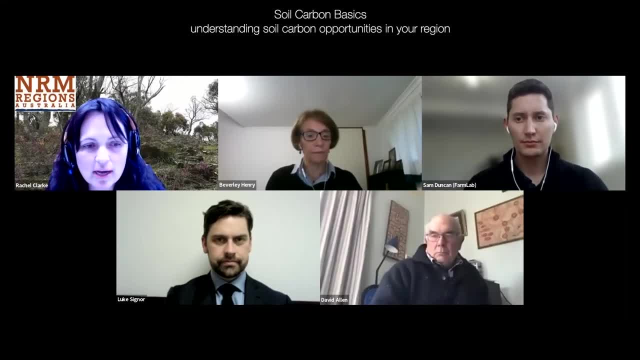 you to start posting your questions and thoughts in the Q&A. The Q&A button's usually right next to the chat button on your screen, so feel free to ask questions, upvote questions and provide answers and thoughts from your own experiences, if you have some. Thanks, everyone, that started. 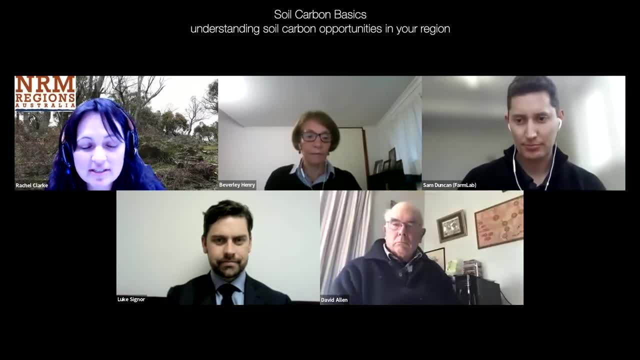 putting in where you're coming in from. today, too, I'd like to emphasize this is Soil Carbon Basics, so there's no such thing as a dumb or obvious question. If there's a question you're hesitating to ask, you can guarantee it's one that at least five other people are desperate to hear the answer. 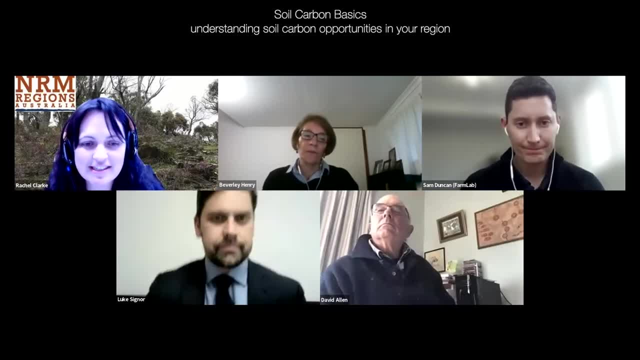 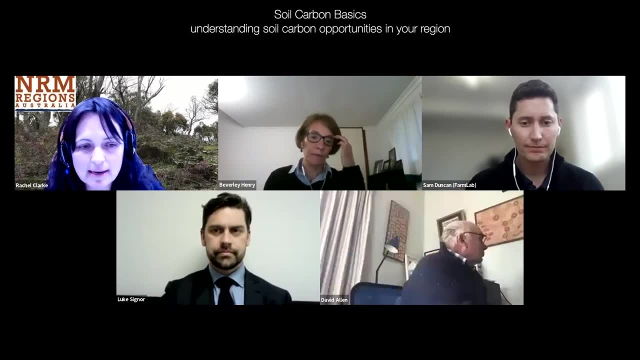 to. So please feel free to put your most seemingly obvious questions into the Q&A, and I'm sure many people will thank you for that. We'll be holding all questions until the end of the presentations, so please start posting questions as soon as they come to you and we'll get as many questions as possible we'll get to. 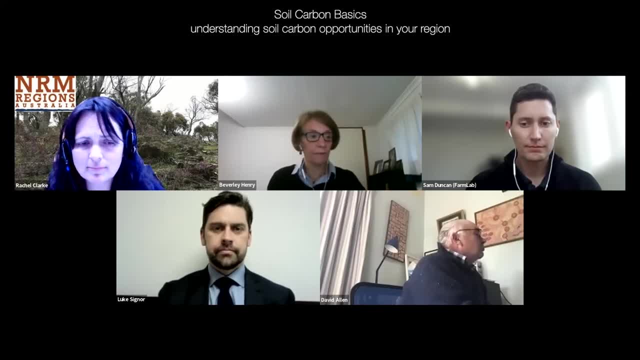 as many questions as possible at the end during our panel session. If there are links and specific resources we don't manage to provide in our discussion, we'll send those around with the recording. later I'll also be encouraging people to fill in a very short survey at the end. just 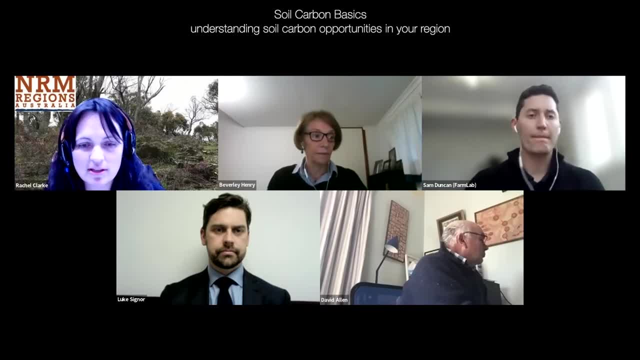 so you're prepared, so that we know how useful the session's been and whether there are things we can consider for future webinars. So to support us in our quest to understand more about soil carbon, how it's stored and the benefits it can offer, we're joined by four expert speakers. 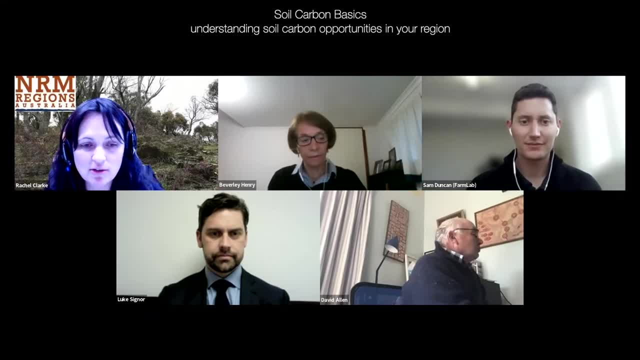 Associate Professor Beverly Henry from the Queensland University of Technology, Sam Duncan, the CEO of FarmLab. Luke Signore, the Assistant Manager of the Savannah Agriculture and Soil Team at the Clean Energy Regulator. and David Allen, a beef sheep and now soil carbon farmer from the Karangamite region in southwestern Victoria. All our speakers today are playing a. 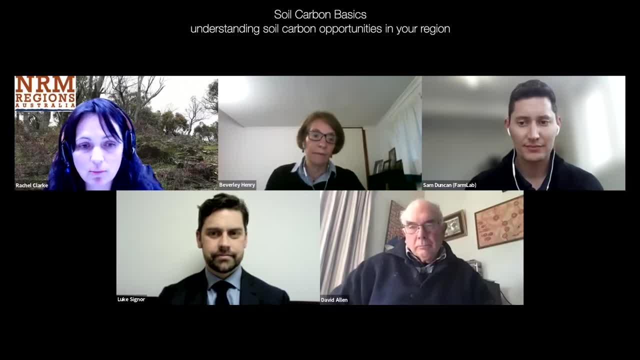 unique role in the early understanding of how soil carbon farming can work in Australia, so I'm really delighted they've been able to join us. So now I'd like to turn to introducing our first speaker. so, Beverly, you can think about sharing your screen now, and that's Associate Professor. 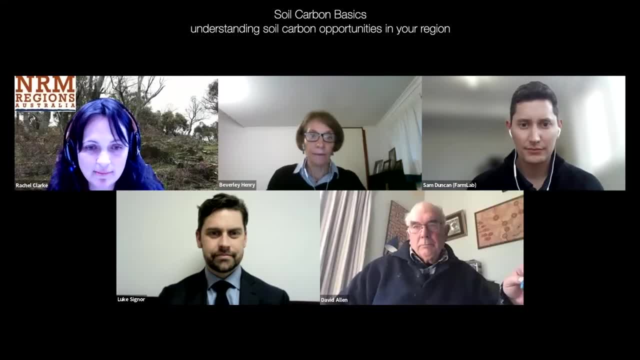 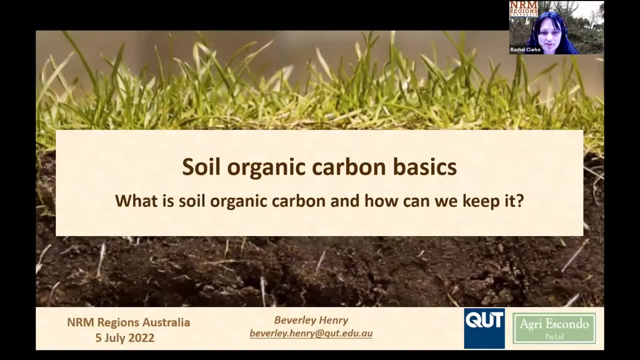 Beverly Henry from Queensland University of Technology. Beverly Henry has been involved in research, policy and industry roles across agriculture and land use sectors for 30 years. Her work has largely been in the areas of climate change, climate variability and environmental management in Australian and international research and committees. Thanks so much, Beverly. 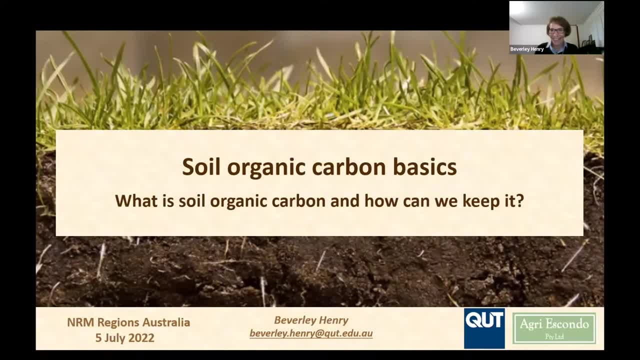 I just need to unmute. excuse me, You're unmuted now. Okay, thank you, and can you see my screen, Rachel? Okay, good afternoon, thank you, Rachel, and good afternoon to everyone. Firstly, I'd like to acknowledge the First Nations People's of the land from where I join you today. These are the Bundjalung people, and I pay. 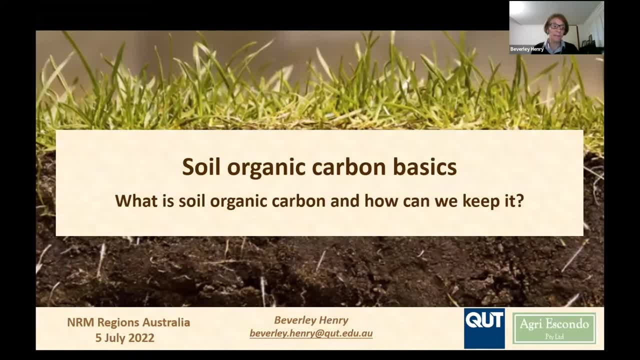 respects to their elders, past, present and emerging. I also acknowledge all other First Nations People online and wish you a great NAIDOC week. So I've been asked to speak to you today about the basics of soil carbon: What is, what it is and how we can keep it in the soil. I'm not 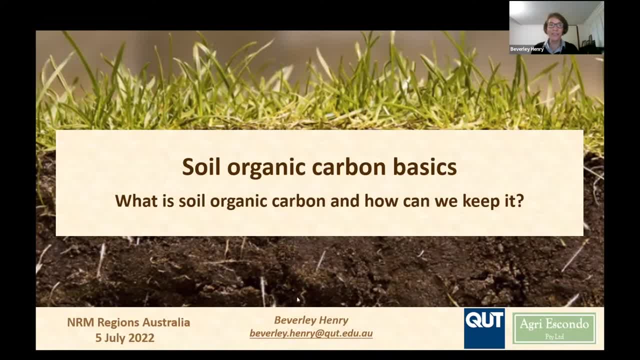 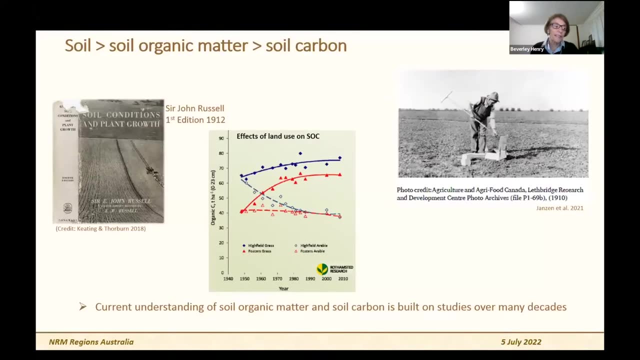 going to get into the details. I'll leave that to the experts. I'll leave that to the experts, But follow me as well. The first thing I'd like to. the first thing I'd like to do, though, is to note that, while soil carbon is getting an awful lot of attention at the moment, and mostly in relation to soil, 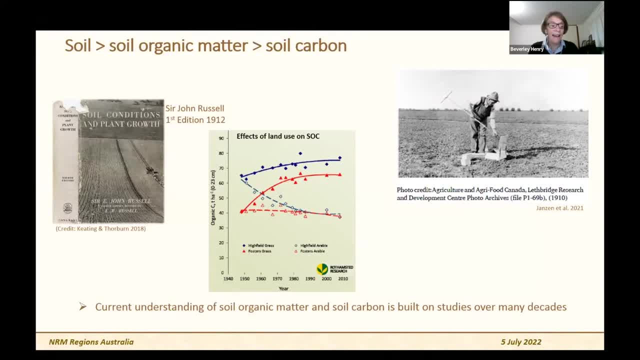 carbon sequestration and offsets and also some extent to address climate change mitigation and soil health for food security. it isn't new. Soil carbon has been of interest for hundreds of years. Farmers and gardeners have been very aware of the importance of soil organic matter for a very long. 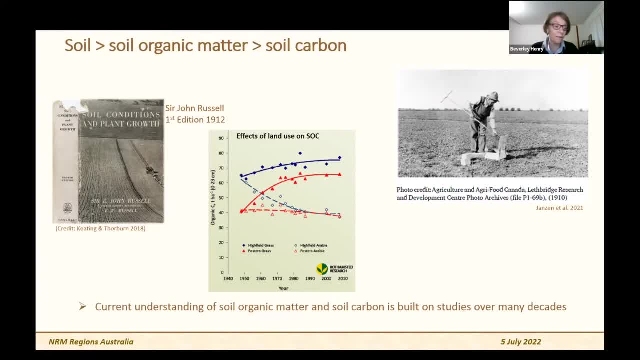 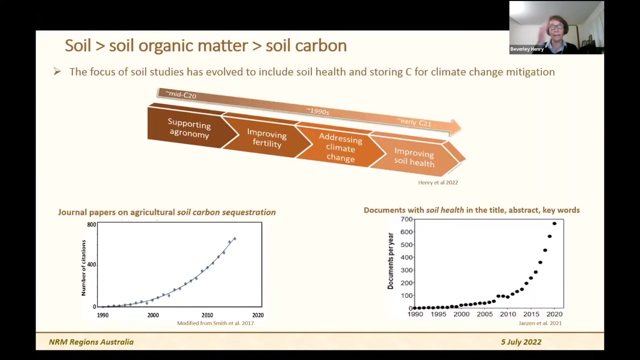 time, and it's been the subject of a lot of research, including some critically important long-term trials established at research stations some as long as ago as the 1840s. We've begun by providing some of our best records of what soil carbon is and how it cycles in soils, So there's a lot of science underpinning what we know, although there 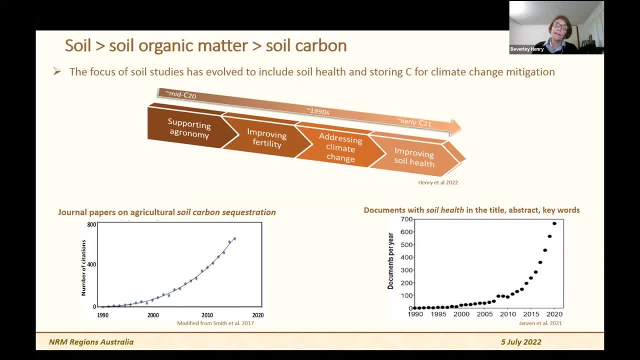 are still some questions to be answered. Initially, the focus was on understanding how soils and atmospheres support plant growth for production reasons, and this remains, of course, of fundamental importance, but i just wanted to just illustrate the rapid growth in interest in in soil carbon. the two graphs on the bottom of 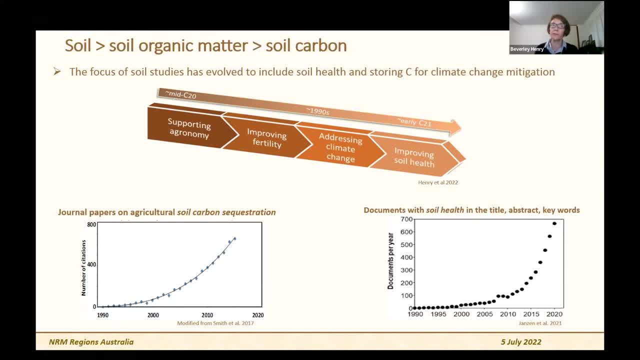 this slide show the growth in in number of papers published on soil carbon sequestration and the number of publications on soil health. so this is the basis for a lot of the interest that we have now, and no doubt some of the stuff that i present will be very familiar to a lot of you. but 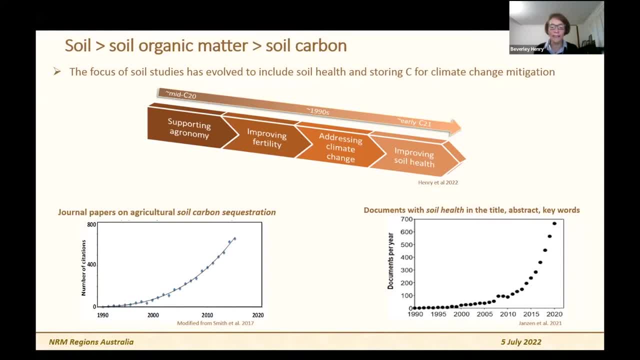 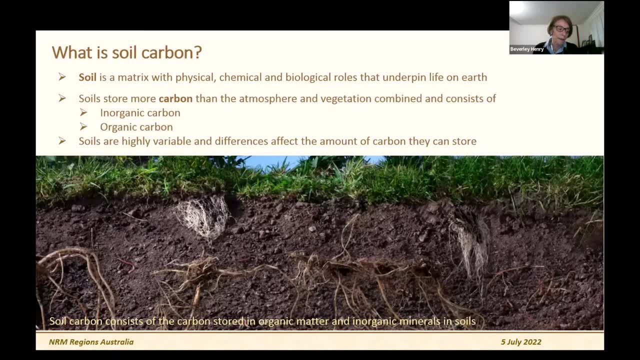 i hope it's not too basic and i hope it helps to get us all on the same page for the presentations to follow. so what is soil? carbon i mean? firstly, soil is a fundamental importance to life on earth. more than 99 percent of human food starts with the soil. 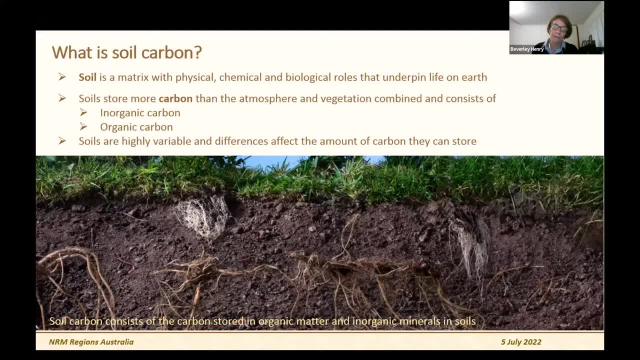 soil also stores a huge pool of carbon. it's estimated that there's around two and a half, two and a half billion combined. so soil carbon within the soil is important to the chemical, physical and biological functions that soils perform, and soil carbon includes both inorganic and organic carbon. the inorganic compound carbon is 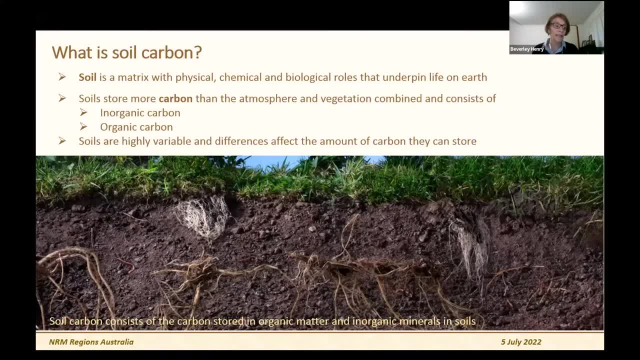 largely the carbon that's held in carbonate minerals. it's much more stable than organic carbon and much less influenced by management. i'll talk very little, or probably not at all, about inorganic carbon, but i'll focus on the organic component. so what is soil organic carbon? we talk about it a lot. 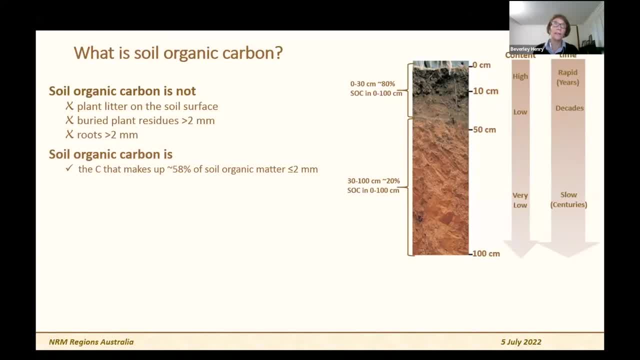 but one of the issues is that it's not always used consistently. i think there's some confusion that arises from the fact that we don't all talk about the same thing when we talk about soil organic carbon. soil organic carbon is not plant litter on the soil surface. it's not buried. 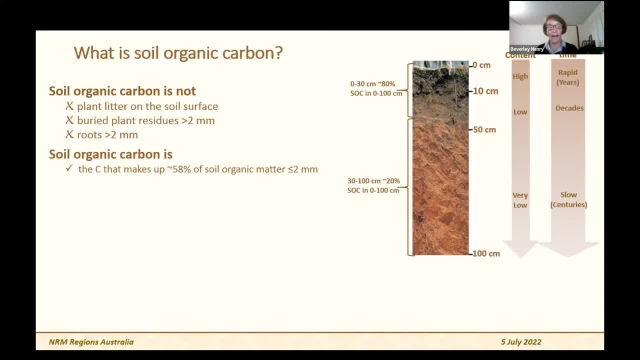 plant residues or bits of roots that are fairly large. soil carbon is the carbon that makes up a 58 percent of soil organic matter in the component that's up to two millimetres in size, So it's something that is measured in a very specific way. 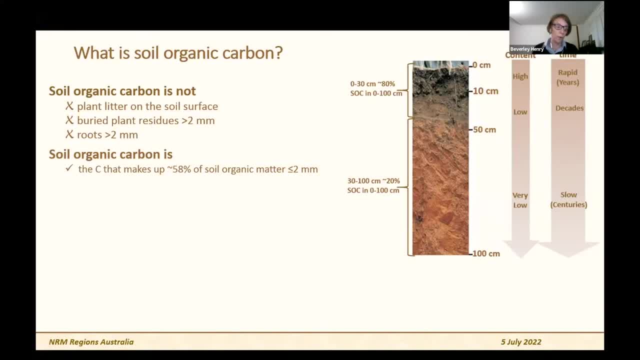 and accounted for in a very specific way, and because of the way we need to think about soil carbon, we just have to look a little bit to start with about how it's measured. So, because it's only in the less than two millimetre fraction, soil is firstly sieved. 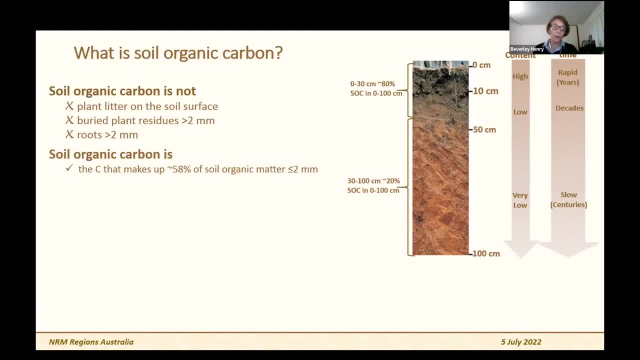 that removes the, the larger bits of organic matter that isn't counted as soil carbon. it also removes the gravel, and if we're wanting to account properly for soil carbon, we also remove any inorganic carbon chemically. So what's left then is bits of plant biomass that have been 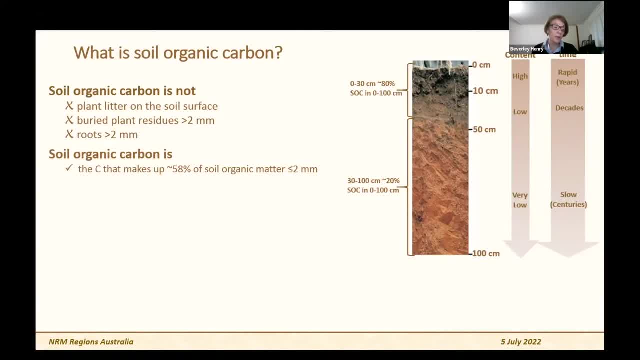 that are partly decomposed- root exudates and material like that and dead material, that sorry dead microbes and soil fauna that are also decomposing, that are fed on these materials. If we want to reliably measure the change in soil carbon, we also have to measure soil bulk density. 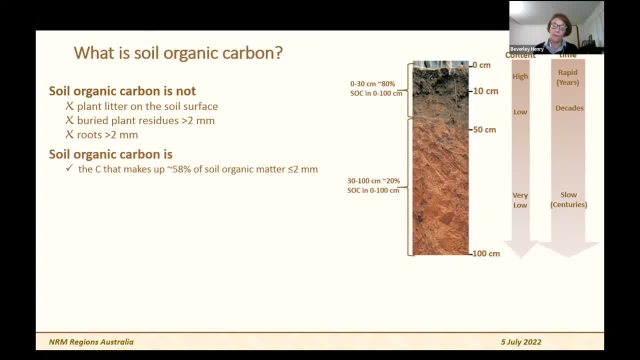 and that enables us to compare like with like. So if you're looking at a change over time, you have to compare the amount of soil carbon in the equivalent soil mass, And this is a little technicality and Luke will probably touch on that later in with. 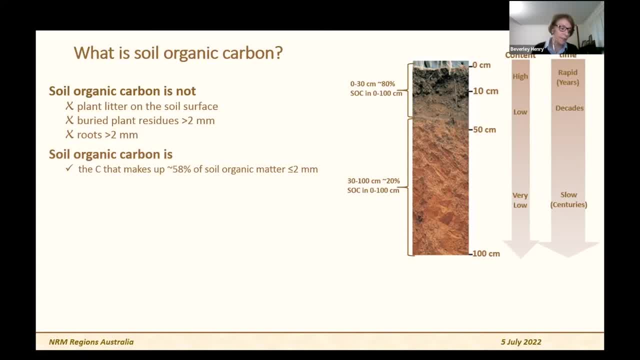 relation to accounting for the under the emissions reduction fund. So within the soil, organic matter is subject to physical and chemical transfer formations and from that you get a continuum of forms that make up about one to five percent of Australian soil amount, and these, this material, cycles at different rates depending on the stage of 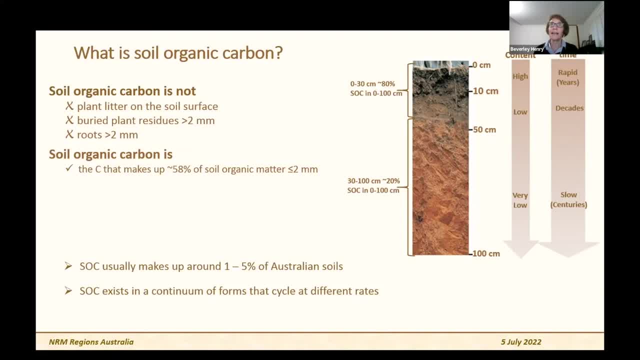 decomposure that it's at. and if you look down the soil profile, most of the soil carbon is held in the top layers, in the top 10 centimeters or up to 30 centimeters, and this is largely particulate carbon. that's fairly recently added and a little broken down as you go deeper in the 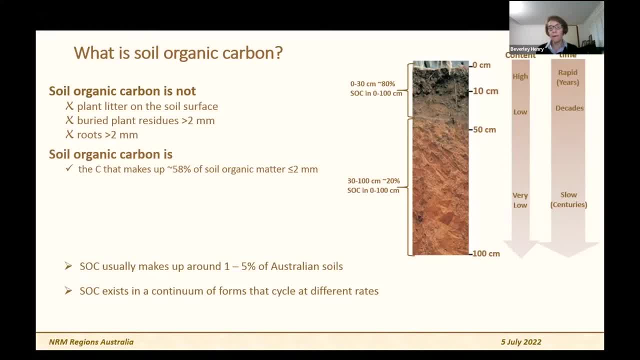 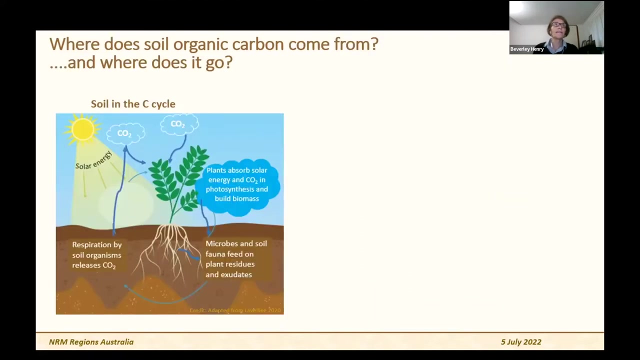 profile. the material becomes more decomposed, smaller and generally more stable. So sequestration of soil carbon sequestration requires the accumulation of the long-term storage fractions of soil organic carbon and it's important to understand that. So if we look at the the carbon cycle and how it gets into the soil, to start with, 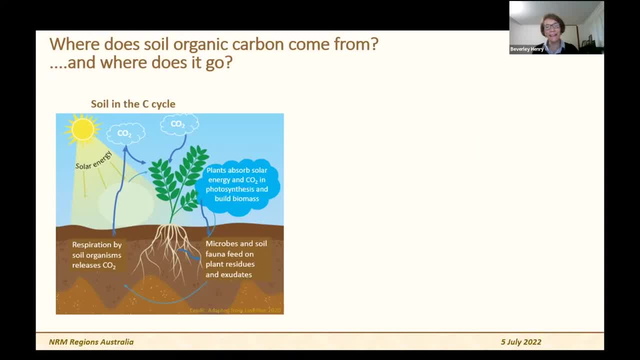 and- and I do appreciate this is fairly basic, but you know it's important to understand this- that soil carbon comes from the atmosphere, so plants take up carbon dioxide in the process of photosynthesis and, with the help of all of solar energy, they transform this into plant biomass. 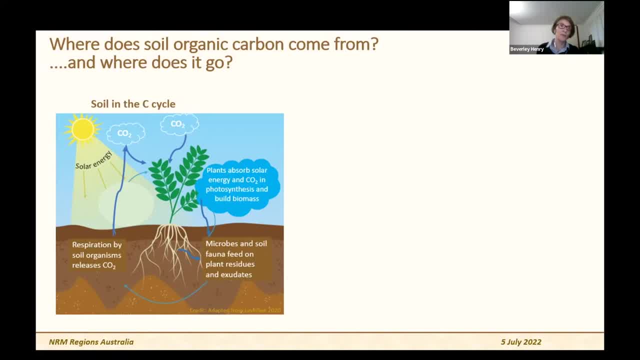 and if this helps to and it breaks down, helps the soil to decompose and it's important to understand that plant to function and to grow becomes part of plant growth. it enters the soil through decomposing leaves and roots and and also exudates and as the microbes feed on it and it breaks down. 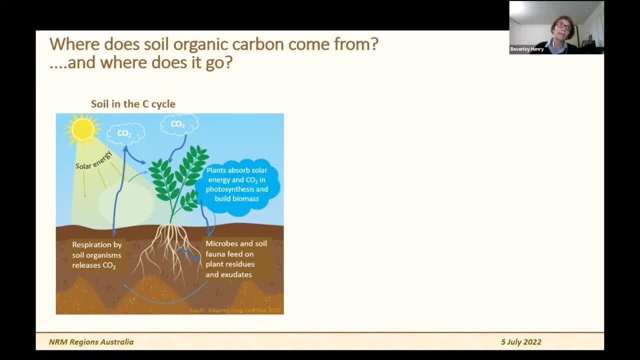 respiration returns this, the carbon, to the atmosphere as carbon dioxide, and up to about 80 to 90 percent of the carbon that's taken up in, that's added to the soil through photosynthesis, is returned in quite a short time, in a, you know, a matter of months or a decade or two. 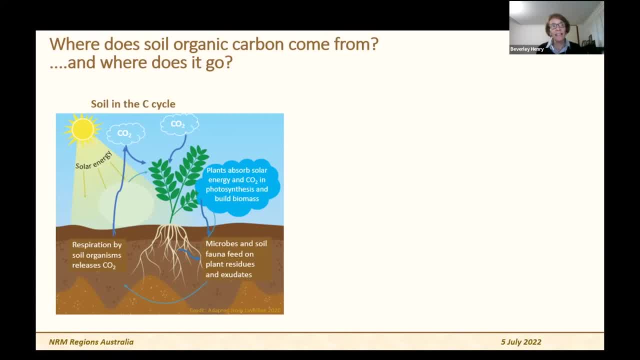 This is a very important cycle. it releases nutrients for plant growth and without that we wouldn't be able to have the plant biomass in the first place. so nitrogen, phosphorus and soil and sulfur- nutrients like that- are released in this process. but up to 10 or so of the carbon is not released in this short cycle but is transformed and becomes. 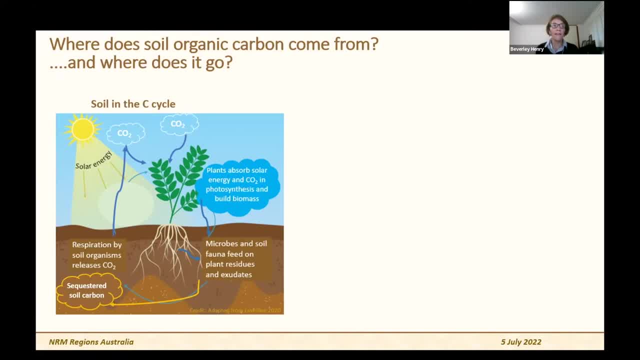 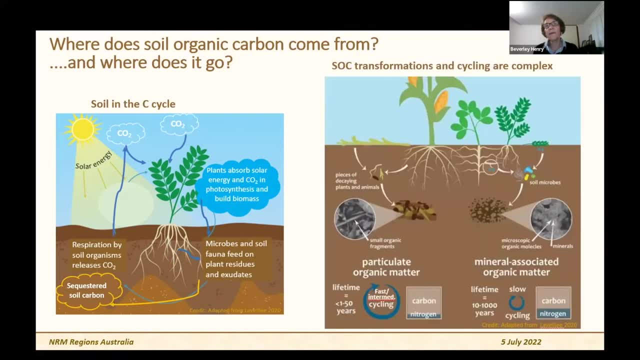 protected in the soil in mineral aggregates, and that's the component that stays in the soil for a long time- is called sequestered soil carbon, and if we separate out these two in a diagram just for ease of looking at it, the particulate organic matter is the part that um is nearly. 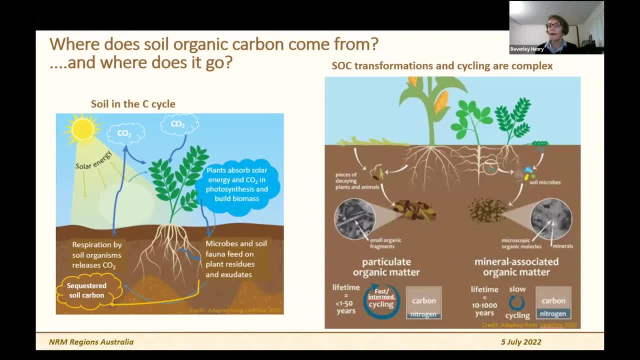 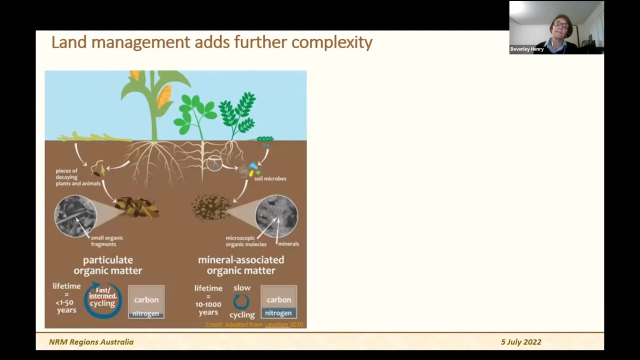 the soil surface generally and cycles fairly quickly. and the mineral associated organic matter that exists as sort of films around mineral particles protected from breakdown by microbes and stay in the soil for a longer time, and that's the soil carbon that's kept out of the atmosphere and is called sequestered soil carbon. That cycle in a natural system ends up being pretty. 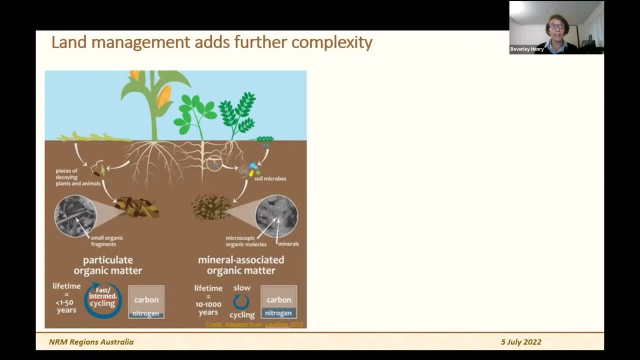 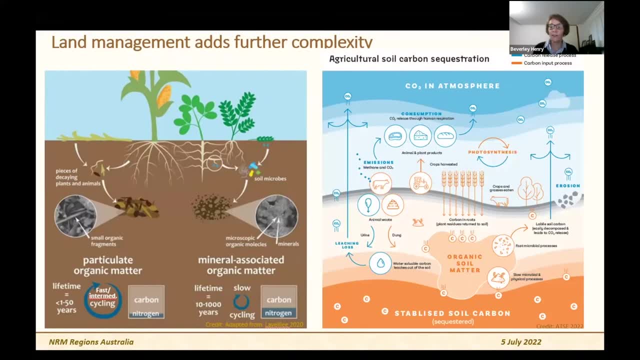 much in a steady state. so there's a little little change over time and it's a little bit more time in the amount of stored soil carbon. but once you introduce agricultural management it adds a whole lot of complexity to this relatively simple cycle. so agricultural practices change the inputs. 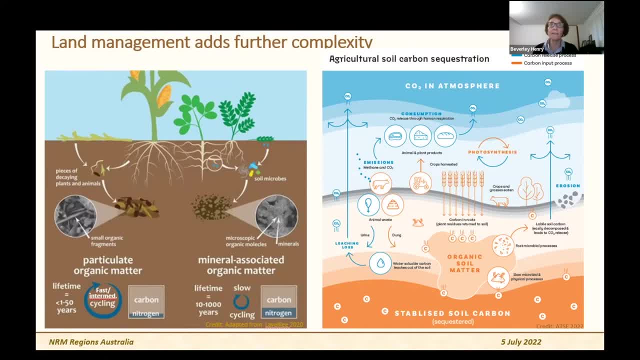 to the soil if there might be organic amendments added. there's material removed through harvesting crops and through livestock consumption. there's the soil properties are changed by adding lime to change the pH by um, by cultivation, by irrigation, for instance, and that changes the activity and the diversity of soil microbes and also influences the cycling process and both the the slow cycling. 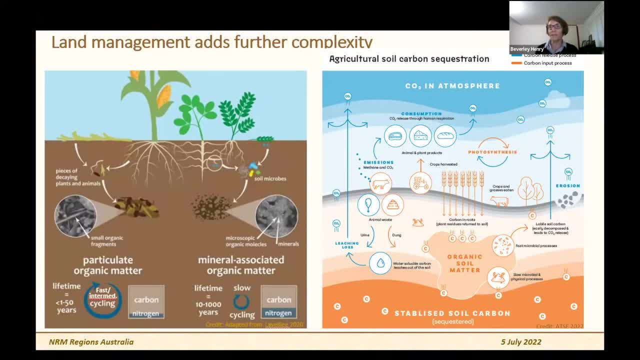 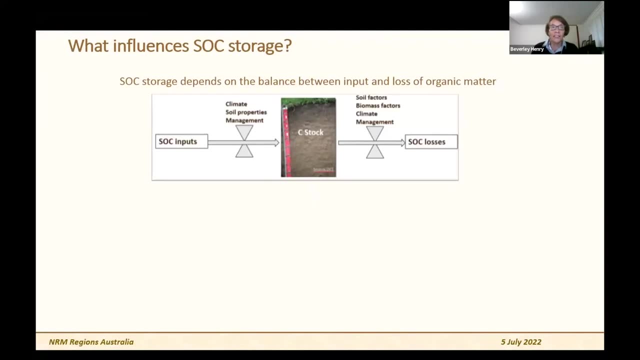 material and the stored cycle and the stored carbon material are important, but they're important in slightly different ways. We need to understand how management effects them. Just to look at this in a rather simple way: the amount of soil organic carbon that is stored depends on the balance between the inputs and the loss of organic matter, and there are a number of 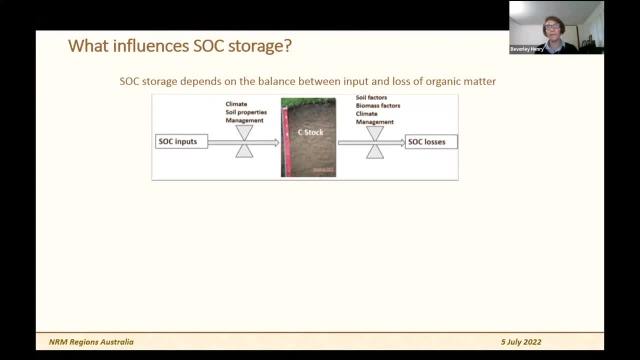 factors that affect the rates of input and the rates of losses, and to change the storage. what we want to do- if we want to change the storage- we need to stop collating the soil with some material and and turn that into a supply chain- want to increase it- is to shift the balance in these processes more towards the inputs and less. 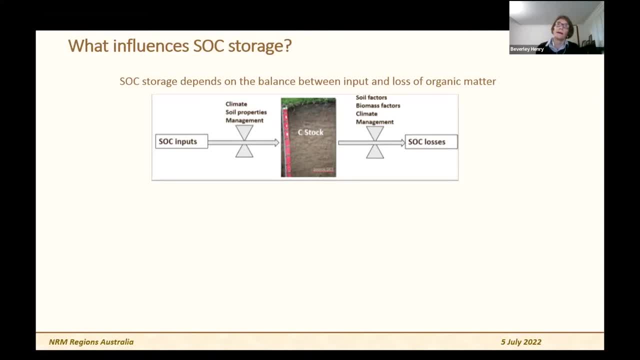 towards the losses, and we've already said that. you know there are a number of factors that affect it and that management affects it. but a number of analyses show that the most important influences, the biggest drivers on the amount of carbon stored are climate and soil properties. so 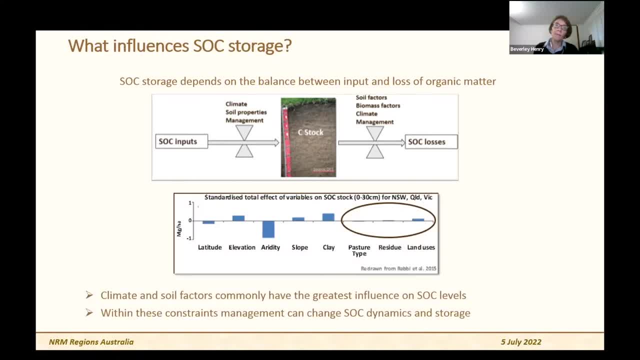 if you look at this graph it's a little bit complex but this is a meta-analysis. I looked at all the studies that have been done that looked at soil organic carbon stocks in soils in New South Wales, Queensland, Victoria. these are agricultural soils and the variables that 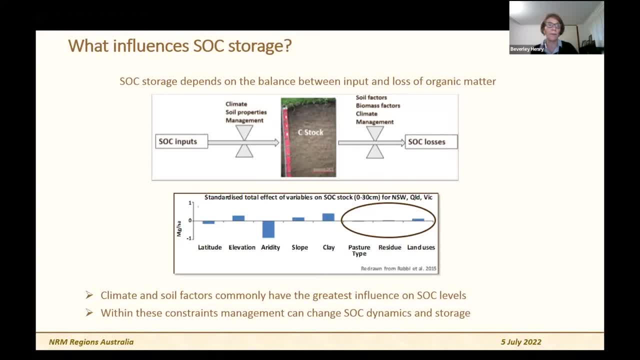 influenced how much soil organic carbon there was, and you can see that the biggest blue bars are aridity and clay. so aridity is. you can see that the biggest blue bars are aridity and clay, so aridity is. largely depends on rainfall- the amount of moisture that's available in the soil for plant. 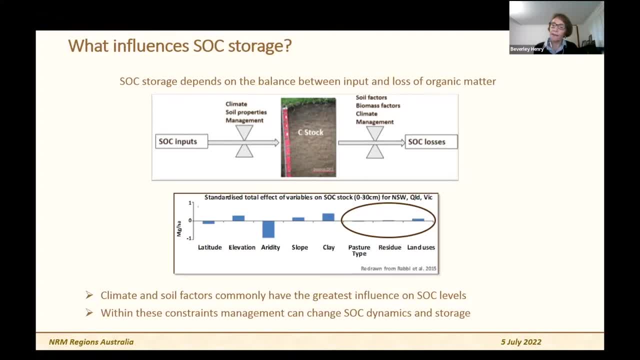 growth, and clay is a soil property that largely determines the amount of mineral associated organic carbon. so they're the principal drivers of how much soil organic carbon is stored in these soils, and on the right side I'll put a brown circle around them. there are three variables. that do influence soil organic carbon and they're the main drivers of how much soil organic carbon stored in these soils, and on the right side I'll put a brown circle around them. there are three variables that do influence soil organic carbon and they're the main drivers of how much soil organic carbon. 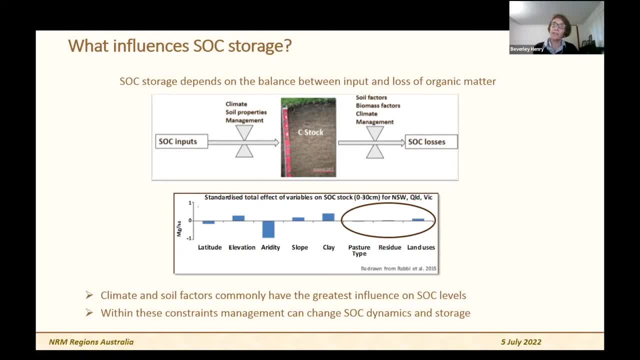 stocks that are subject to management: pasture type, residue, residual returns and land uses. these have a smaller effect, but, within the constraints of climate and soil organic carbon at any location, these management factors do influence how much soil organic carbon is stored and it's important to know that we are able to to change the environment. 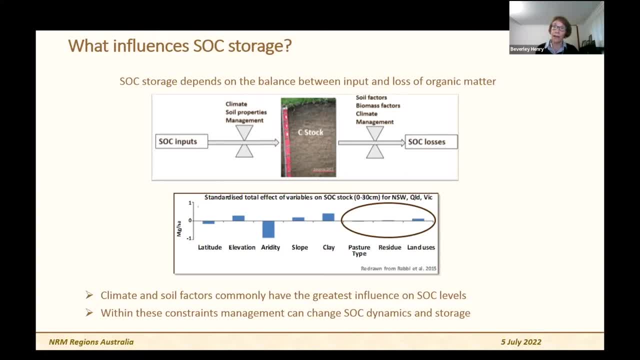 to change the amount of soil organic carbon, and it can be a positive change or it can be a negative change, and so we have to try to understand how this influence occurs, to know how much change we can make to influence both productivity of the soils, the health of the soils and its potential to 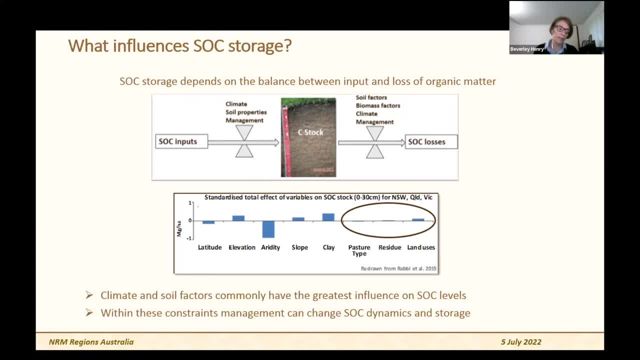 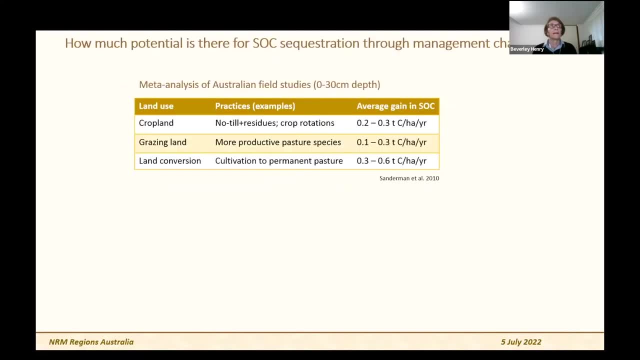 add climate change. to add to climate change mitigation benefits, we we have to sort of think about how much we can change. what is the potential for soil organic carbon sequestration? there's a lot of a lot of interest in this question from the last slide and the influence it causes. 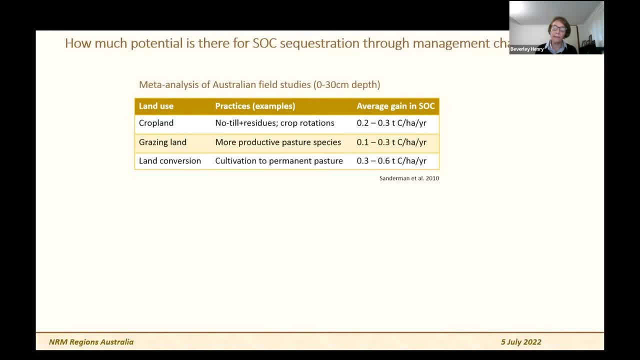 in terms of how much climate and soil properties have it becomes clear that there are regional differences in how much soil organic carbon can be changed, and we have to bear this in mind, so not to extrapolate from one side to another too freely, because it's probably not going to work. 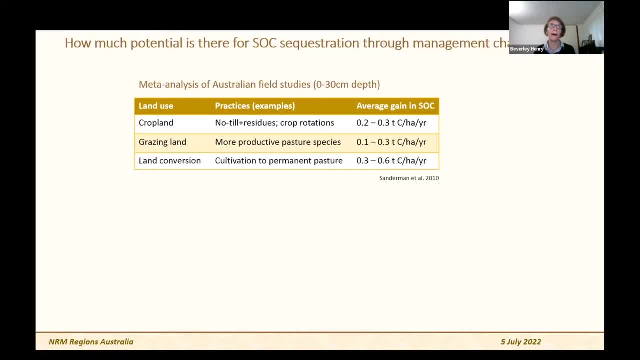 this table here shows us the summary data from a meta-analysis of australian field studies. then we've got some recalling from the last slide focussing on example models. after that we've got data showing that other types of plants that are used, so soil organic. 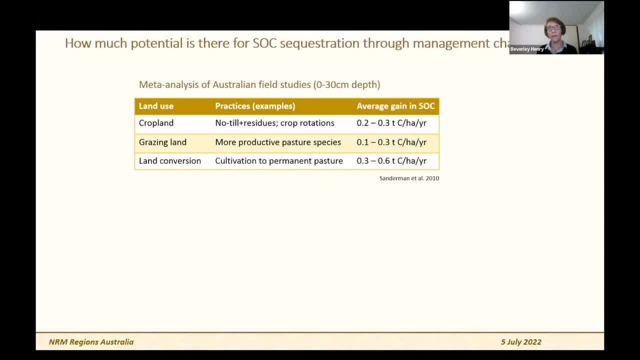 carbon, new ideas that are used to capture soil. organic carbon increased. the 14 state science provincial�� that we've breathed into quite a bit here and the effort in the science provincial science common안 farmenin is acting on these studies and so in some studies provides that you're getting cell health awareness. we're getting 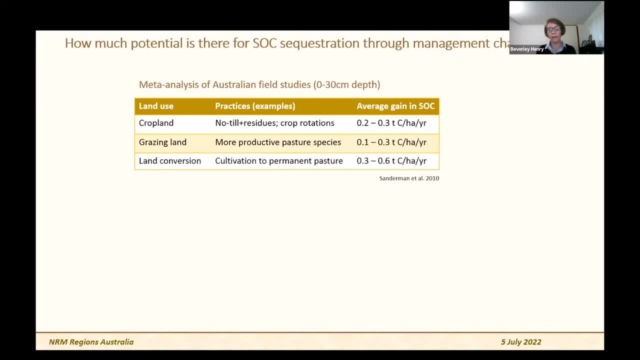 fairly critical changes. we're raising the target health central industrial Dobu田. To know moreamm. we need to add soil organic carbon, a number that would increase disturbance of the soil, so the amount to which soil organic carbon is exposed to microbial breakdown, and it increases the continuity of input generally. so there is scope to. 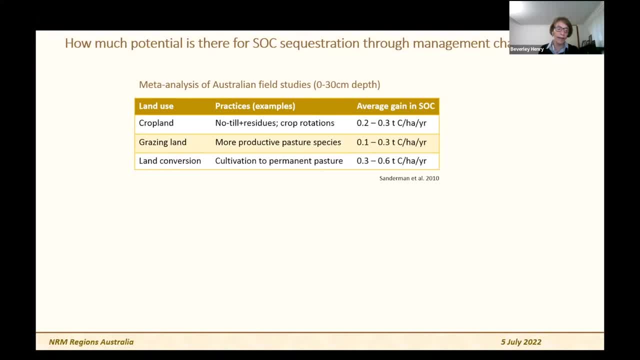 manage the, the amount of soil organic carbon that is there, the, the. the amounts are small and um, but they do cover large areas, so there is a lot of potential, but one caution that that we need to bear in mind is that while we can get bigger rates of soil carbon sequestration than are shown in this table, but often they aren't um. 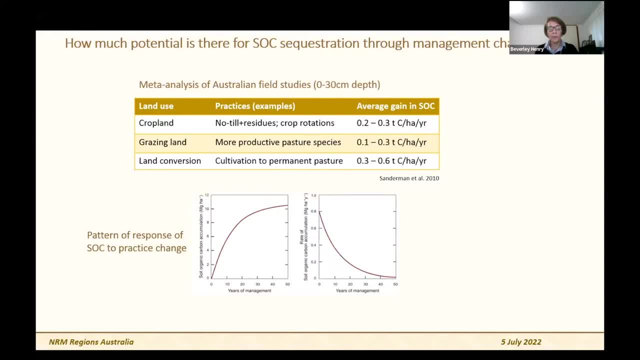 they aren't sustained. so if you have a soil that is fairly low in soil organic carbon and introduce a positive practice, you can get a fairly rapid increase in soil organic carbon. it's making up for the you know what has been lost before. so in the first five or ten years after introducing a new practice, 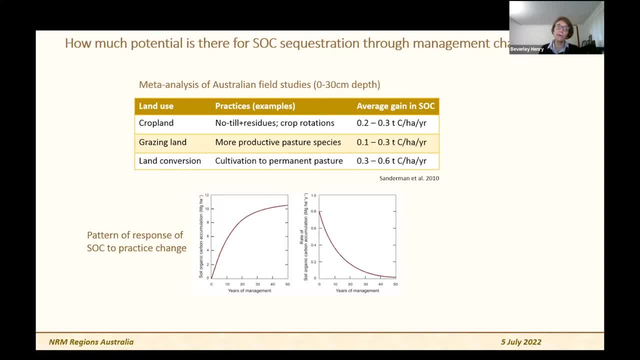 there can be a rapid increase in soil organic carbon, but it's incorrect to assume that that rate will continue indefinitely. what happens is that, as the capacity to store carbon, um, is taken up, you approach a new steady state that's determined by soil organic carbon and climate in the area that you're in, and the rate will slow down. the rate. 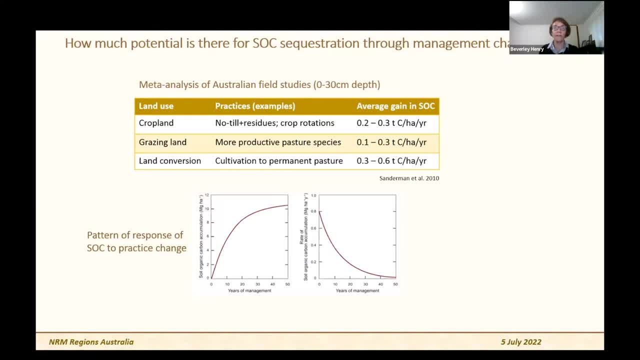 of sequestration will decrease, as you can see in the right hand side of those two stylized curves there. so that's one caution. there's another caution that I would I'd emphasize too, and that is that Australia has a very variable climate. we have droughts, 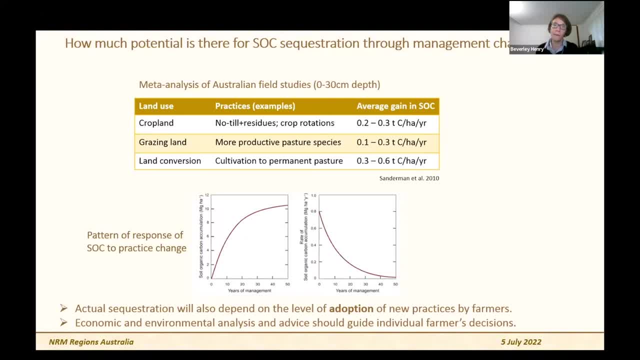 and obviously we have floods, as some people are experiencing at the moment, And the rate of inputs varies with the quality of the season, if you like. One study in New South Wales that was led by Warwick Badger, who showed that 12 years of gains of soil carbon following the introduction of an improved management 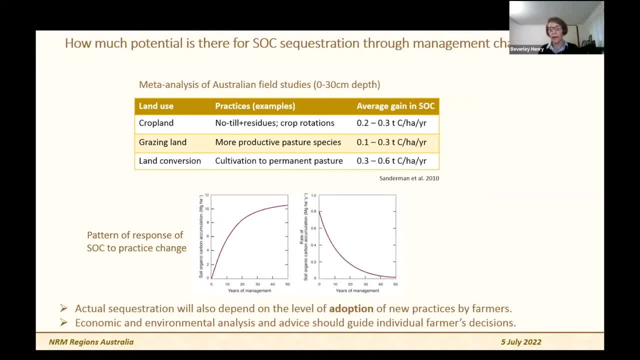 could be lost in three years of drought. So the gains occur sometimes pretty slowly, but that soil carbon can be lost again. The other caution I would say is that it's not a good idea to assume that sequestration that's occurring due to a management change. 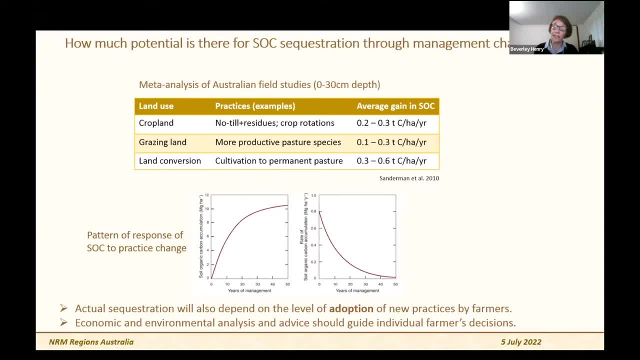 can be multiplied up by the area that is potentially available for that change. It depends on the adoption by farmers, and changing practice is a big decision in farming and it's best done with good information and a lot of homework. I suppose behind it because there are economic and environmental impacts from changing practice. 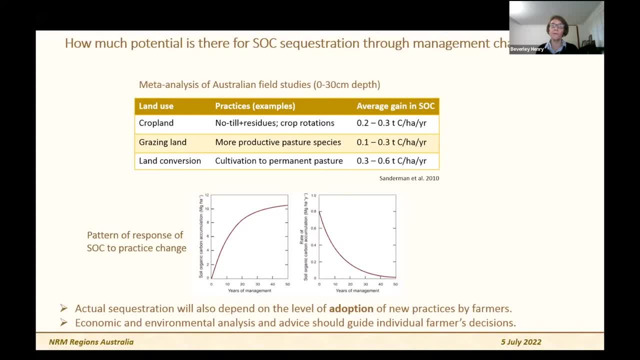 So that it's important for farmers to be informed and it's important for policy not to be a burden on the environment. So that's why it's important for farmers to be informed and it's important for policy not to be a burden on the environment. 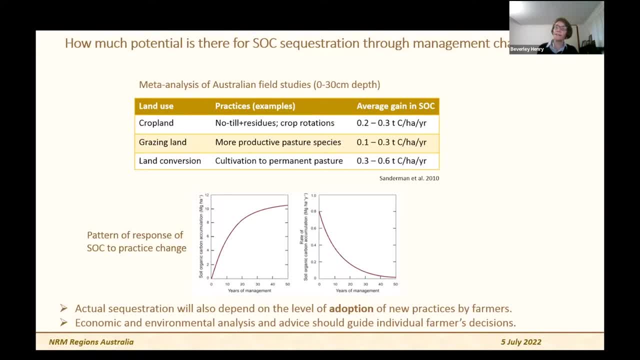 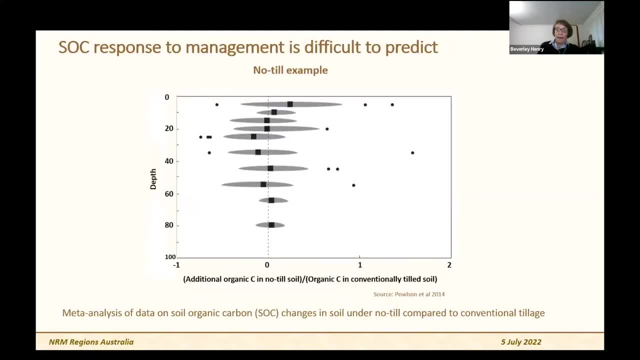 to assume a certain level of adoption, that that can occur. an important decision. So the last point I'd like to make is that in looking at the that, what is achievable under soil organic carbon management, we have to be aware that the knowledge is growing. we don't have all the answers Initially, when we were looking, when our 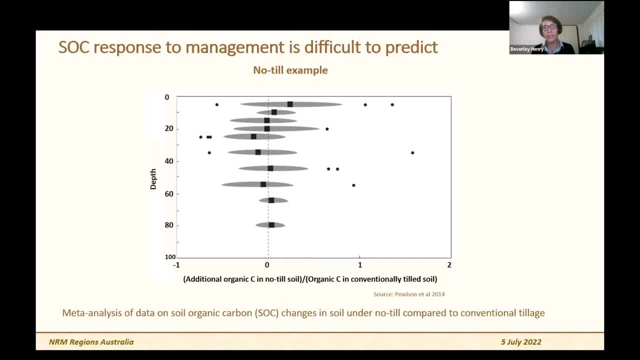 scientists started looking at soil organic carbon. changing all tillage to a no-till system was a good way to sequester more carbon for climate change mitigation benefits, And it became clear that no tillage didn't actually always lead to soil carbon sequestration. 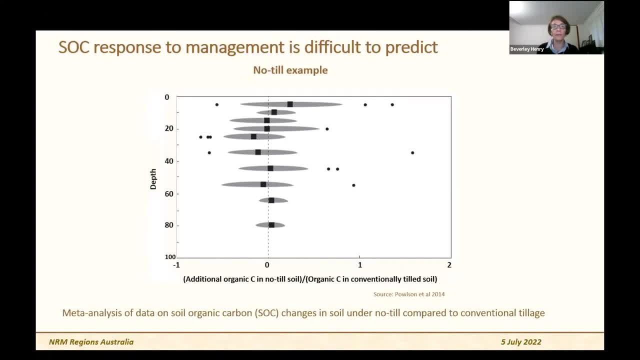 This figure shows the additional carbon under a no-till soil soil situation compared to a conventionally tilled soil and the zero line that you can see dotted there is a no change. So near the surface layers there is more carbon under no till. this is because of the 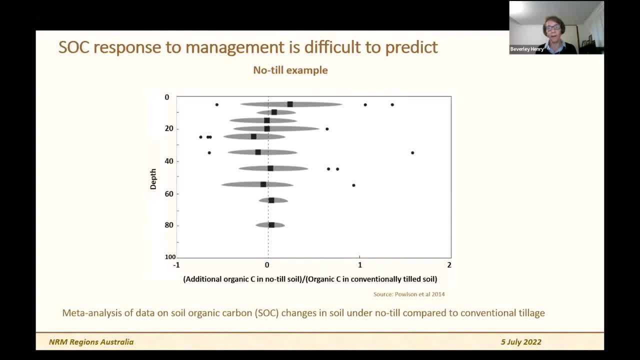 greater inputs and it's largely particulate and rapidly cycling carbon. If you go down to a depth of 20 or 30 centimetres, there's more carbon under the conventionally tilled soil and this indicates a redistribution that occurs when, when you till, versus 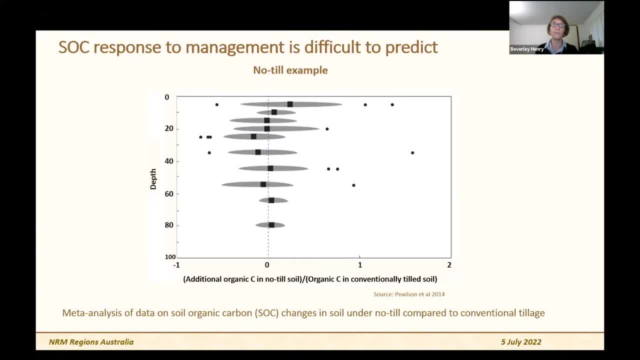 no till. So 20 or 30 centimetres is below the plough depth generally, and that redistribution and the fact that there's very little change of the even great depth means that overall there is often no or very little change in stored soil carbon in these systems. So there's two take-home messages from this. 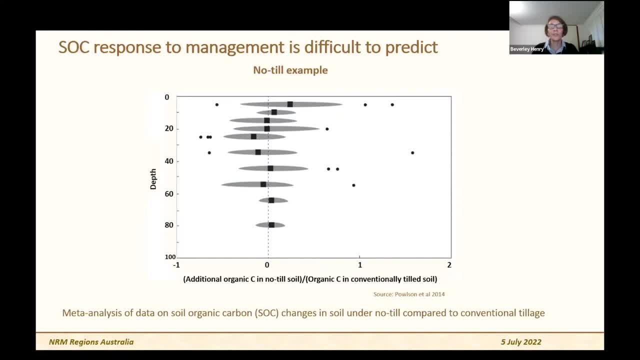 One is that the soil carbon that's increased near the surface soils is very beneficial for productivity and for soil structure and condition generally, but that it doesn't necessarily equate the soil organic carbon storage for climate change benefits. and the corollary to that is that 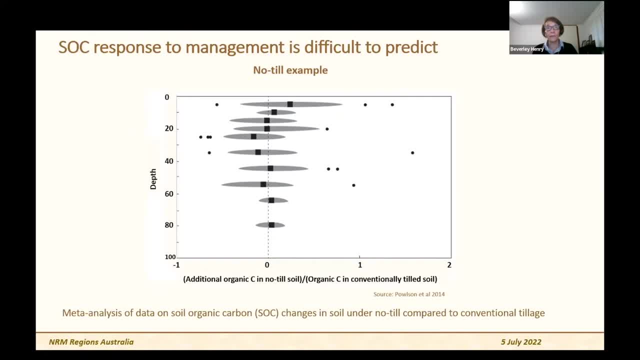 measurement for soil organic carbon sequestration. the long-term storage has to take into account a greater depth than the top surface layers. What so again in the top 10 centimetres does not necessarily translate to increased storage over a longer time. So I've rushed through that a little bit because there wasn't much time and I've 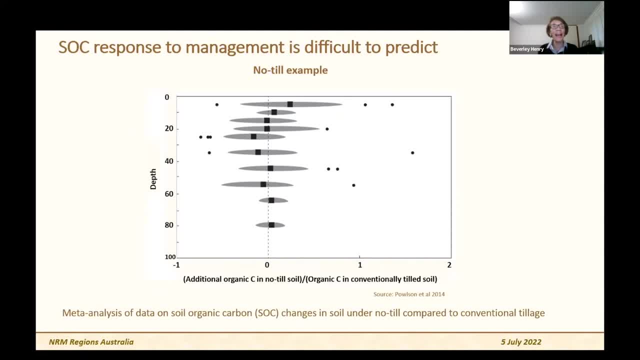 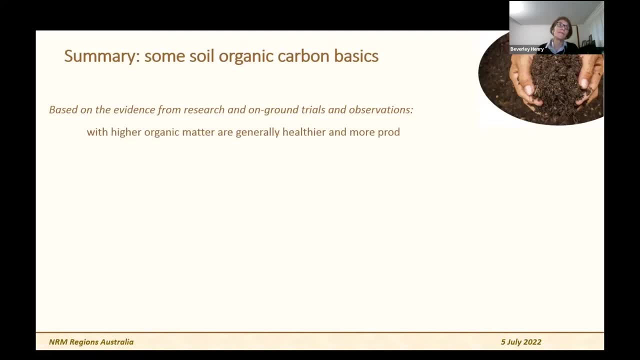 tried to fit in a lot. I hope that it hasn't been too confusing and I'd just like to wind up with some summary points. Firstly, soils with higher organic matter are generally healthier and more productive. Soil organic carbon transformation dynamics are complex and soils can be a net sink or a net. 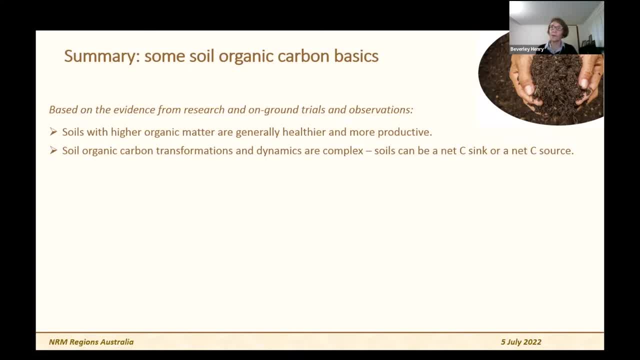 source, depending on how management is, but also depending on natural fact natural climate factors. Managing agricultural soils to improve soil organic matter content and dynamics provides many benefits. Rapidly turning over soil organic pools release nutrients for plant growth and improve soil structure and condition. Slower turnover soil organic carbon pools may also contribute to climate change mitigation. 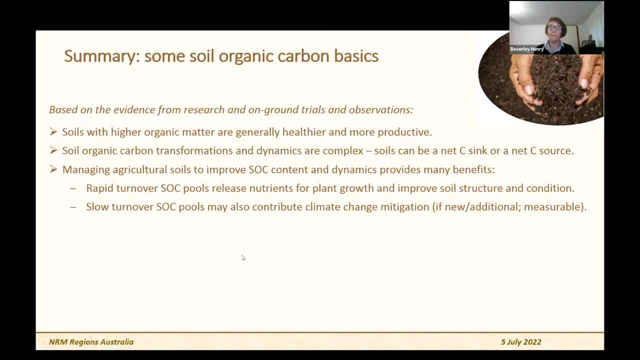 but there are a number of factors around counting that as soil carbon offsets, which you'll hear more about in later slides. So again, there's been interest in soil organic carbon transformation. later talks: the practices that store soil organic carbon often have co-benefits for. 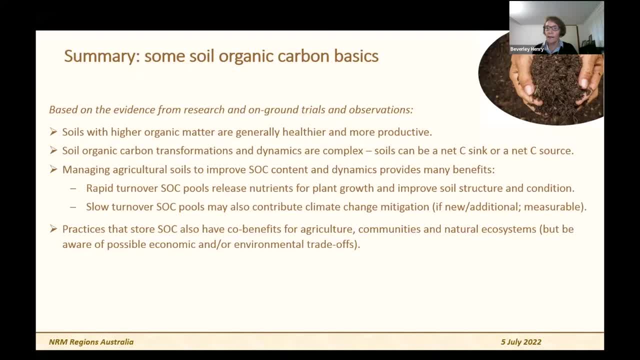 agricultural communities and natural ecosystems in terms of soil structure, water quality, a whole lot of ecosystem services. but it's important to be aware that there can be possible economic or environmental trade-offs when you change management for soil organic carbon. so adding irrigation may have implications for water costs, for instance, and and water availability for other. 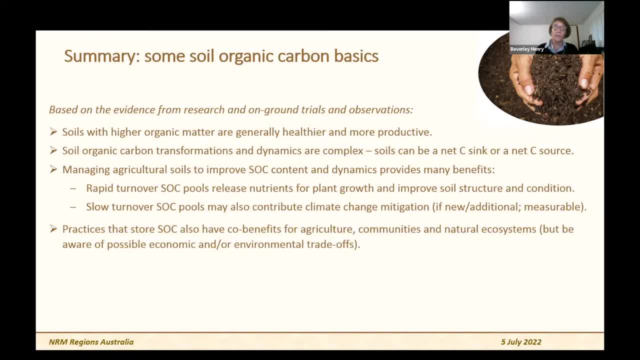 purposes, and it can also affect the the business side of of farming as well. so within climate and soil constraints, good management can increase carbon in soils, but maintaining that soil organic carbon is more difficult. it can be lost again and neither the soil organic carbon nor the science of soil organic 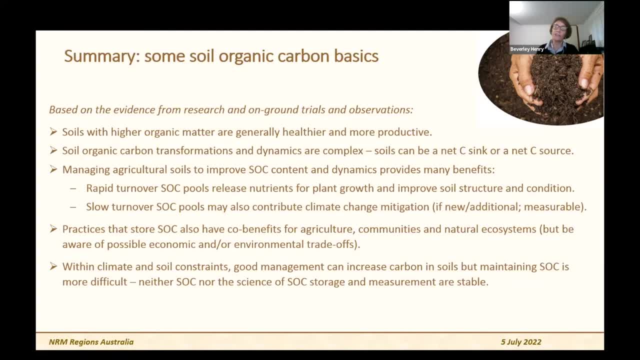 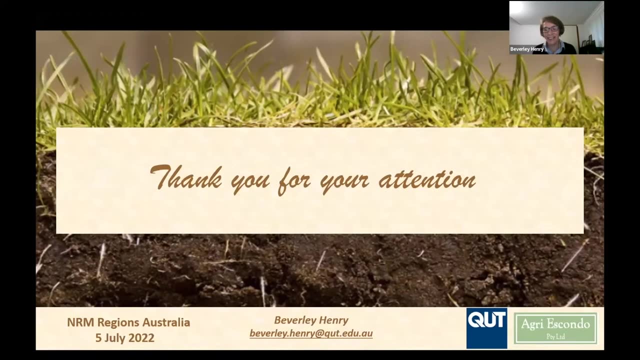 carbon storage and measurement are stable. we need to stay on top of the growing knowledge, and that's only been that can will continue to develop. so with that, i would like to thank you for your time and i'll see you next time. thank you for your attention and hand back to Rachel, thank you. 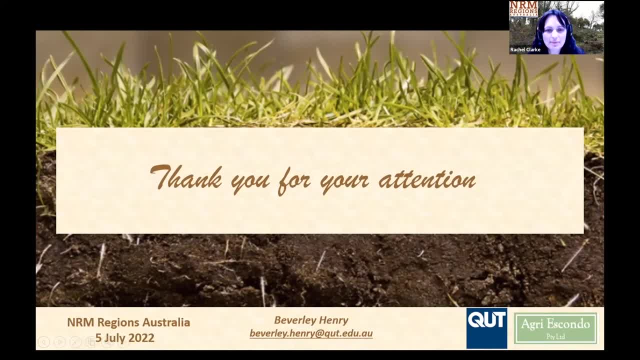 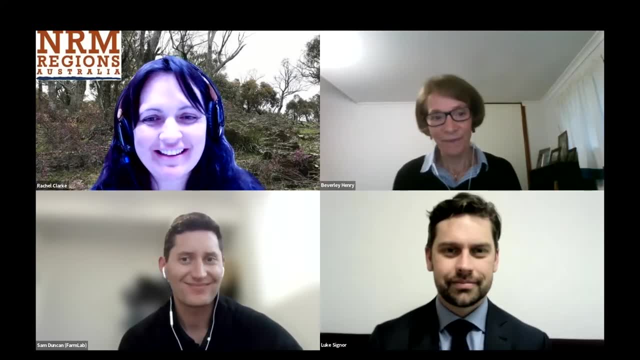 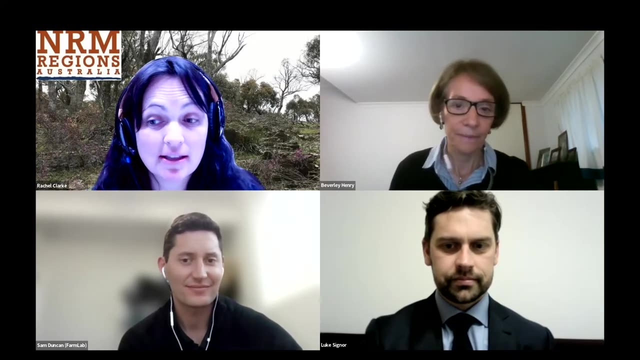 thank you so much, Beverly. that was um really interesting and i'm really looking forward to picking some of those um muddier issues during the Q&A panel session after everybody's spoken. so thank you so much for um your introductory talk there. um also thank the the first brave. 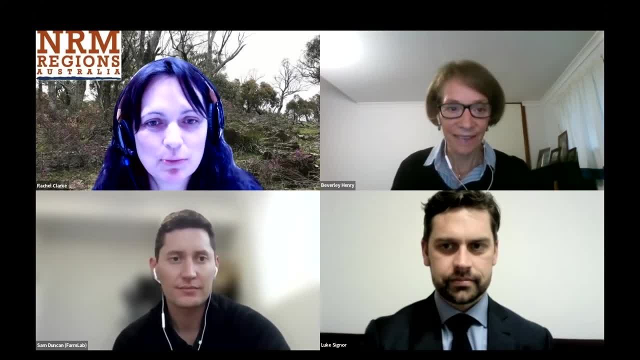 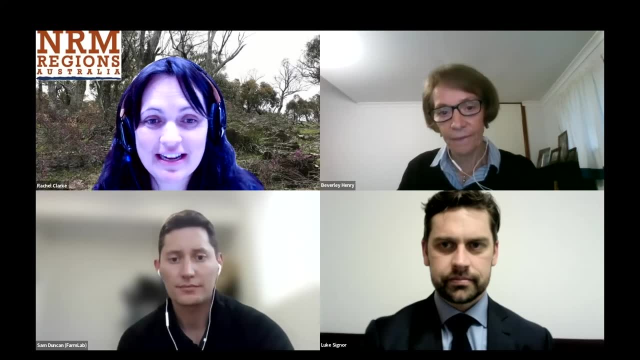 person that's put a question into the Q&A. so this is just a reminder: to put your questions into the Q&A. um, and we'll get to them when everybody, all our questions are answered and our speakers have had their opportunity to speak, so um. thanks so much, Beverly, and um we're. 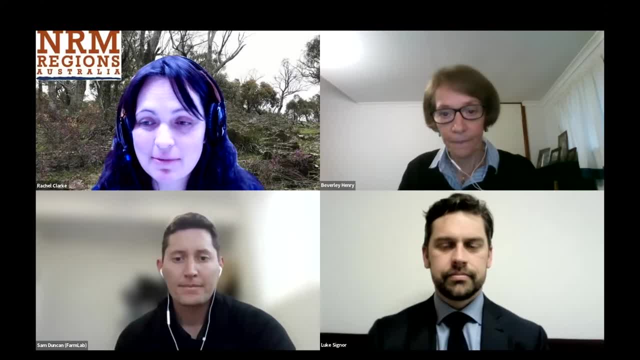 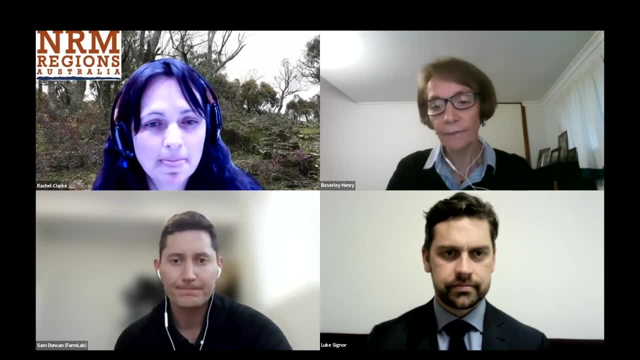 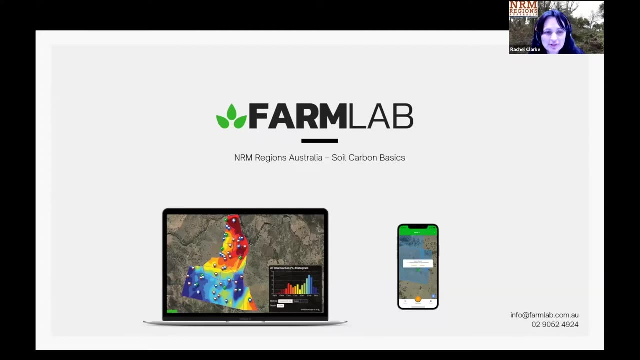 going to move on to our next speaker, Sam Duncan. Sam, if you'd like to get ready to share your screen. so Sam Duncan is the Chief Executive Officer of FarmLab, and i first saw Sam speak at a future farming conference that was broadcast from South Australia last year. Sam was the first person that 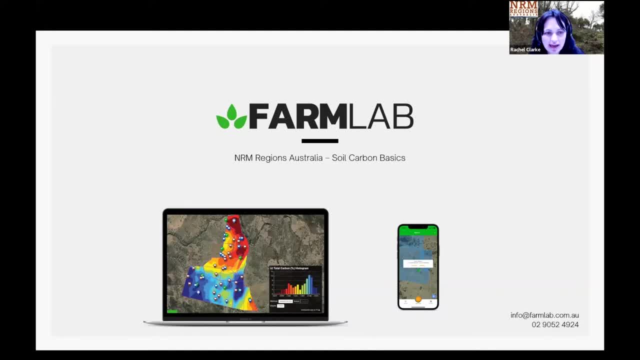 addressed some of the really key questions i had about how and where soil organic carbon could be stored. so i was really- i'm really delighted to be able to get Sam to talk about that and i'm really excited to come along today. Sam's a passionate advocate for sustainable agriculture, a lover of. 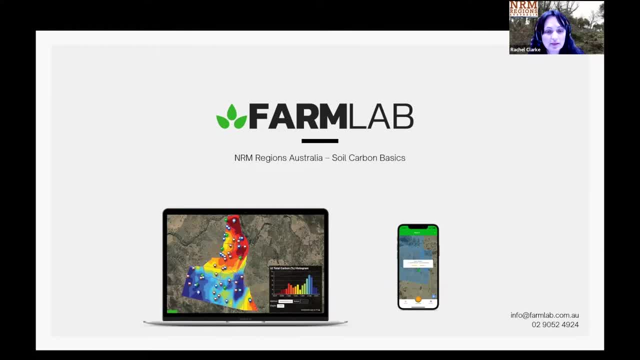 the outdoors and an air force veteran of 12 years, he founded FarmLab in 2016 with the hypothesis that if farmers had better soil data, they could better manage soil carbon. since then, FarmLab has evolved into a sustainability company, helping farmers and their consultants collect and measure. 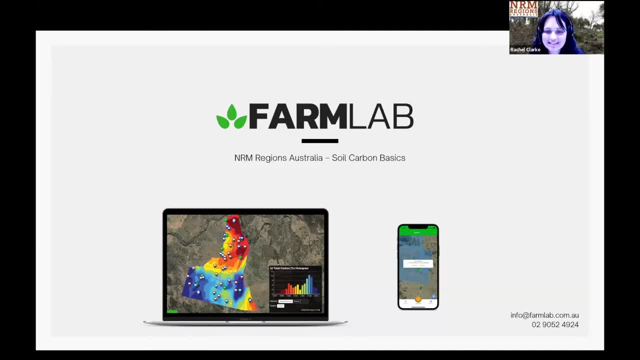 the environment using technology. welcome and thanks so much, Sam. thanks, Rachel, you can hear me, okay. yep, sounds good, fantastic. well, uh, thank you for squishing me between Beverly and Luke. so, um, i i'll be very careful about what i say today, because i've just come after the science piece. that was fantastic. 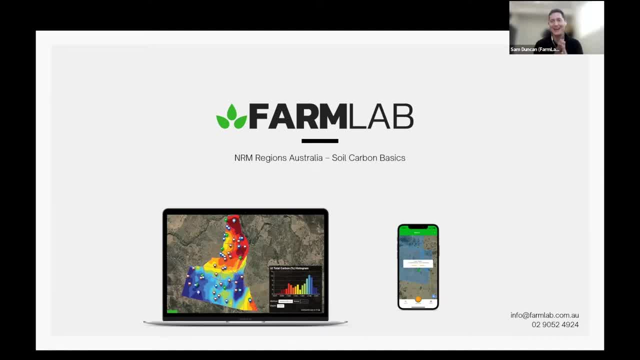 thank you, Beverly, and, uh, Luke will tackle this from the regulator piece. uh, we'll see. we'll sit in between and i'm going to try and make this as pragmatic as possible and as practical as possible for those farmers out there in the audience and those consultants out there in. 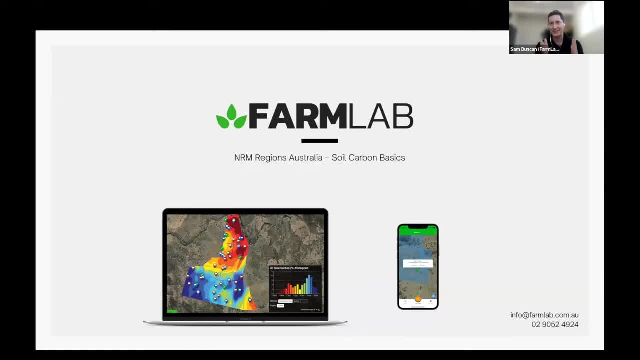 the audience, working with these farmers. so what does FarmLab firstly just say to you is that you know we're a software platform. we reduce the cost to complexity to run these projects, for a consultant um to to measure the soil to run the incredibly complex clean energy regulator. 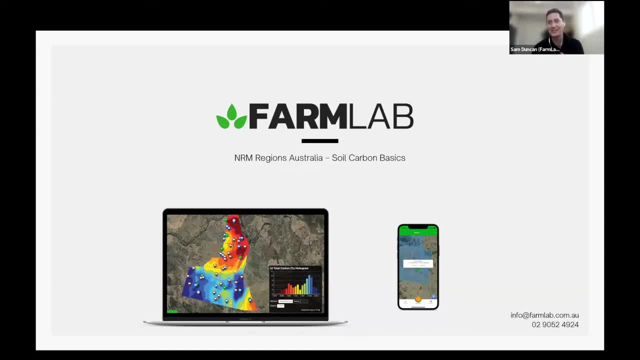 calculations. sorry, Luke. um, Luke and i are on the phone every second day at the moment trying to figure, figure, figure some some of these things out and, um, really just reduce the cost to the farmers. right now they're quite. you know, with complexity comes high cost, so we're going to try. 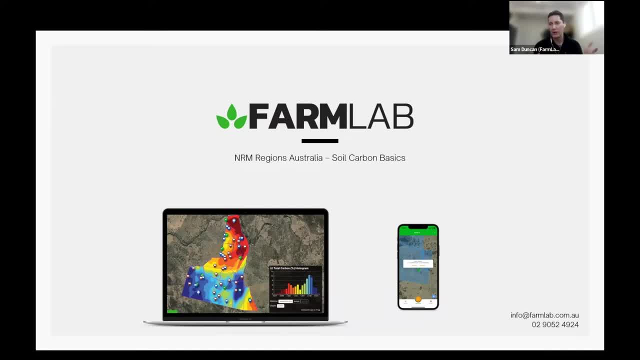 and we're all about trying to streamline that. but more broadly, we're an environmental measurement platform. we give people a mobile app to collect samples. soil samples, we're moving into plant and water samples, hit testing as well. we do biodiversity, so you can go out and collect bird calls and other. 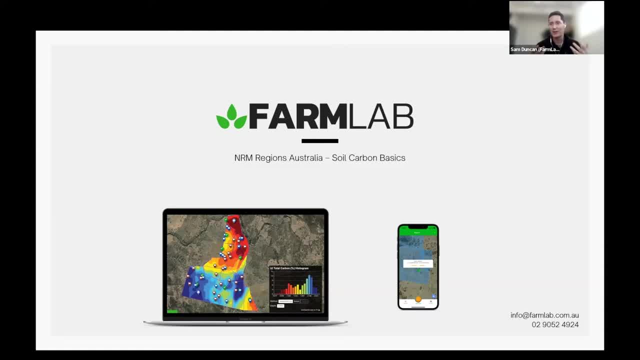 bits and pieces and then map them, and, and the key thing here is that we believe, as Rachel said, that if people have better data um and can better measure things, they can better manage things, and i think, um, you know, Beverly had a really nice little into that um, that piece there which is the 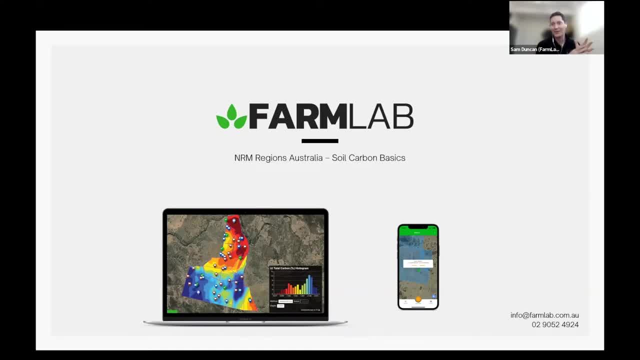 soil, organic carbon. um, the science is developing and we're understanding more and more, um, as we go about carbon and the environment more broadly. we really need the data to to sort of back that up and to help us develop some of that understanding. so, um, without further ado, i'll jump in. so what am? 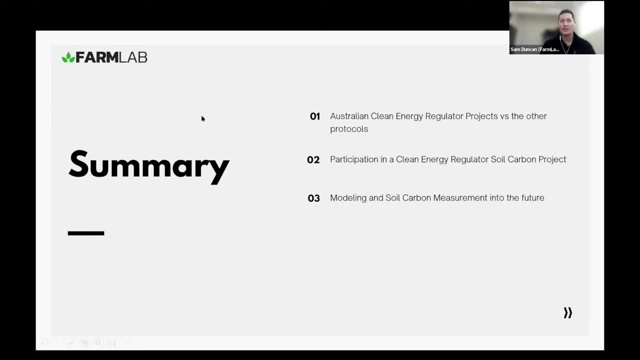 i going to cover today. um, look, i'll talk about the australian clean energy regulator methodology. um, i noticed there was a q a question there about how things are measured. i also will reference other protocols just to situate everyone as to where australia fits in the grand scheme of. 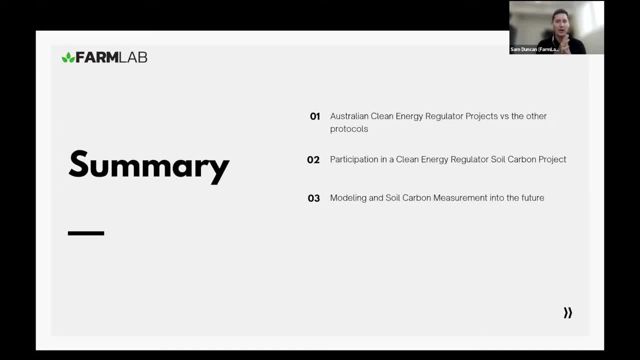 things. we'll look at some of the factors uh to consider when participating in a clean energy regulator: soil carbon project, in particular, carbon potential and what we're seeing across australia. and lastly, we're going to look at modeling and soil carbon measurement into the future of some additional sort of up-and-coming things there, um, which will also tie into so um. 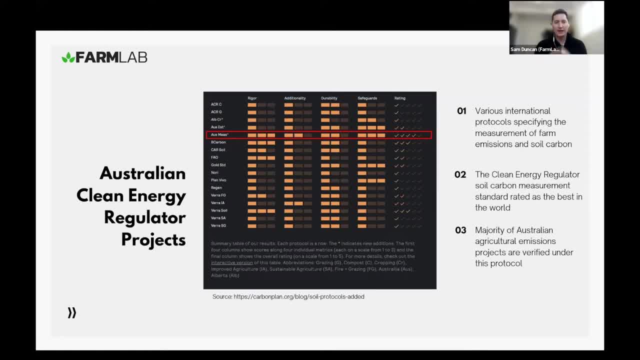 more to follow. so where do we sit as a um, as as a protocol and as a method globally? um, you know, believe it or not, and i think this is a result. i'm sure luke can provide some of the history here- but um, australia has one of the most advanced uh. 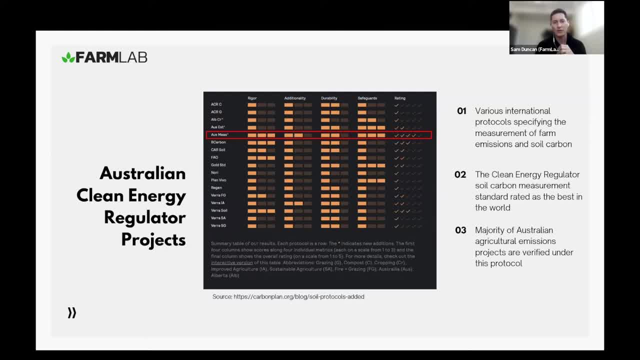 carbon regulation and regular regulations in the world. what i've got here is a little summary provided by carbonplanorg. they are a non-not-for-profit that have assessed all of the different measurement and modeling methods um available today globally. many are voluntary markets, but we are a non-profit organization that has been involved in a number of related work. 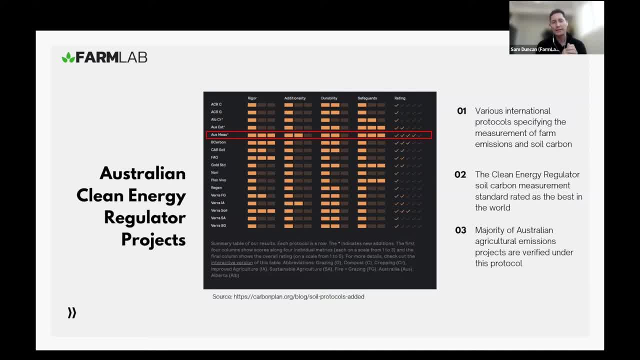 with the government, and we have been working closely with a number of other organizations that have been involved in this overall process, and also with the gold standard. um, that's uh, have developed this method that has been being used, and used to generate carbon offsets and sell carbon. 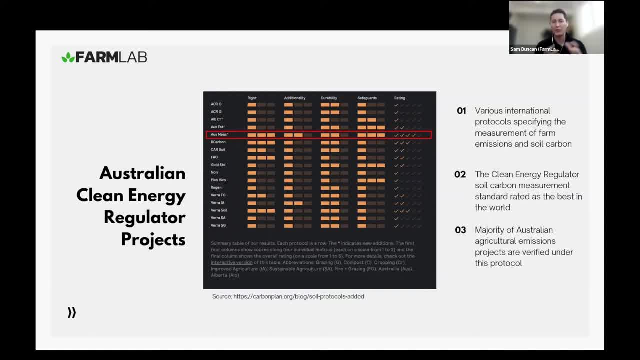 credits. australia, as you can see by the four ticks there on the right, is probably one of the highest standards in the world. but as i said before, with complexity comes cost, so it is a little bit more. I will just say that Australia has an estimated method which uses the full-cam model to estimate changes in soil carbon. 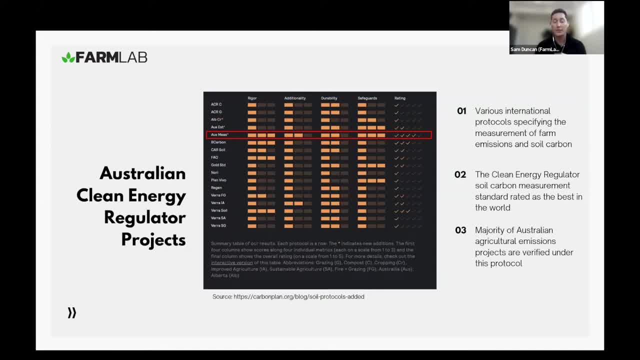 It is effective. However, it's not as effective as the measured approach, which requires actual soil sampling. I can answer any questions about the Luke's. probably better to answer about the estimated method and the full-cam models, but it is out there. 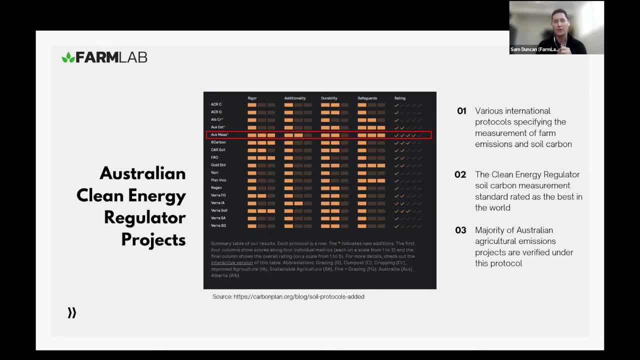 We don't see too many of our clients pick it up just because of the return on investment for the cost of entering the project versus what the client is likely to get, because it does have a habit of not underestimating but potentially underestimating how many offsets. 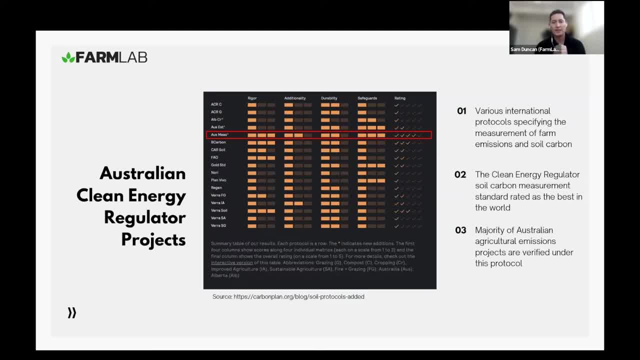 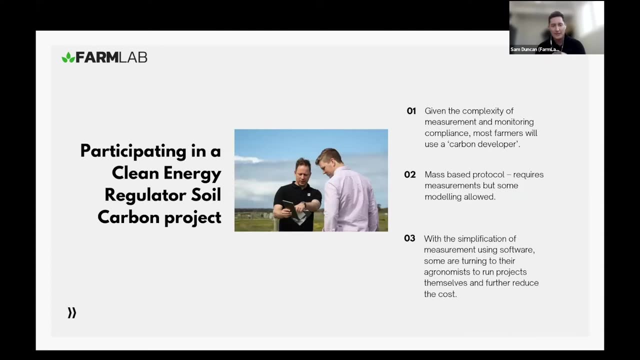 could be generated over that time period. And so, yep, majority of Australian ag emissions projects for soils are generated under the measured protocol, And I'm sure Luke has the numbers on that, And if I'm wrong, please correct me. Participating in a regulated project. 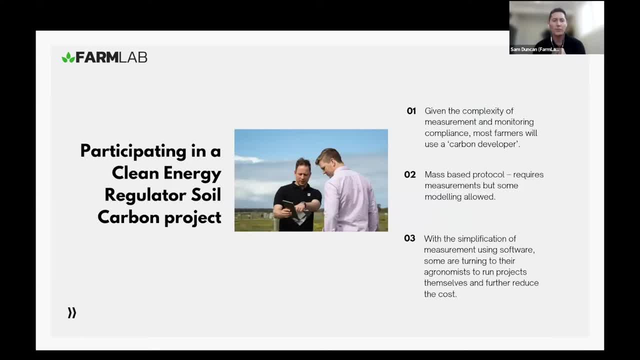 So we'll just touch briefly on what participating in a soil and a clean energy regulator soil carbon project looks like, And because Luke's going to go into this in much more detail, I had a brief look at your slides there, Luke, and I won't spend too much time on this. 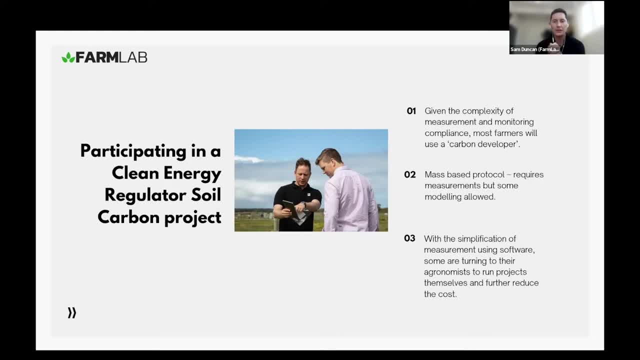 because you'll cover this more accurately than I will. But three things to talk about. given the complexity of measurement and monitoring compliance, most farmers use a carbon developer. It's why carbon developers exist today. You know they're not just there to take your money. 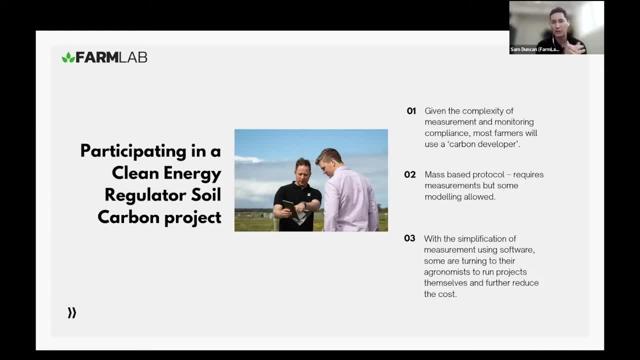 and your offsets. They are there to simplify a lot of the compliance and the monitoring issues. There are a lot of complexities when it comes to this, and the regulations do change, So having somebody that you can work with that's up to speed on the latest changes is really crucial. 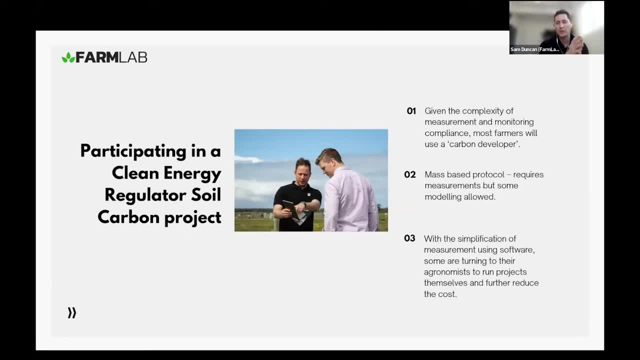 We do sometimes work with farmers direct through the Soil Carbon Services Pack, but quite often it can be more efficient to work through a carbon developer. We work with quite a few of those. Secondly, Australia has a mass-based protocol which requires the measurement of soil. 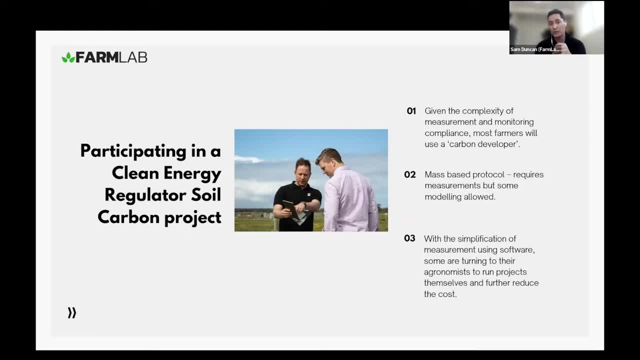 and the estimation- either the estimation or the measurement of soil, equivalent soil mass or soil mass, when those measurements are undertaken. And what does this mean? I think Beverly's touched on this in terms of how soil carbon is measured. We don't just look at the percentage. 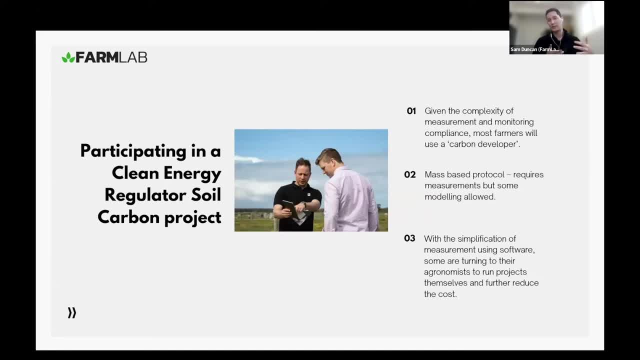 We also have to consider the content of the soil and the bulk density of the soil to calculate the amount of carbon that is measured. So we have to consider the content of the soil and the bulk density of the soil to calculate the amount of carbon. 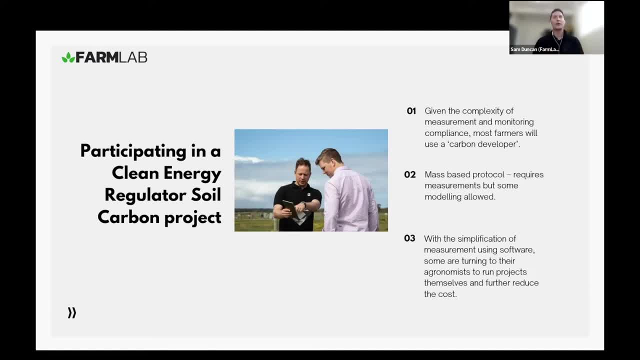 So we have to consider the content of the soil carbon being sequestered in that soil, so really important. what it means is- and i will refer to percentages later on- but, um you know, if you increase soil carbon by one percent in a soil with a high bulk density, you'll um increase more carbon and generate more carbon offsets than if. 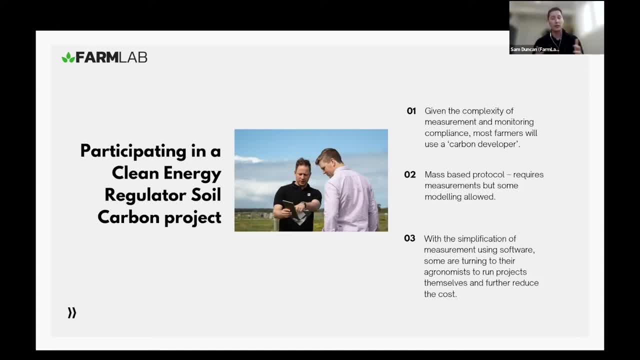 you increase carbon by one percent in a, you know, soil with less, lower bulk density, um, because there's more your potential, you're, you're increasing, um, your uh, you're increasing the mass of carbon, um, and this is what what it's about. lastly, with the simplification of measurement, 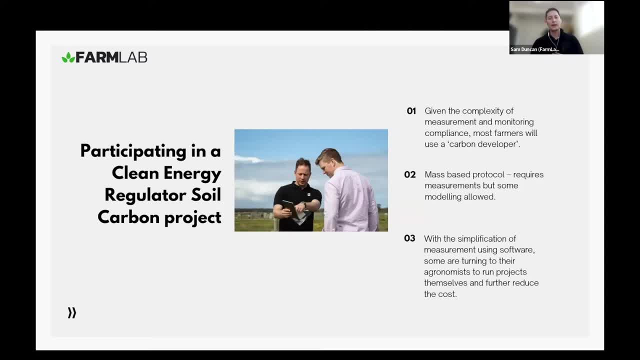 using software like farm lab. some? um of our clients are turning to their agronomists to run these projects and there's some socio-economic advantages there where a lot of the? um, a lot of farmers have really tight relationships with their agronomists and consultants. we are starting to see 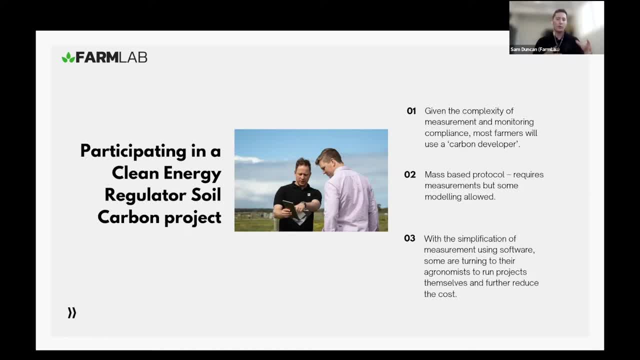 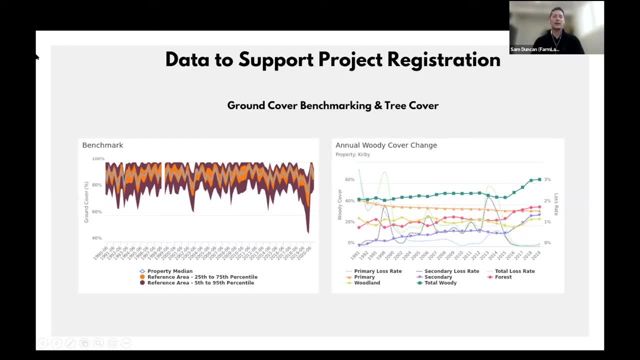 some consultants sort of take the place of the carbon developer and work with their clients to run these projects, which is which is exciting. i'm really excited about that. um. so let's just get into the first step around: um supporting registration and sort of what to look for on your own property and um, if you are considering 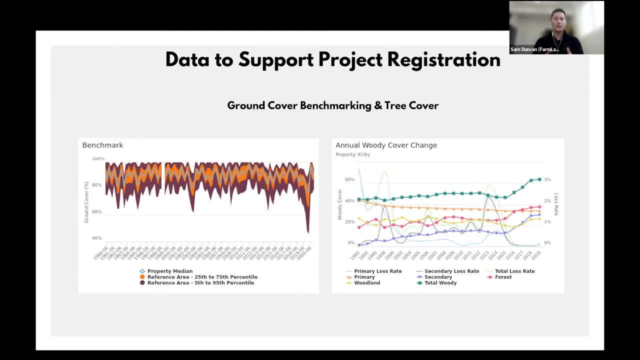 entering, entering a project. so there are a few key things. um, we provide what we call a soil carbon offset report, which is a very general report. it's very cheap, but it's a desktop. look at the farm and what we cover off on uh thing, uh, two things in particular. there's a few things on: 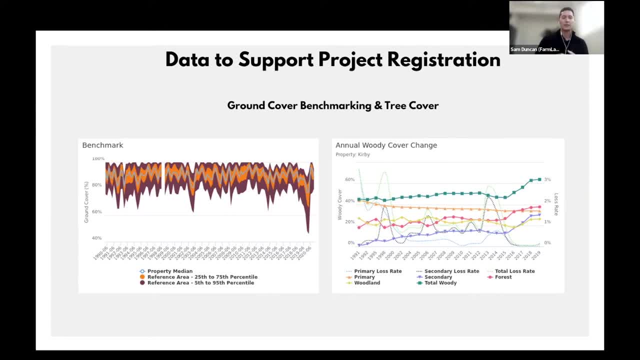 it as well. but essentially we look at ground cover change. we get this through partners um, partners at cebo labs, um, because that correlates- it does correlate well with management practices, as well as soil carbon levels now. so this is the graph on the left hand side and the farm that 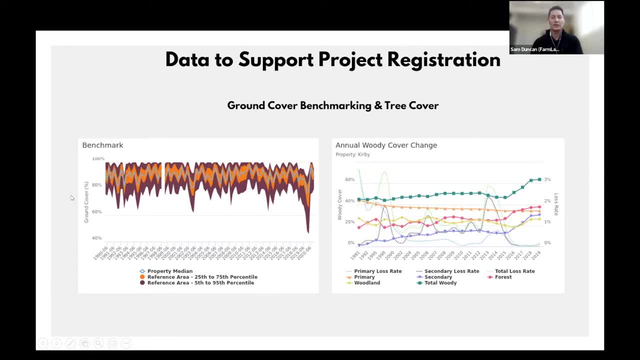 we've mapped is the blue farm, is the blue line here, and what we're seeing is the change in ground cover over time and if there's a downwards trend, which there has been particularly around sort of you know, the drought 2016 to 2019, um, you know. 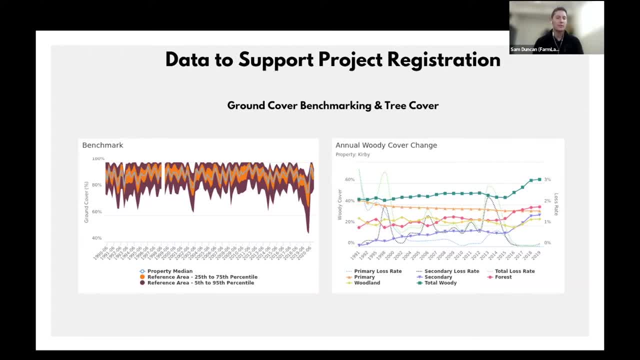 we can fairly, reasonably, accurately estimate that there's been a decline in soil carbon and so this is really important. this is sort of looking at what the man you know, helping a farmer and helping somebody on the ground- link a management practice to a change in change in soil carbon. obviously. 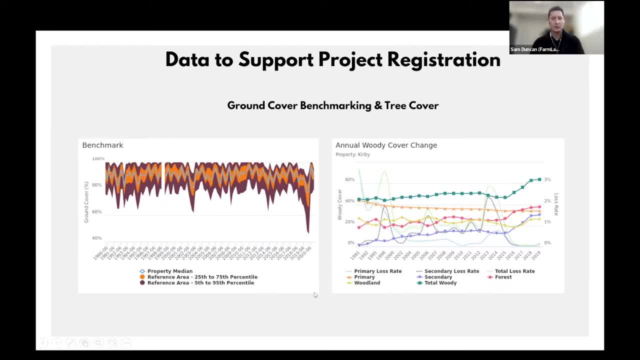 this is looking at ground cover. is that as that proxy for that change in soil carbon? so you know, we look at 2008 to 2012. you know, steady, steady increase here and so in ground cover the farmer and the land manager can link that back to a practice that they may have implemented and when. 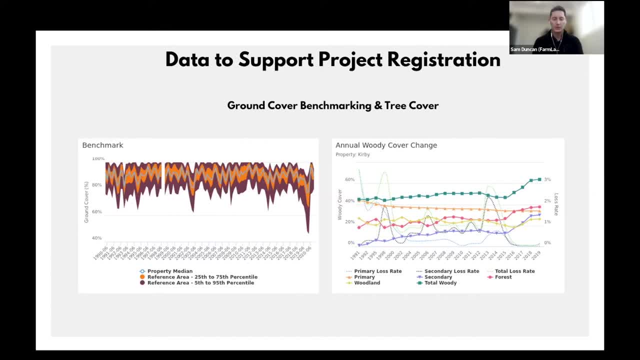 we come down to what you need, what you should be looking at trying to do when you build soil carbon. quite often you know what we we can refer to the literature, but the literature is still developing and quite often it's really good to link what the land manager has done in the past with the changes. 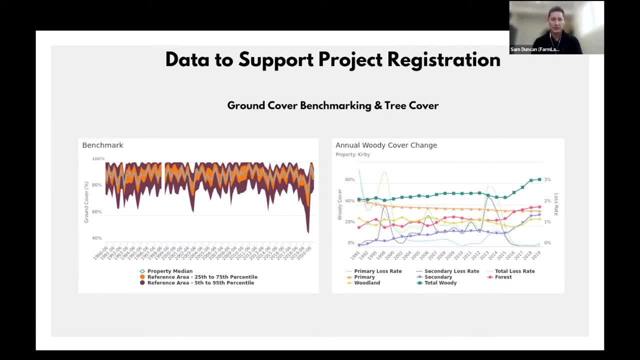 that they've had. and you know, as beverly said, a lot of this is due to climatic factors. so if you can remove that from the equation, you can build confidence, or the land manager can build some confidence around. um, all right, well, there was a drought there. so, you know, take that out of the 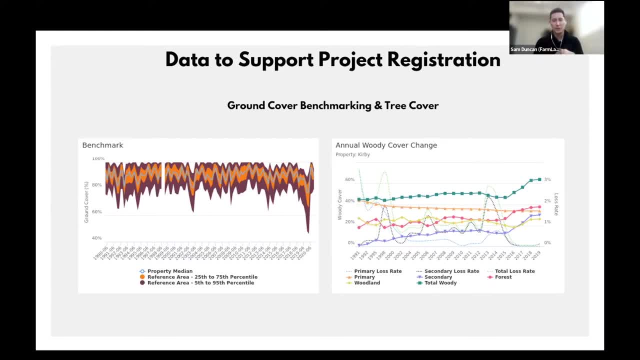 equation, but i had a pretty steady. steady period between 2008, 2012, um, you know, mean rain, median rainfall, um pretty consistent. but i changed this and this was the effect. so really important, because when we, what we're trying to encourage people to do is to generate um, where i think the literature 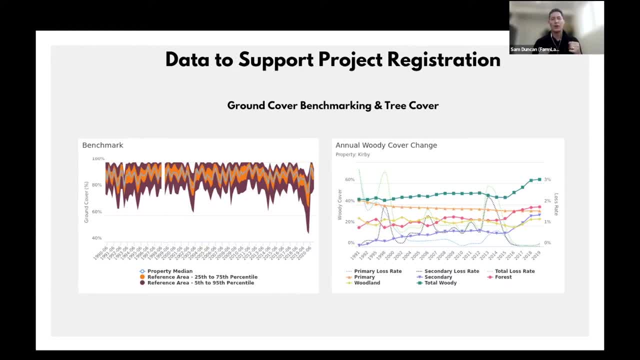 falls down today is we don't have a clear insight on the effects of the effects, of the effects of the impacts on. you know, if i do x, what is the impact on soil carbon, if i do y, what is the impact on soil carbon? and and some of these things are still evolving and it's causing a lot of, i guess. 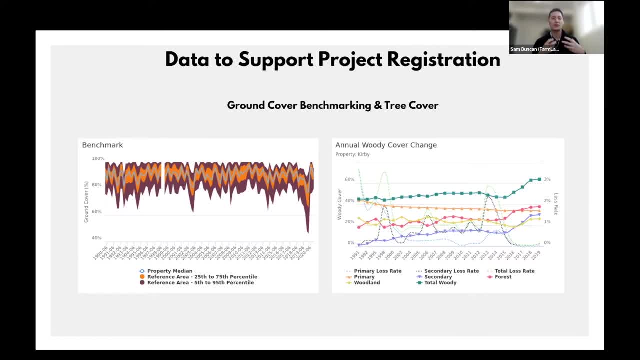 uncertainty in the industry right now. people. people won't enter. enter until they can manage that risk, until they know what to do. um, we have annual woody cover change here and this is really around land clearing primarily. this is used as a way to look at how much land can be used to. 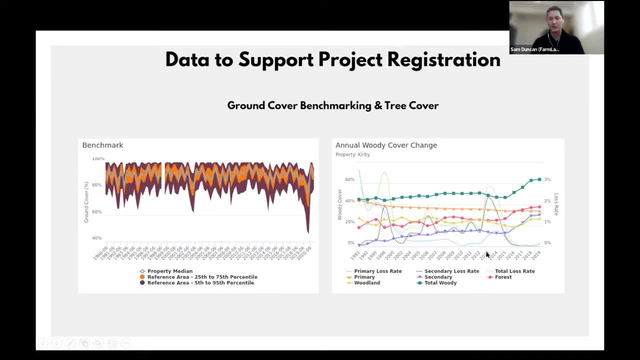 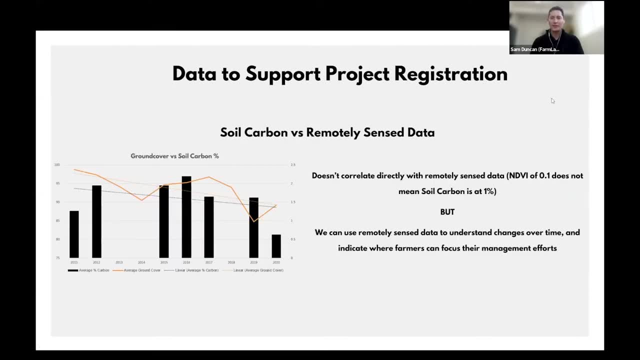 sequester soil carbon. so we simply remove the amount of um forested area- uh, greater than 20 canopy cover- from from the project area there. all right, so this was a little presentation. um, i've regurgitated this a few times, so this is great. 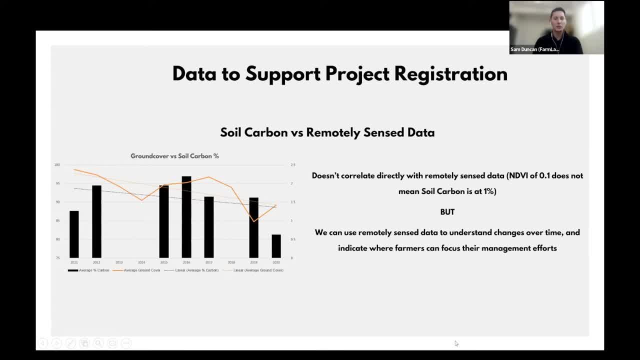 because this is what this graph here has done is we've mapped ground cover, now two percentage soil carbon for a local farm in um uh. in the region i'm based in um uh, i know one country, um armadale, new england, and this is a farm over in urella. so what we have here is the change in. 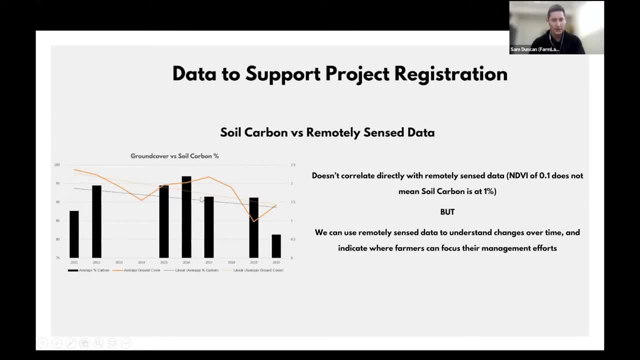 um ground cover, which is the orange lime. so you see a decline, pretty steady decline there until 2019. versus carbon test results averaged. this is um uh, if we've got percentage carbon yet on the right axis here, um averaged uh for for that farm and you can see a pretty steady decline over time. but but really importantly, there is a lag. 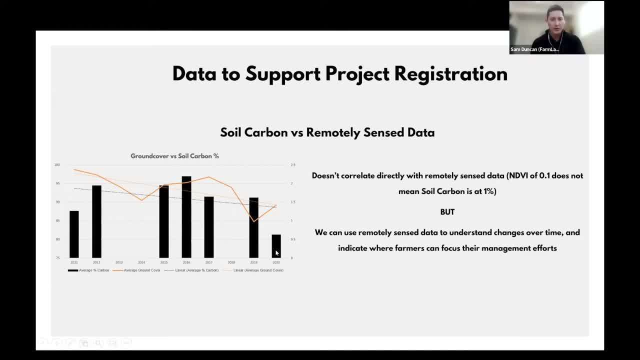 effect here. so after ground cover has dropped, we see a drop in soil carbon levels. um so really key to keep in mind is that there is this obviously um key thing in your um um imagination: um, um, um, um, um, um. one or five years measurement should be done between year one and year five. usually we see 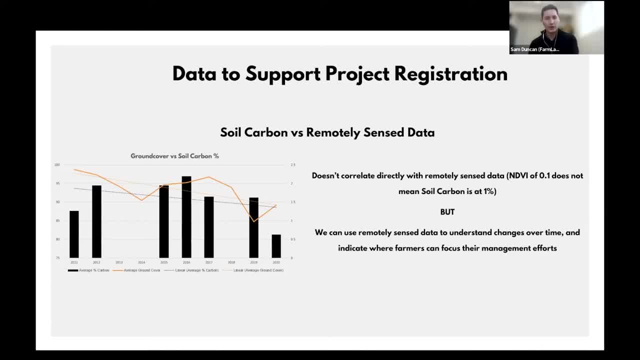 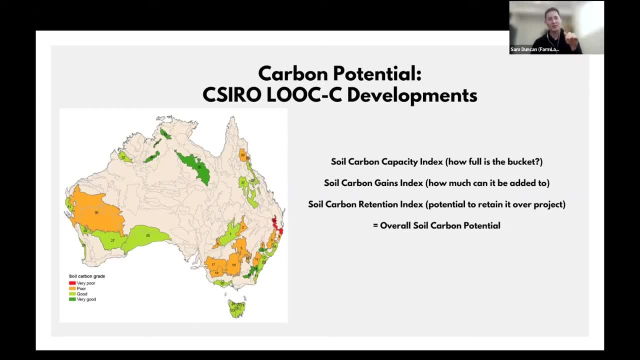 it done around year three or four, depending on what's happened in that time. now, one of the key things that i have to address for rachel is um- carbon potential across the landscape. um, and this was really hard when i was putting this this brief together, i was trying to trying to understand you. 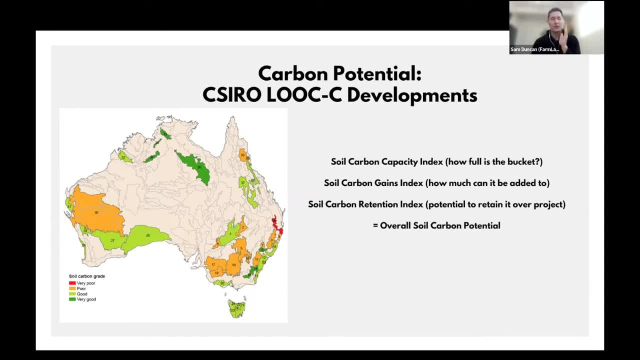 know what we're seeing. the challenge is um 90, probably 95 percent of projects, um carbon projects have been registered in the last two to three years, so they're yet to see an offsetting accrediting event. um, we are starting to see, you know, a few. come up now with a few of our clients and we're 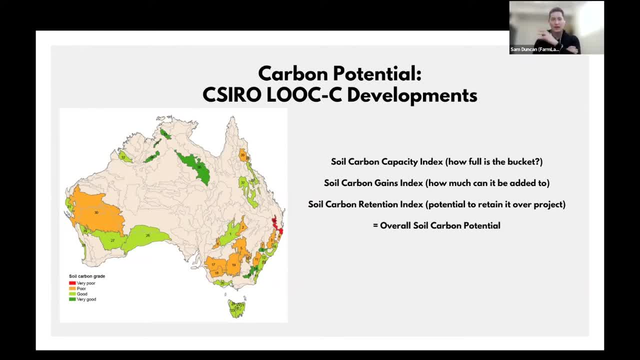 starting to see a few more. so it's really hard to actually gauge where things are increasing because of the events that are um we're seeing. we're seeing um increases and some of the things that we're seeing. um we're seeing um increases and some of the things that 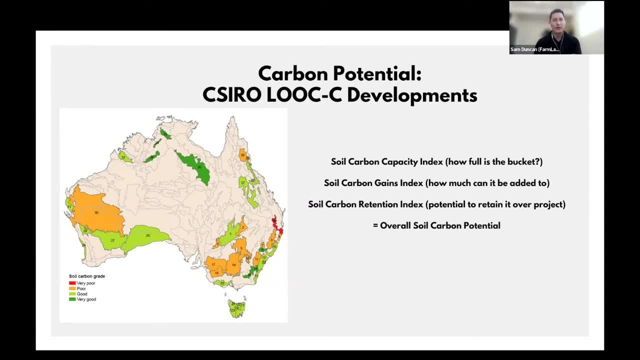 we're seeing um increases and some of the things that we're seeing um we're seeing um increases and all carbon they're, you know, few and few and far between. however, however, um what i thought i might do today: naughty, naughty, but um csiro, have some look c developments that we're currently working. 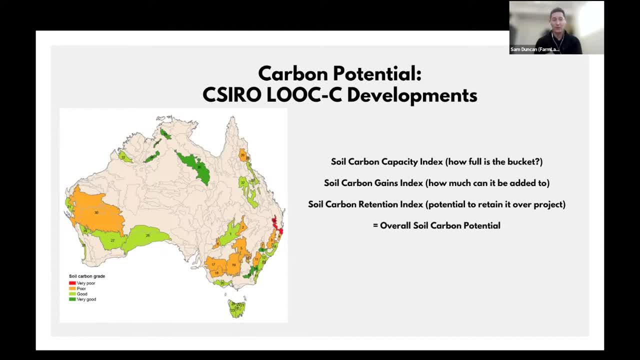 on them to uh to assess and uh provide them with feedback. um, if anyone wants to be part of this, we're more than happy. please reach out to me afterwards and we'll give you access to the tool through us, because we have to provide feedback to csiro on this and what they're. 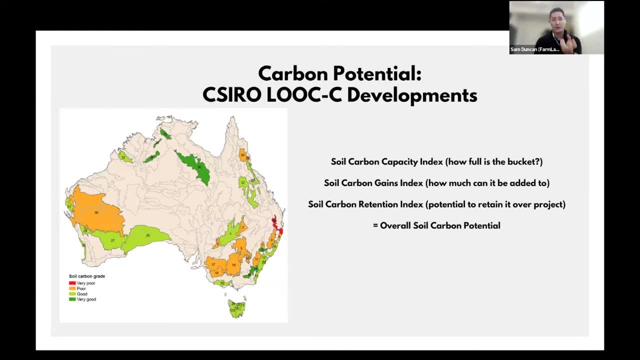 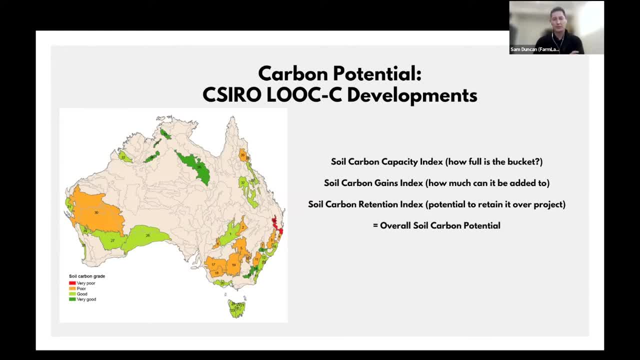 environment environment report, but it's very similar in terms of um. it's very similar looking to what csro about to produce and this is going to sit on top of the look c tool. so, for those that have seen the look c tool, it's a carbon calculator that will estimate carbon for a polygon that you 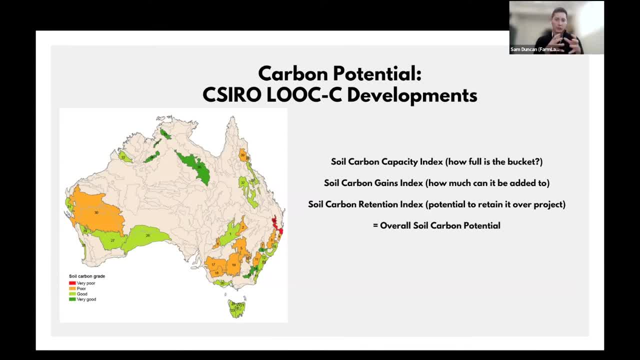 draw um, and this is an add-on. we're just going to also tell you for that area that you've drawn out the um capacity. so i'll just go through the little list there on the right: how your health full is the bucket, how, how um you know what's your potential to increase carbon um the gain. 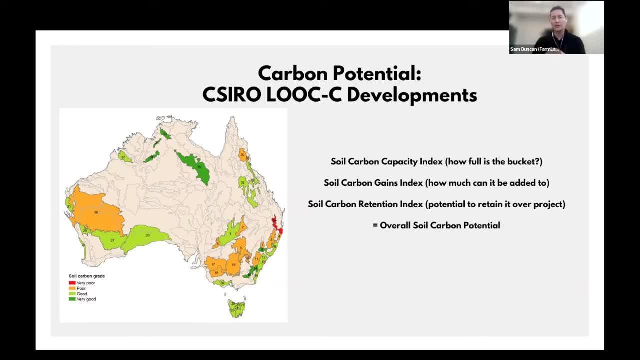 gains index, so how much you can add to that bucket. so you know, for the one of these green areas, you know you might have a max potential of five percent but you might be sitting at one percent carbon right. and then retention, which is about how long, how likely you are to retain carbon based on 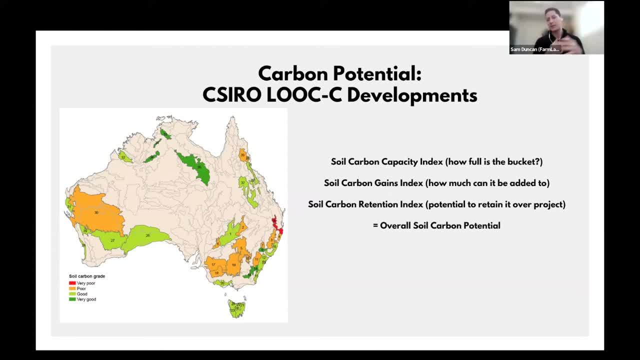 climate, climatic factors and a whole bunch of other things that csiro put in there, and all of this is going to contribute to an overall carbon potential score. so, like i said, we've got access to this tool. we're looking to- um, uh, looking to sort of push. 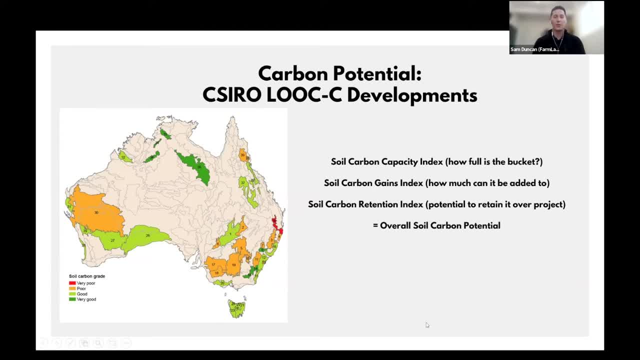 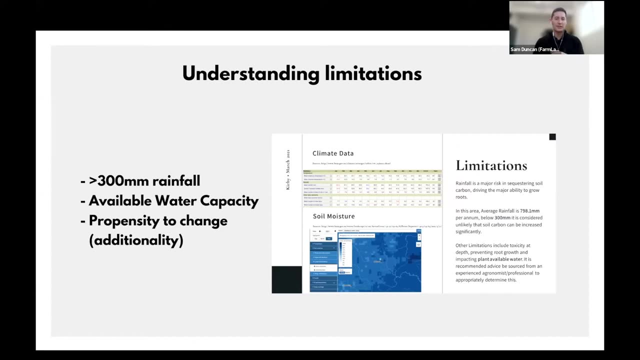 this out and get some feedback on behalf, you know, behalf of csiro, and it will help hopefully assess, um, hopefully make um land managers, um, uh, give land managers a bit more insight into what their potential is across the landscape. um, yeah, so some of the key things when it comes to understanding. 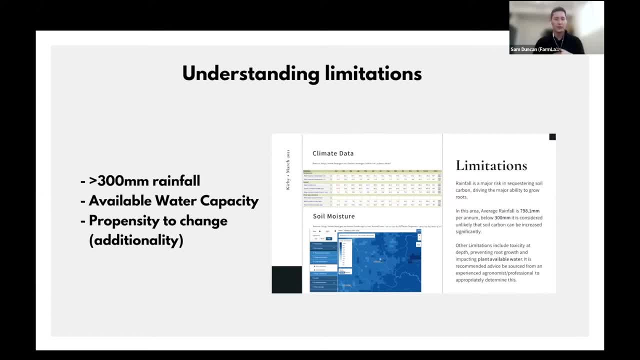 limitations. and these are some of the takeaway- key takeaways for um- for you to think about before you enter a project. are you greater than or less than 300 mils in rainfall? um, if you're less than 300 mils of rainfall, very, very hard to sequester carbon between three and four hundred mils um. 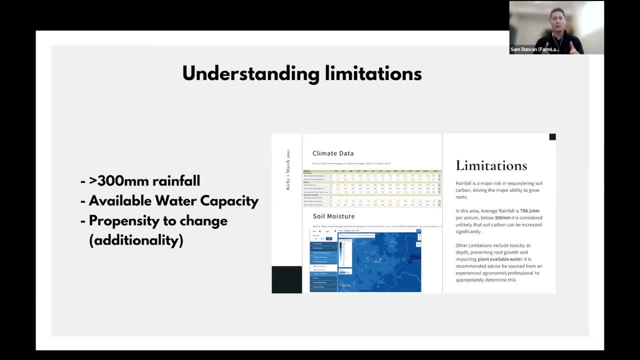 you know possible. um again, it's quite difficult but you know can be done. just looking at really emphasizing some change in land management practices, um, for we're here in new england and a lot of our projects and clients are here in new england out, you know, with sort of six. 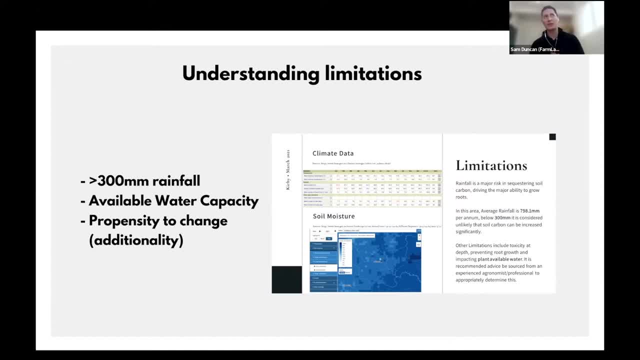 seven hundred bills. i mean this year it's probably been about two thousand mills. it's been reduced so far it's not so that's quite ridiculous. um, not quite. but um, you know, higher high rainfall and lots, of, lots of potential um available water capacity and this comes back to that clay. 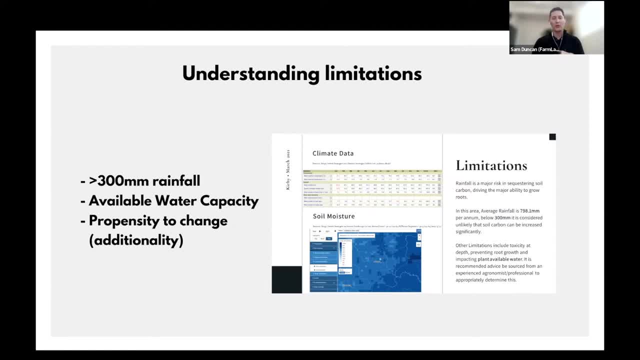 you know that biograph, that beverly gate, before we had sort of clay being one of the primary primary drivers there. you know, available water capacity is just a um, uh, i guess a more advanced way of saying clay, clay content absolutely. soil type is really, really key because you have to be able to 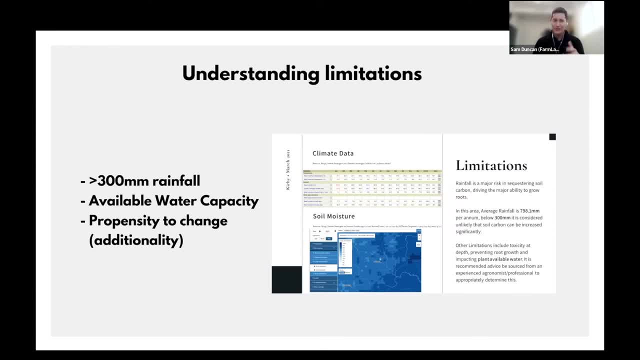 grow those roots to sequester carbon um. and the last one there is interesting: it's propensity to additionality, which is um, which is really tough, right, this is what management practice can a land manager introduce to sequester carbon um. rachel, how am i going through time? sorry, i do have a. 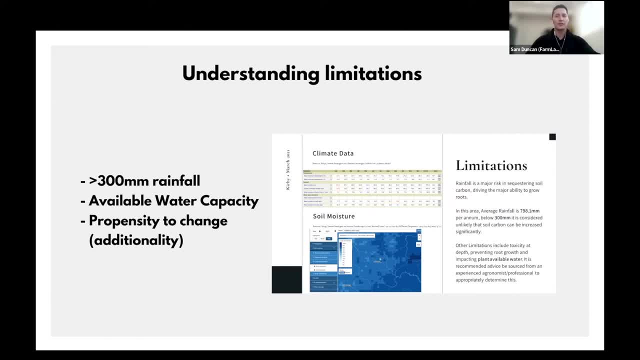 timer in front of me. you can have another minute if you'd like. sam, give me one more minute and i'll fly through the rest, because i've covered off on all the really exciting things. i can answer the rest. so, um, i have a few slides here on how a project is registered. luke's going to cover this. 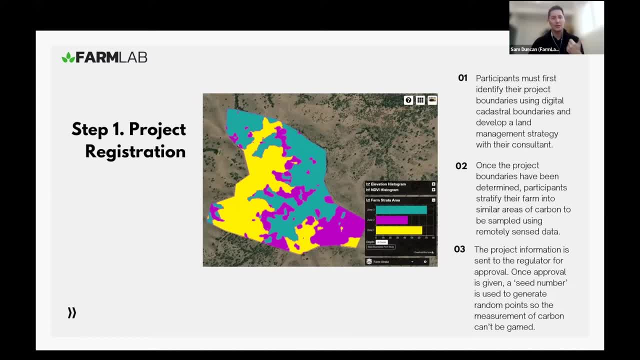 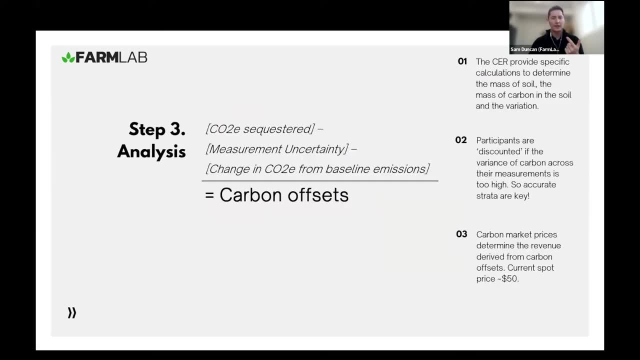 a lot more, a lot more detail, so i'll just skip through. but basically stratification, so you know where to sample. submit that sample plan to luke, luke approves it, and um, it's then set, sampled and measured, nice and easy, and then we calculate the amount of carbon offsets and we produce something. 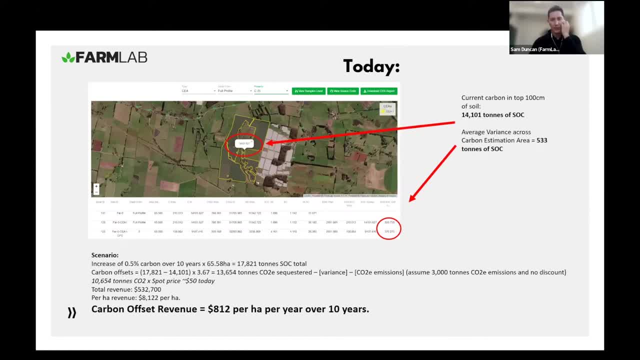 that looks like this, and so this is the. this is the end result for a carbon project where, at t0, we had about 14 100 tons of carbon in the top 100 centimeters of soil, and this is really the number to be. so when you enter a carbon project, this is sort of the first number, um. 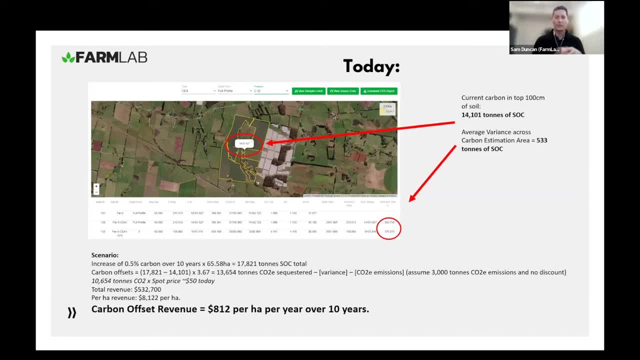 david. david allen could probably talk about his experience, i know, having gone through sort of this baseline sample around himself. um, you know, this is where a sample has come out. the project's been registered and now he's got that number there and he's now implementing some changes to um. 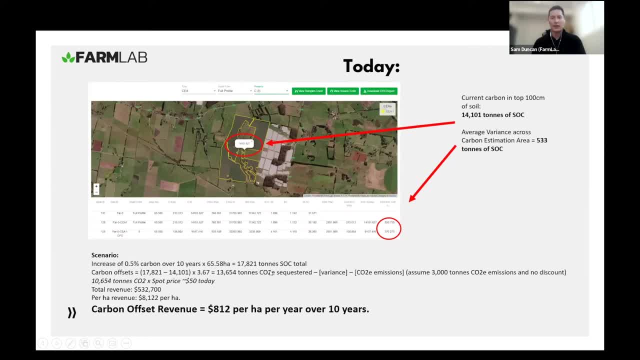 hopefully increase this where what happens next is that then you go out in three to five years time, or one to five years time, and you try and you remeasure after you've implemented these management practice changes, and you look at the difference. um, if we assume, just to give you some, 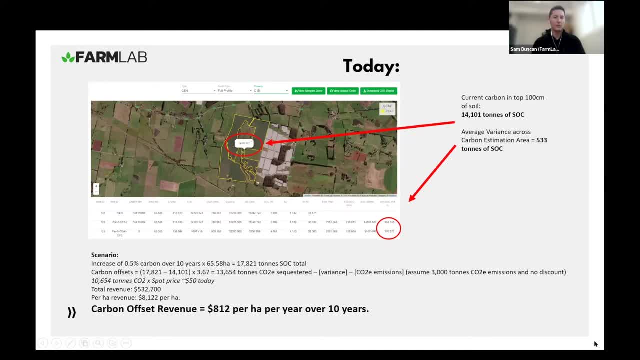 uh, reasons for your need for carbon, um, and there's this one time or another event you've you know we've got to bring this in. i've got to bring in more people- is, if you're in this environment, it's because there's a lot of things that have to be done, and i i'll talk about this. 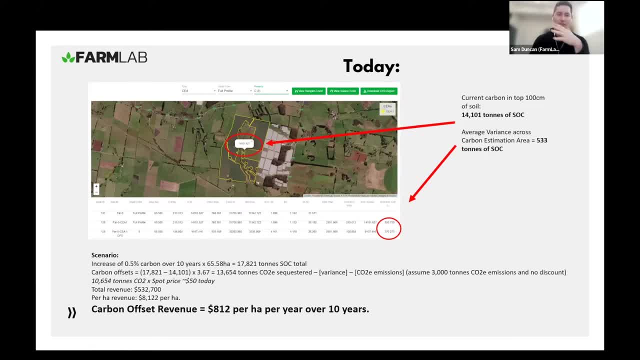 later. so, in terms of what you can do, um, if you're in a, in an environment, if you can't access it because you've gotta have your own, um, energy is you've got to have a few different technologies to go around and try to find what's right for you. you're going to have to make changes to your. carbon, but you're not going to be able to get that out of the organic environment in there. so, um so, everybody loves you, know this. you know everyone wants to know how much you can actually make doing this. right, we always we will talk about the environment, but there's also this other driver. 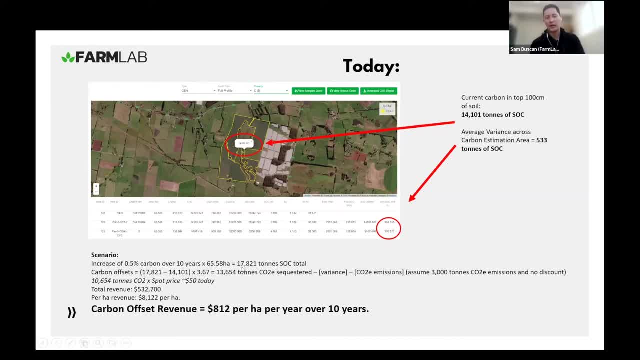 that over 10 years, which might be achievable, we get that. we ended up with an end amount of carbon of 17 800 tons. the difference between 17 800 tons and 14 101 times is about 3 000 tons. sorry, um yep. 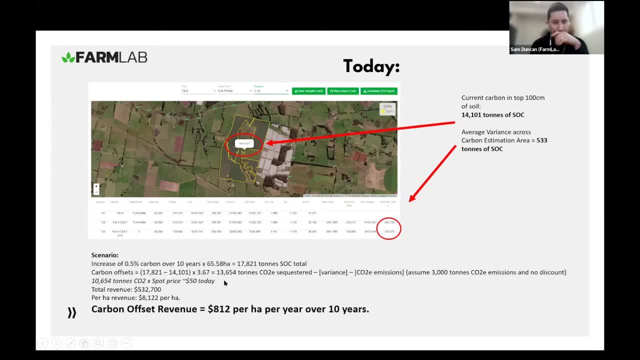 3 000 tons and then we multiply it by a constant of 3.67, which is the constant to convert co2 equivalent um from from solid carbon. then we subtract. we subtract variance, which is an indicator of accuracy i'll talk about. i can answer this in the q a. we subtract any change in baseline. 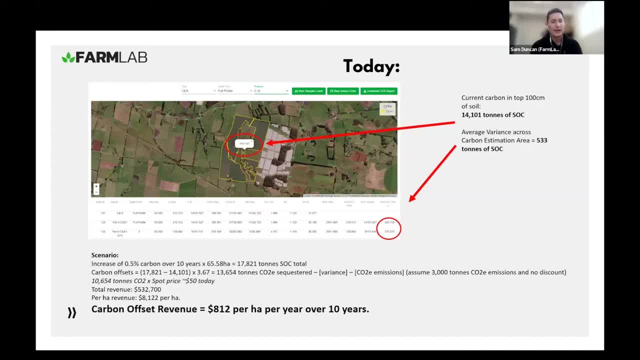 co2 emissions from that farm. most importantly, um, we then end up with the total amount of carbon, in this case 10 654 tons of co2, at a spot price. i don't think it's quite fifty dollars today, but let's assume fifty dollars. we get a total revenue of five hundred thirty two thousand dollars over. 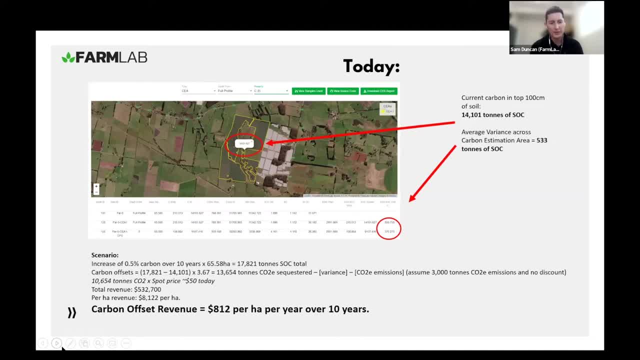 the quarter about ten year project um per hectare. eight thousand one hundred and twenty two dollars per hectare, or eight hundred and twelve dollars per hectare per year over ten years. um, i think that's correct as far as my math goes. yep, um, uh, i've looked at this enough, so should. 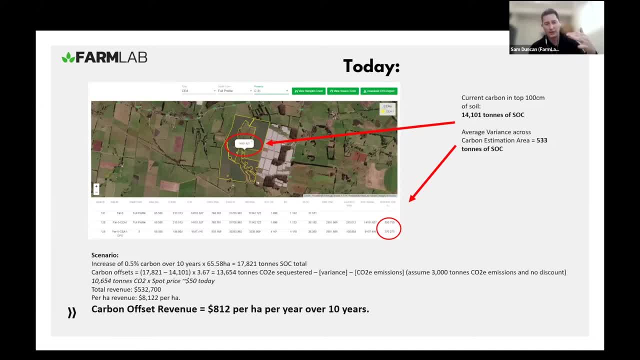 be right. so that's sort of what it equates to now. that's, if a land manager can get to that point, five percent increase. and the key thing is: i mean, this is all the easy stuff, right, this is all calculating it, but at the end of the day, somebody has to actually 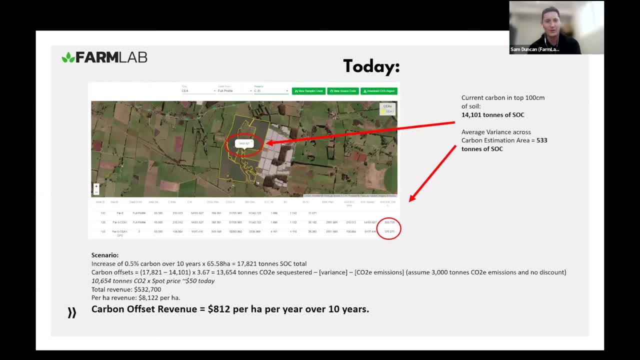 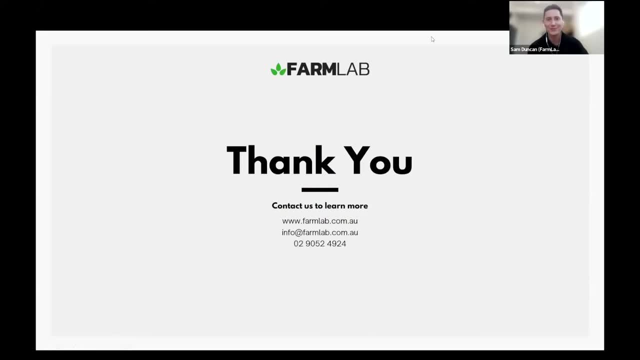 drive up carbon and do so consistently um across their property and that's um. that's about it. a bit of the amount modeling, but thank you very much. so um, thanks, rachel. sorry i think a little bit over time, but perfect. thanks so much, sam. that was super interesting and i really enjoyed all. 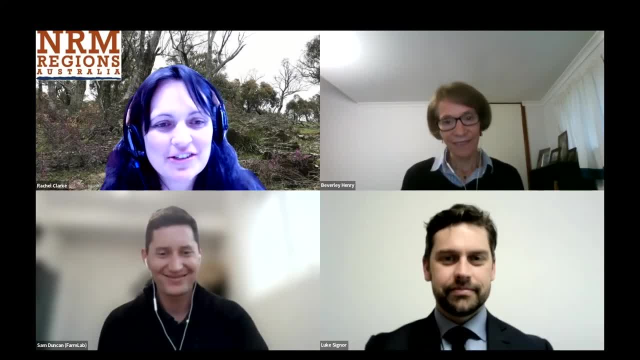 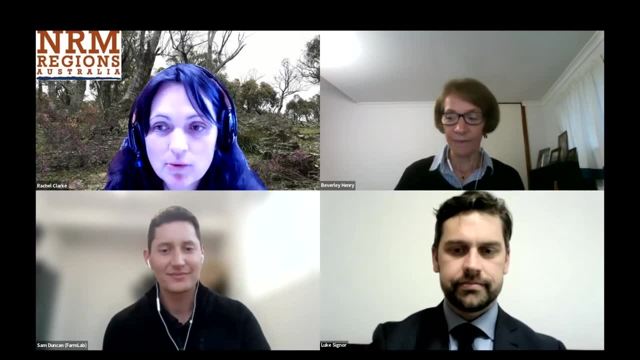 your maps. so thanks for um, for showing that, for showing sharing that with us, and um, and also i was really interested to have those figures there at the end. i'm sure people that you know are farmers that are involved with farmers really looking for some of that um, some of those numbers. 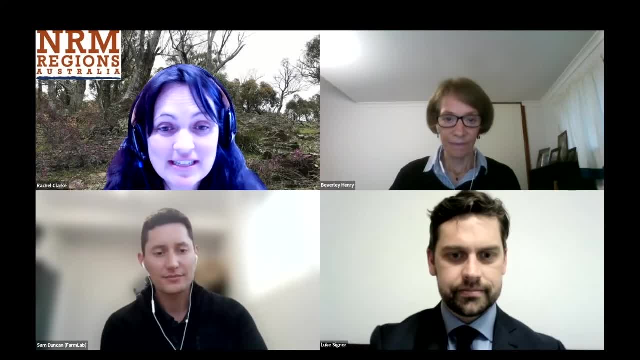 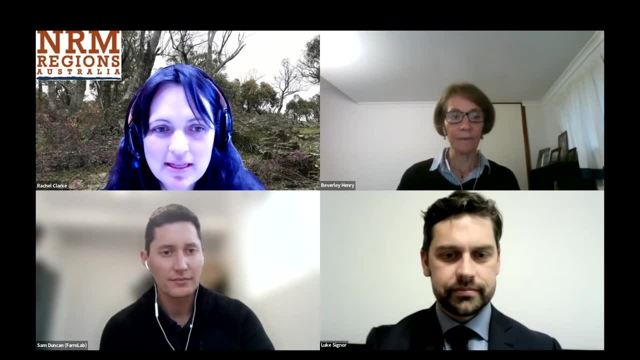 so thanks so much for for popping those in. it was fantastic. um, i just reminded everyone to keep your questions coming in. i have seen quite a few flowing in, so thanks to the people that are putting them in there. so our third speaker today is luke senior, the assistant manager in 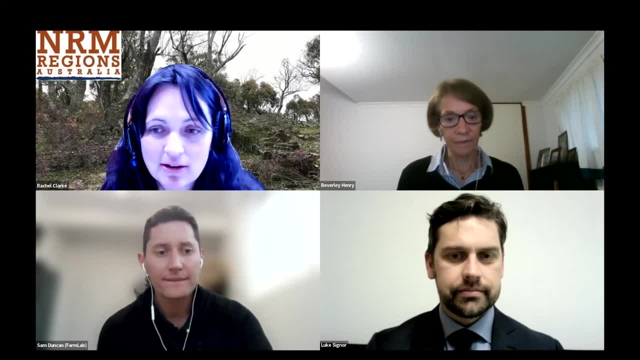 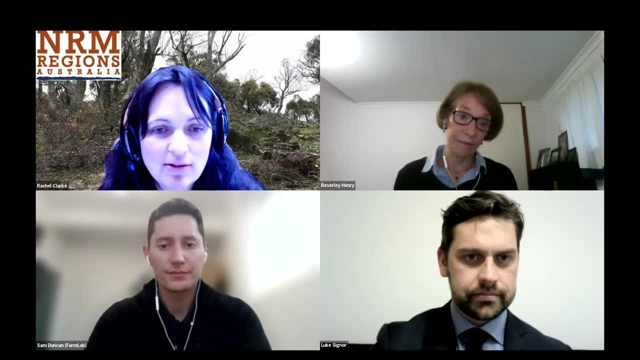 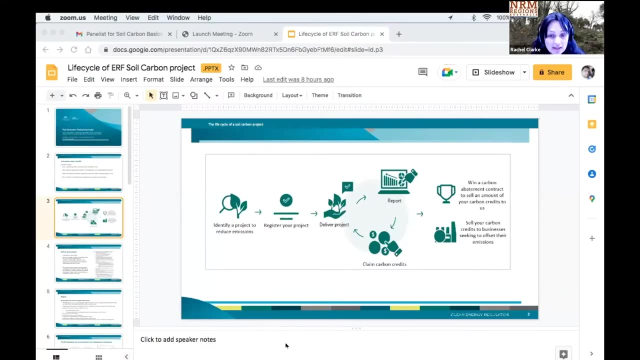 the savannah agriculture and soil carbon credits team at the clean energy regulator, so you can share your screen now if you'd like to look. so luke's primary role is the facilitation and regulation of soil carbon projects registered under the emissions reduction fund, and this includes managing the registration, crediting and variation of any projects in 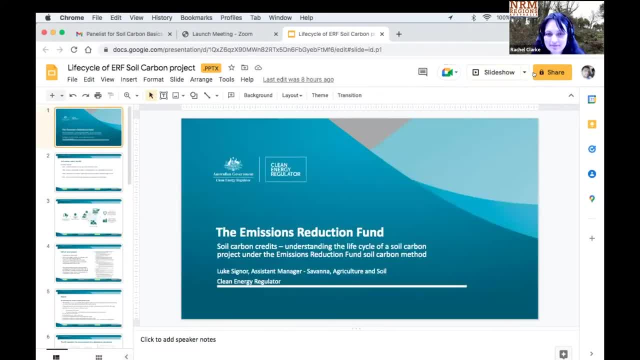 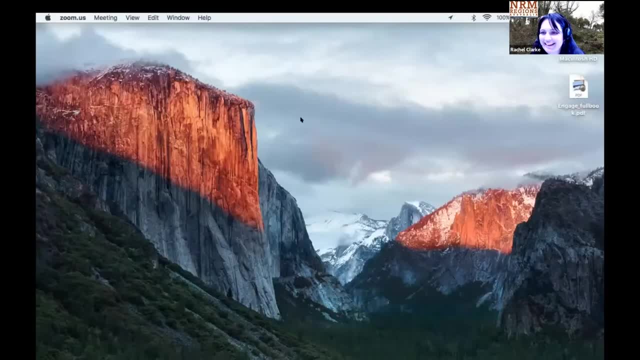 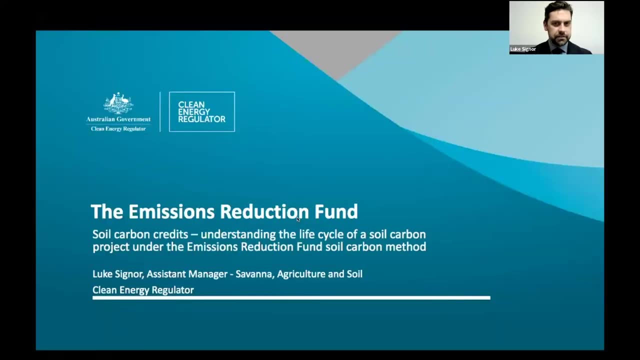 the soil carbon space. so thanks for joining us, luke. so you're still muted, i think so sorry. thank you so much. let me bring up these slides. so thank you very much for that warm introduction um luke signor, the assistant manager of the savannah agriculture and soil team. 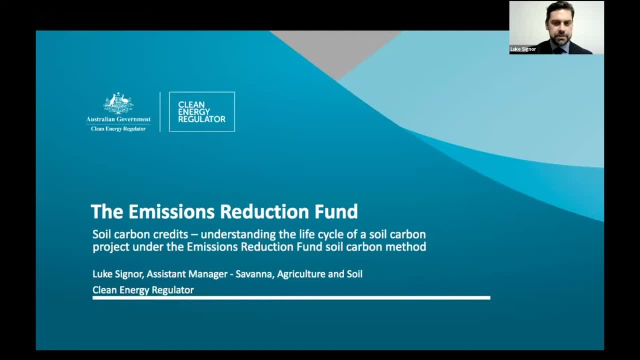 at the clean energy regulator. don't let the name for you. we also take on blue carbon. um, we haven't added that to our name yet. i'm sure it'll get there soon. i'm going to give you a very, very high level brief introduction into the life cycle of a soil carbon project. it's a little bit different to some of the other. 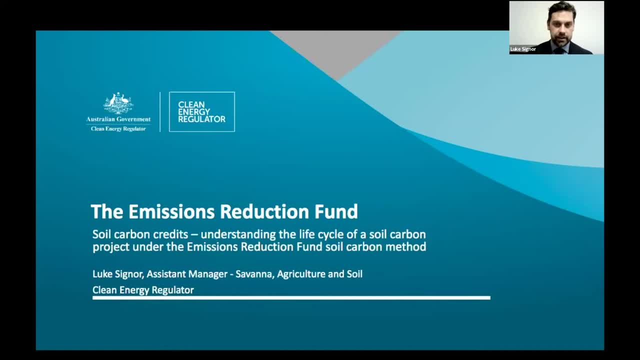 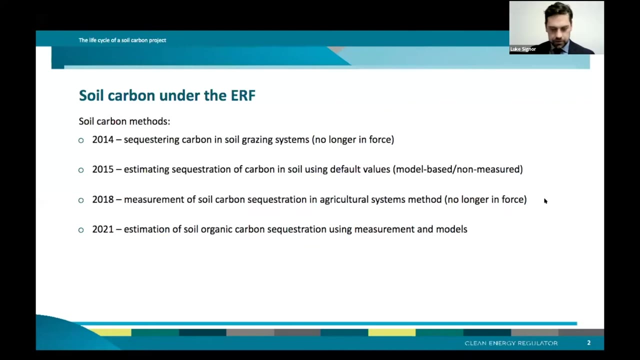 emission reduction fund projects that run at the cer. so i just wanted to make sure that everyone understood what their responsibilities are if they were to be a participant under this scheme. so, first of all, um, we've had a few people mention that, yes, there are. there are two active methods for soil carbon at the moment, which is the 2015 method, which 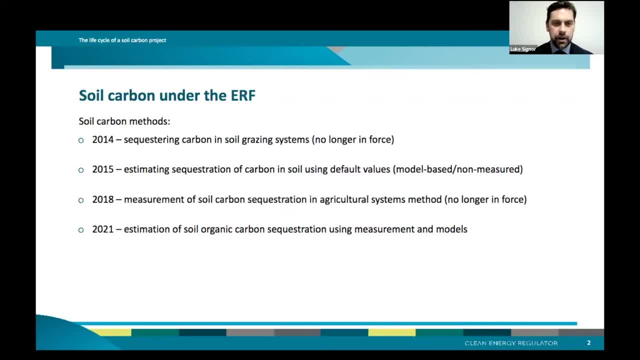 is model based or non-measured, and the 2021 method, which was released at the end of last year. we have projects that are still registered under 2014 and 2018 uh and generally we expect most of those projects to transfer across to the 2021 method for reporting. 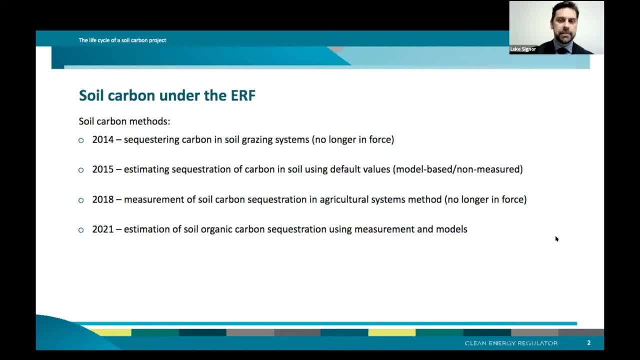 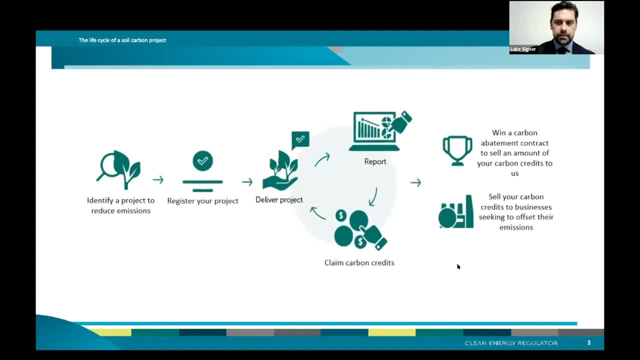 uh, to take advantage of some of the the advantages that the newer method has, this is a graphic that's thrown around our agency a little bit. um, it's very, very general um pictogram about how the projects work, so you would identify the project that you want to run. for example, you want to register a project under soil carbon. 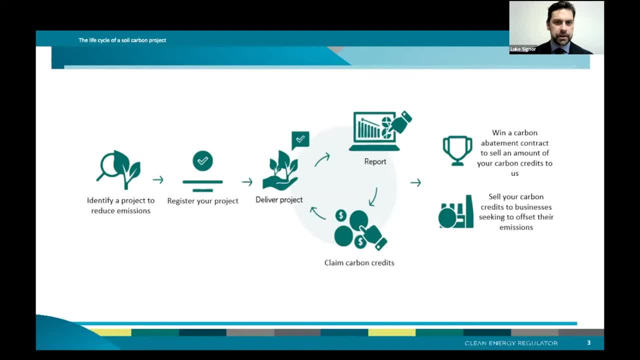 because you see a potential to sequester additional abatement in your soil, you apply to us to register the project. there's eligibility criteria that we assess and then, if the project is eligible, the project is then declared. from that point you would deliver the project, which involves. 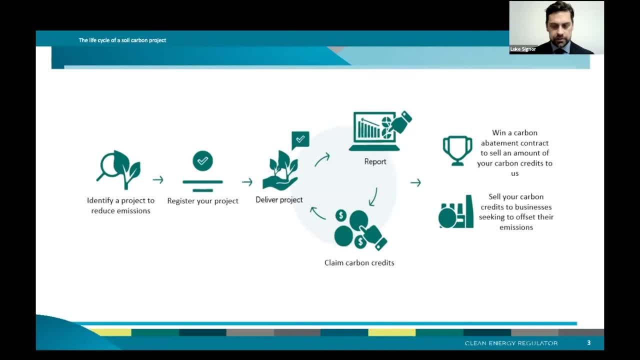 implementing your new activity, which i'll go into shortly, and then also taking your your measurements, so that includes a baseline and a subsequent. you get that soil analyzed and then you write the offsets report, you submit it to the regulator again for an assessment and if there's been genuine calculated and measured abatement, you are issued carbon. 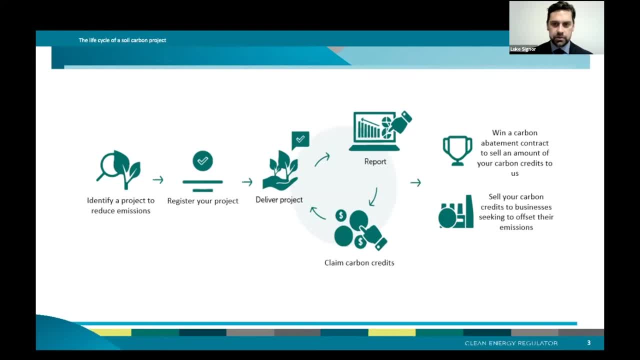 credits. one carbon credit is equal to one ton of carbon dioxide equivalent units removed from the atmosphere. you can then choose what you want to do with those carbon credits. you can sell them on the free market as a commodity, or you could sell them back to the regulator if you have a contract. 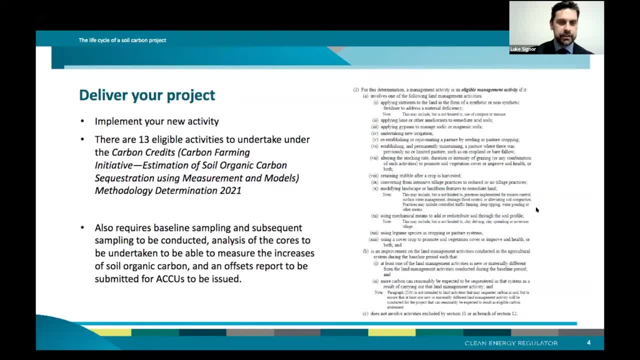 and now i apologize, this slide does look a little small, but when you deliver the project, you're implementing one of the eligible activities that are stated within the method. so there's 13.. um, they're listed there. essentially, what we're looking for is a new or material difference to what you did during. 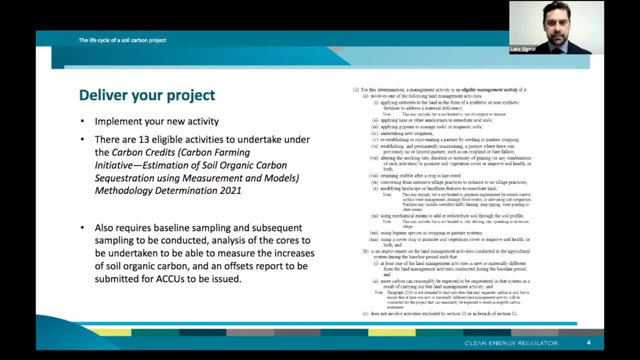 the baseline, which is five years, before you apply to register, so you can apply nutrients, lime or gypsum. you can undertake new irrigation, change your stocking rates, rejuvenate a pasture or use a cover crop, provided that it's something additional to what you did in the past five years. generally we'll accept that as a new activity and that's the activity that you will. 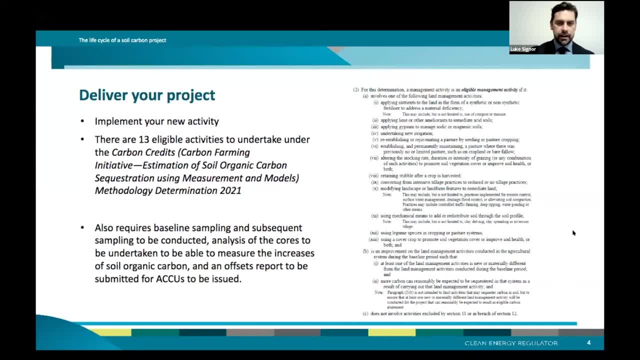 be credited on and, as also i mentioned in that first reporting period, you'll need to do a baseline measurement to take, take the stock of the um, of the carbon that's in your soil at the beginning of your project, and then you'll have to do another sampling round to measure the increase between one 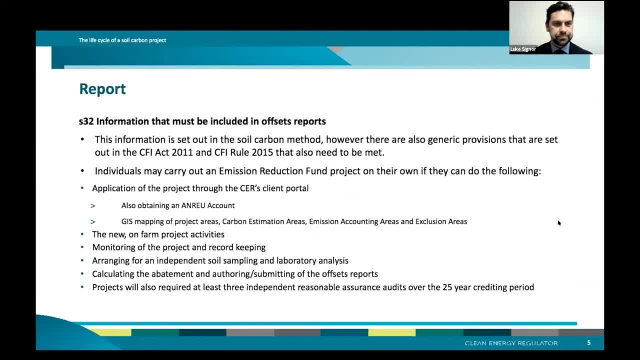 and five years later now, the report? um there's uh this information is set out uh under the method. um it's section 32 for those who are very interested. there are also generic provisions for all emission reduction fund offsets reports um to be met under this the carbon farming initiative act and rule uh the reason why. 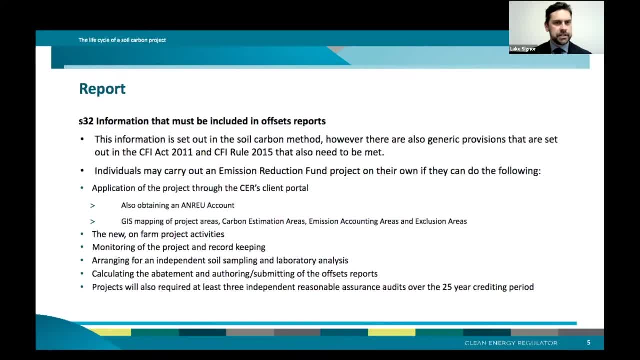 i bring this up is because we often have questions from individuals who want to run projects. uh, and it's advised that, if they feel that they are confident in meeting all of the requirements that a proponent needs to meet, uh, you can um, however often, uh, we see carbon, um, uh, carbon. 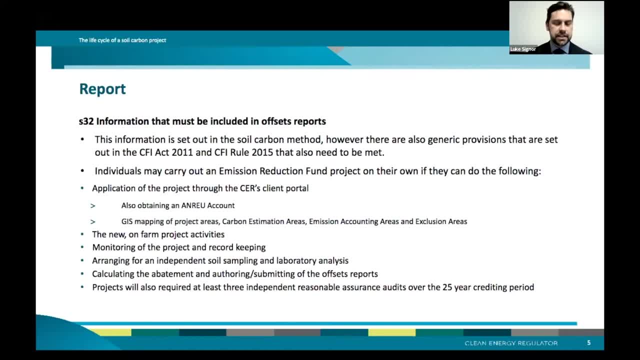 project, uh, project developers come along and assist those um, and that could be a private um commercial relationship between yourself and those providers, um. but it's just important to note that you would need an anru account. you would need to be able to do your geospatial mapping of the project area and 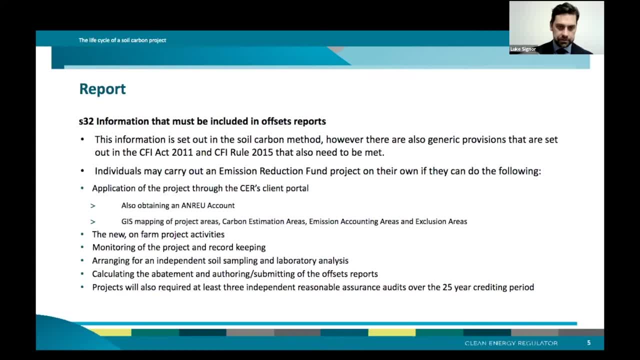 carbon estimation areas. you'll then have to implement new activities, monitor the activities, arrange for the soil sampling and laboratory analysis, calculate the abatement and put in the offsets reports and then also ensure that you can get three- at least three- independent, reasonable assurance audits over the 25-year credit. 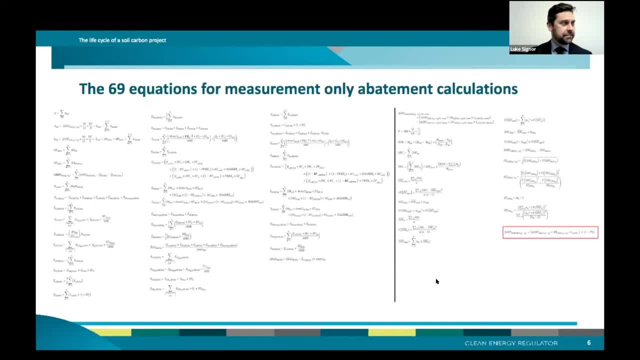 in period um. again, if you've got a small screen, the effect has probably lost a little bit here, but these are the 69 equations from the method uh that are used um to determine your abatement. a lot of them are about determining baseline emissions, um. some of them are about determining. 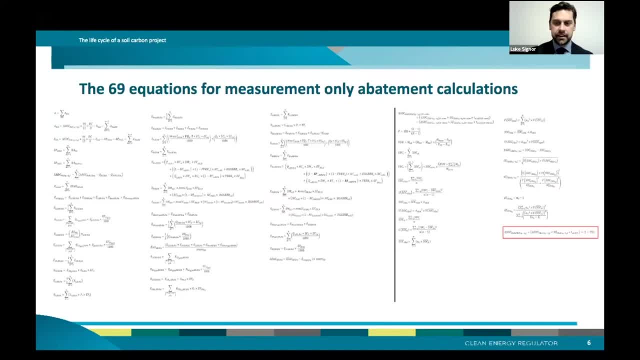 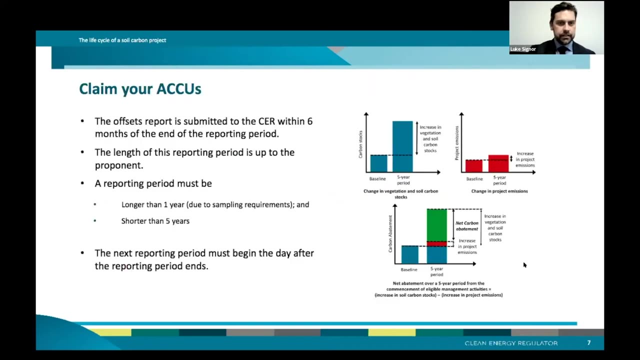 the percentiles of the of the cores that you've collected uh. and the final red box down here is, once you have all this information, um the amount of uh accuse that you're going to be issued for that reporting period. so if you have uh measured an increase in your soil organic carbon. 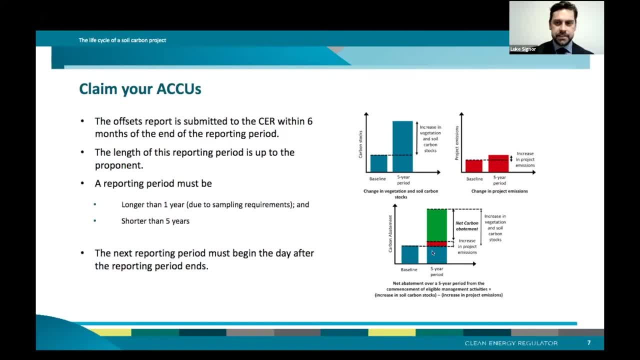 and you've put your offsets report in um. this is just a very simple um infographic about how, how many credits you're issued. so we have a baseline measurement, which is this much, and then there's been an increase in the amount of um, uh soil carbon stocks in this portion uh, and then we reduce, uh the number of credits that 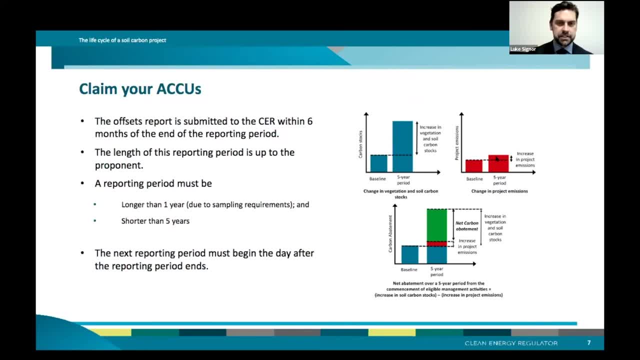 you're issued by the increase in the project emissions for carrying out that project. um. those reports have to be submitted within six months of the end of the reporting period. um you decide how long those reporting periods are, provided they are longer than one year and shorter than five years. 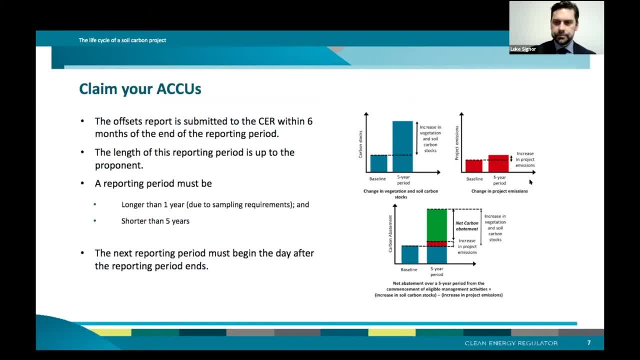 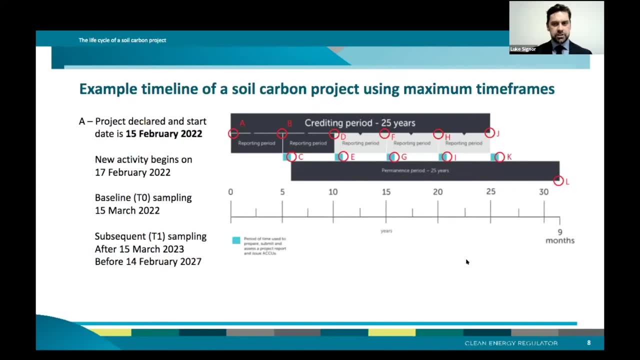 and these next few slides are. they're all very similar, but this is essentially the entirety of your crediting period. so there's some key dates here and they're assuming a few things. one, you're doing your sampling at the very last minute and two, you're using a five-year reporting period. 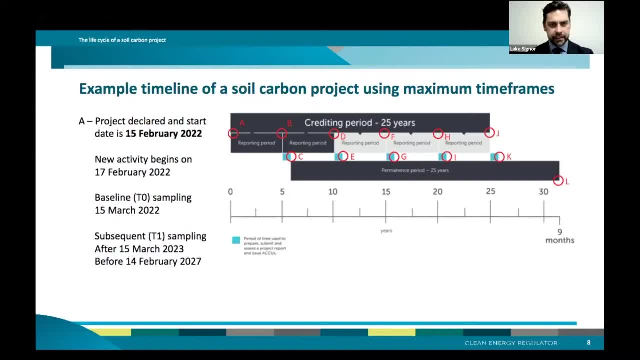 so if your project is declared on the 15th of february 2022, you can begin your new activity immediately, and then you're organized. so you've organized to get your baseline sampling completed on the 15th of march. you then have to wait at least one year to do your subsequent sampling. 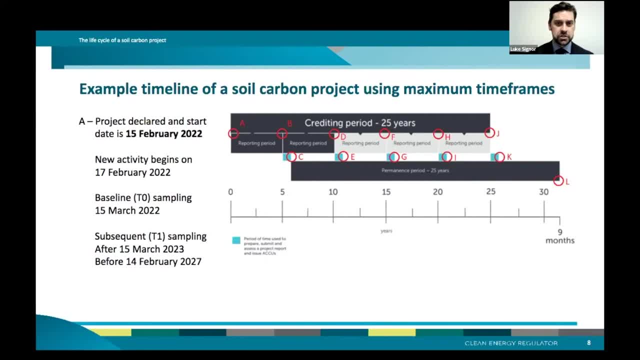 and the next round of sampling has to be completed within the first reporting period, so that's before the 14th of february 2027, so you can begin your new activity immediately. and then you're organized. so you've organized. then your next reporting period will begin on the 15th of february 2027. 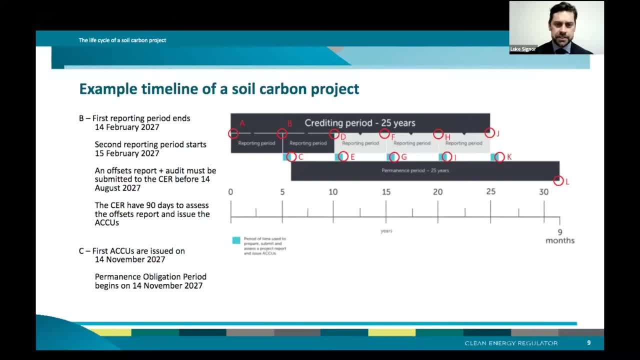 you'll submit an offsets report and an audit before the 14th of august 2027 and then the cer may take up to 90 days to assess that offsets report and issue the accuse if the first issue um instruments of accuse is on the 14th of november. 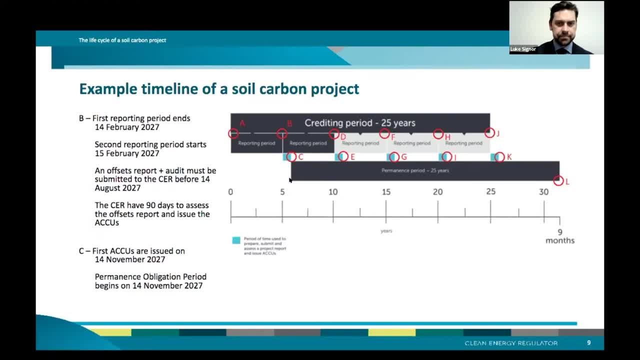 this is when your permanence obligation period begins, and then you're going to have to submit a report on the 15th of february 2027. then you're going to have to submit a report on the 15th of february 2027. 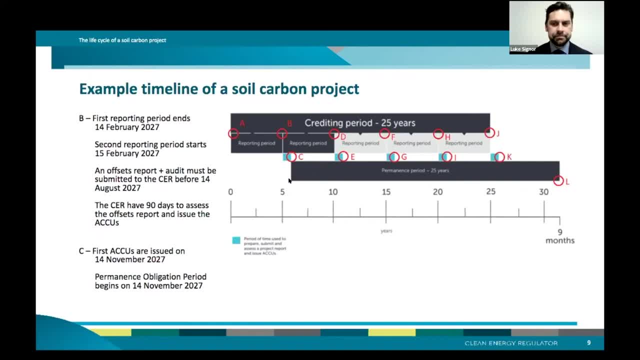 it's. it's fundamental to the scheme that um you are maintaining the carbon that you sequestered into the soil for that period of time. ramifications of not continuing the project activities or revoking the project because you no longer want to participate is that you may be required. 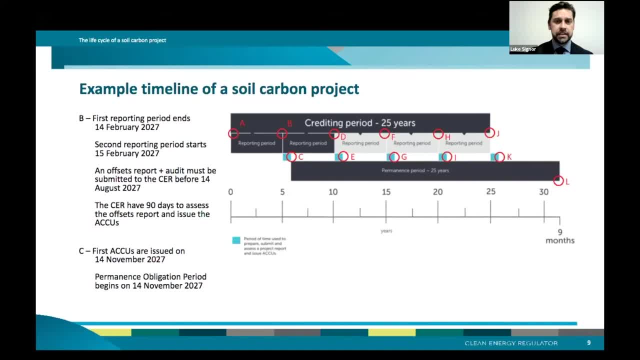 to relinquish some or all of the accus that you've been issued to date, and i'll quickly just click through- um, pardon me, um- through this, through this graph. it's the same process over and over again, so you would need to have another sampling round at some point during that reporting period. 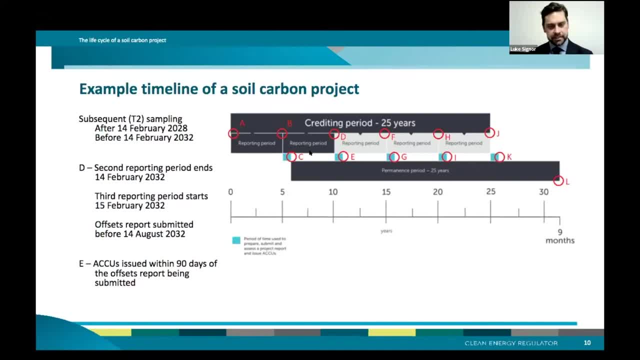 you then get the data, write your offsets report, submit it to the regulator and we issue the credits. and i will just briefly mention that. um, as part of that eligibility assessment of your project, uh, you must have a land management strategy which includes information about how you will maintain the sequestered carbon in your soil for that permanence obligation period. 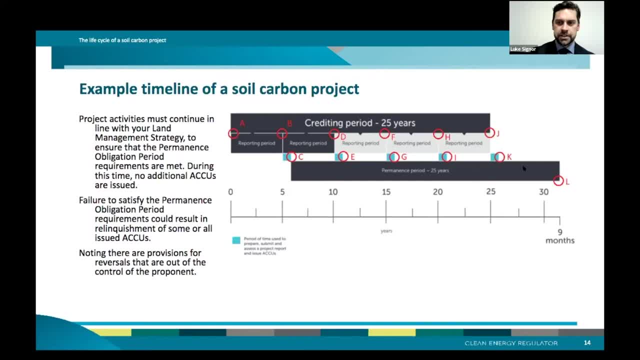 there is this period between k l, with the project activities are expected to continue, but as the crediting period has finished at j, there will be no further accuse issued for that time, um unless there is a a review of the method and it's determined that it can continue, And that process is done by eRAC. 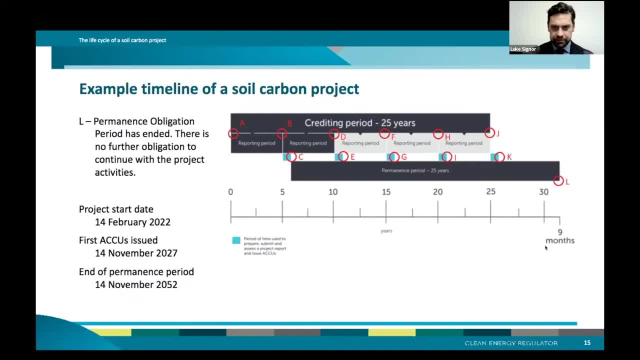 So just the final word on dates. If the project is declared on the 14th of February in 2022, it's expected that this project will likely continue until the 14th of November 2052.. So you were issued for 25 years worth of credits, but the project activities would. 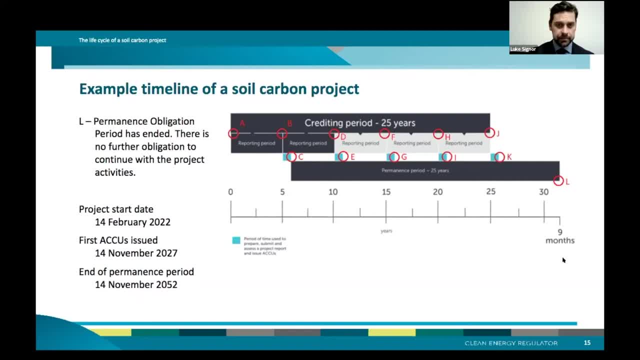 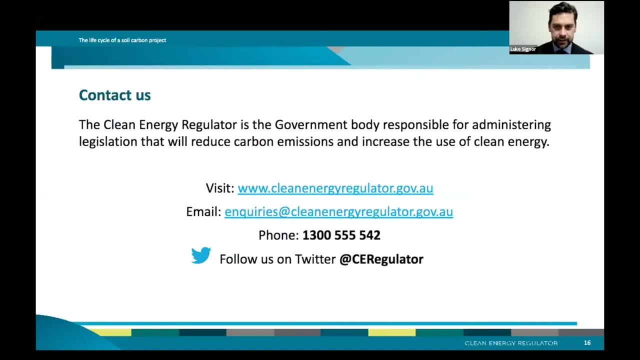 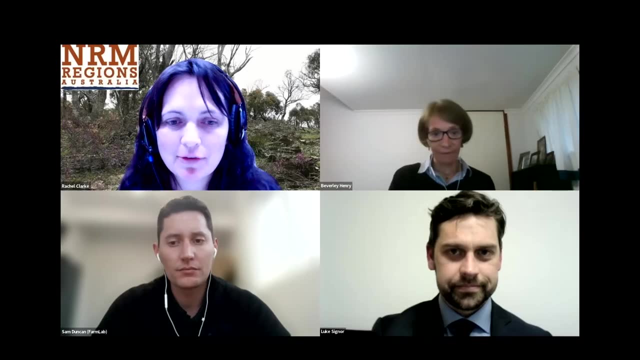 have to continue until for 30 years and nine months, And that's about it for me. Sorry, I went to touch over time. Now, if you have any questions, you can contact us there. Thanks so much, Luke. We have had lots of questions come in for you actually. 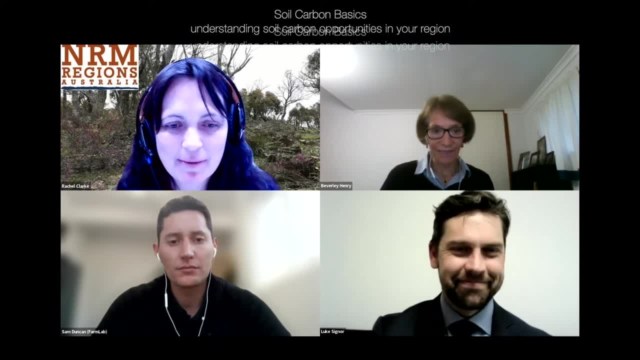 through your talk. I think there's a lot of detail in that presentation. Looking forward to unpacking that. Thanks so much, Luke. We have had lots of questions come in for you. actually, through your talk, I think there's a lot of detail in that presentation. Looking forward to unpacking that. 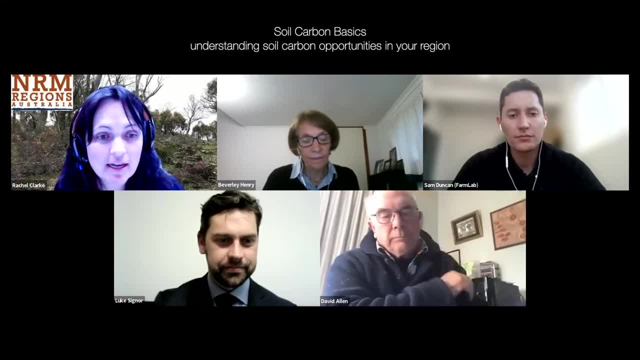 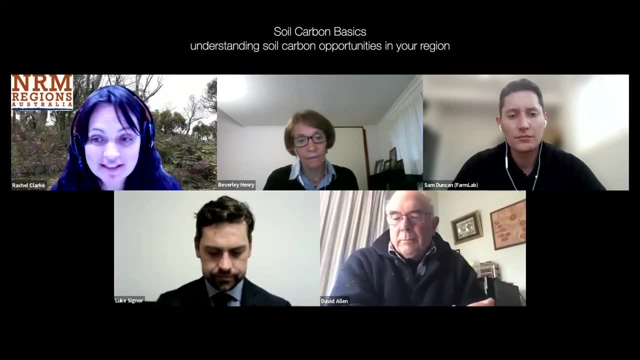 picking a few of those details during the panel session, But we will. we are going a little bit over time, So I'm just going to pause there and introduce and welcome our final speaker, who's been patiently waiting for his turn. So we've got a farmer, David Allen David's, from. 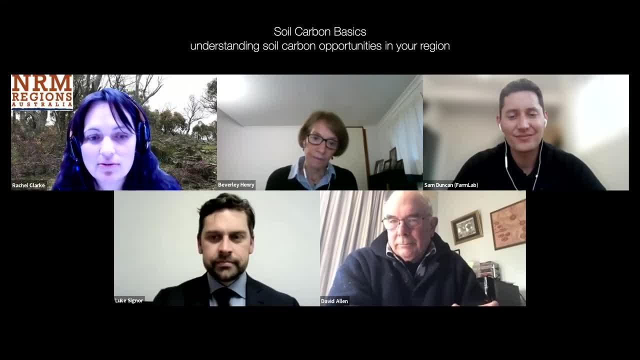 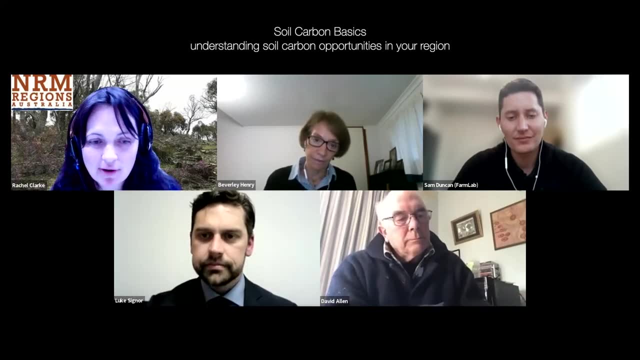 the Corangamite region in southwest Victoria. David runs a beef, wool and cropping farm that has been in the family for 116 years. David's been involved in land care for around 30 years and he's currently running a soil carbon project on the family farm. 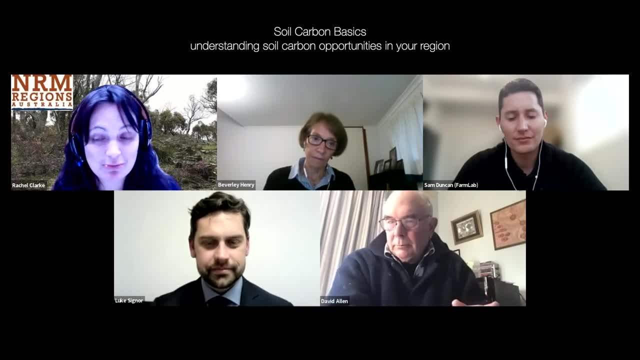 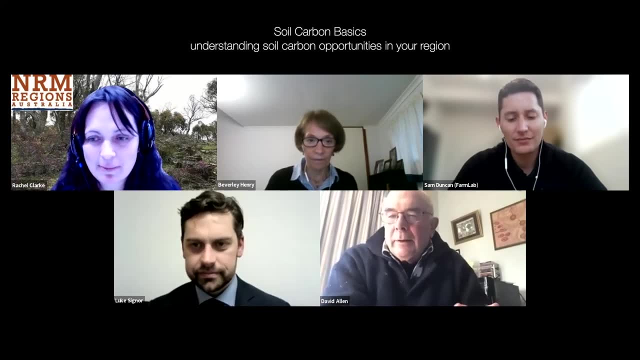 David's property is also a McDonald's flagship farm, which you might tell us a little bit about, the only one in Australia. So welcome, David, and thanks so much for joining us today to talk about your experience- farmer experience- of undertaking a soil carbon farming project. 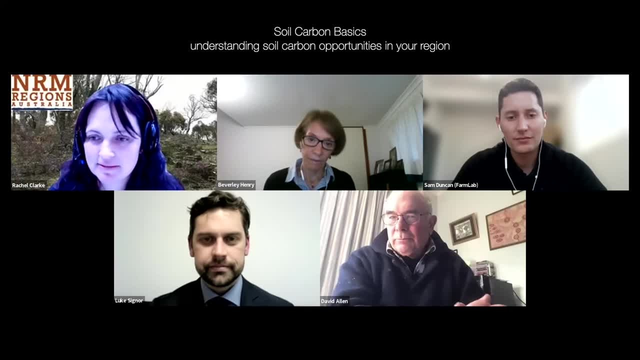 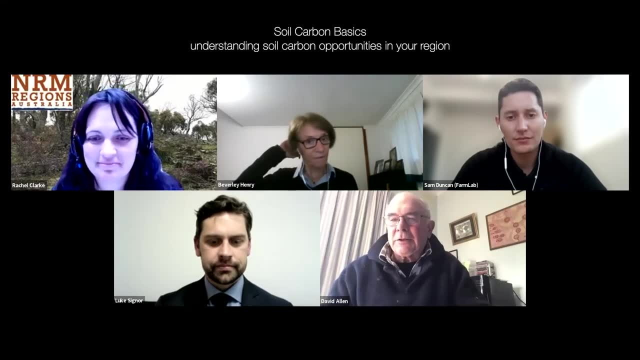 Thank you, Rachel. Can you hear me okay? Perfect, The internet has been a bit wafty today, so I hope it doesn't drop out, but I'll continue on anyway. So thanks for that introduction. We're on Japarong Country down here and just across the creek is Kiriburrung Country, So we certainly 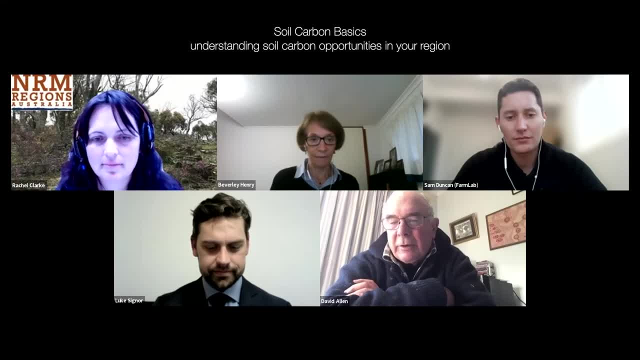 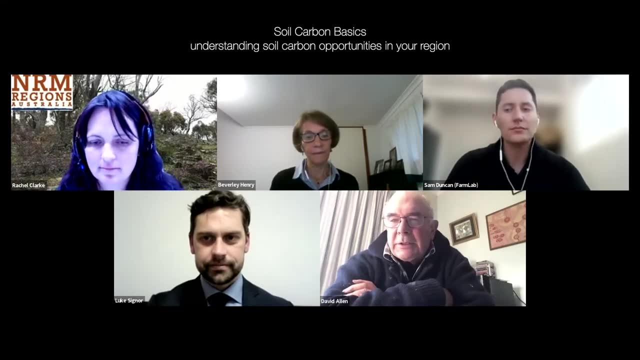 acknowledge all the past history of the Indigenous folk in this area. We've got a soil carbon project. We began that process in the year 2020, and it took basically nearly a year to find a project developer and build a case and then do all the. 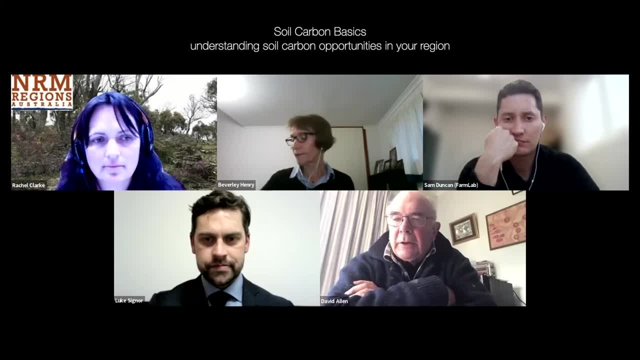 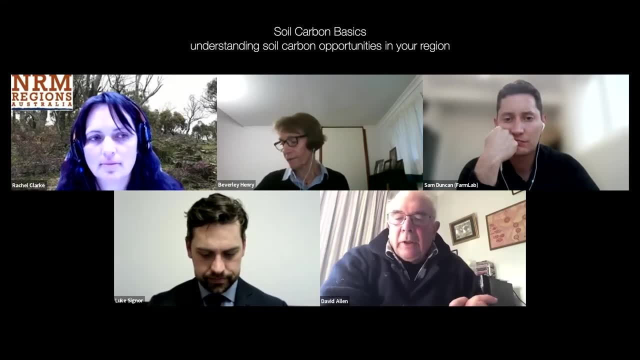 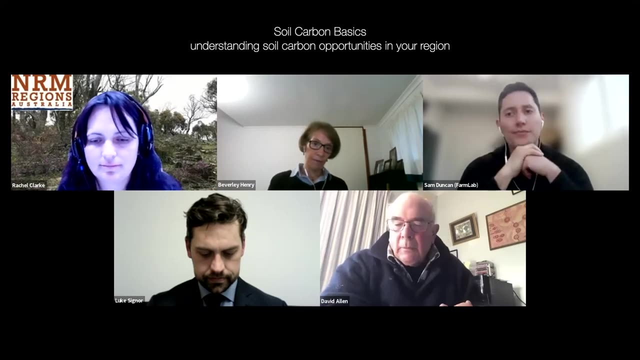 mapping and identifying the carbon estimation areas which the other speakers have touched on, And so then we were finally granted a project in February 2021. And then we could begin our do our baseline testing, which involved- so the carbon estimation areas is broken up into three- 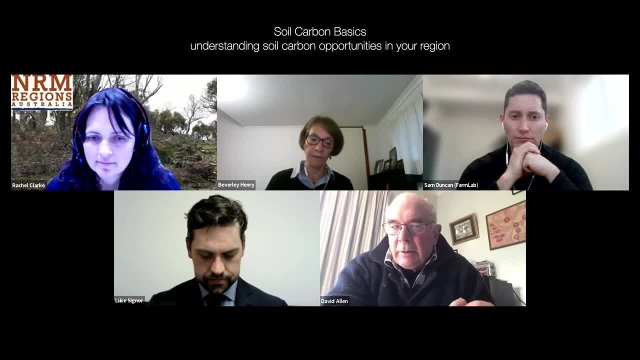 minimum of three strata And there's got to be three drilling sites, three core samples per strata and then the minimum of three per CA carbon estimation area. So there's nine minimum of nine holes per carbon estimation area And that's based on sort of soil type and land use and things over. that We've taken out. 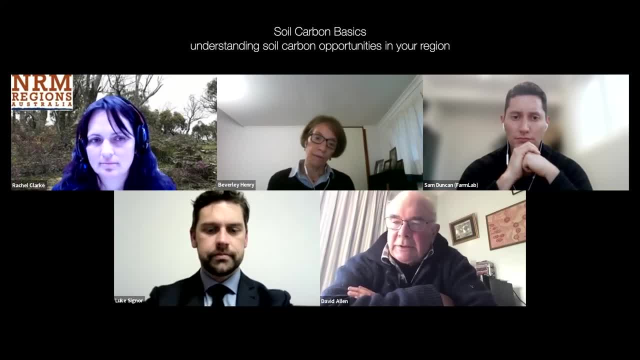 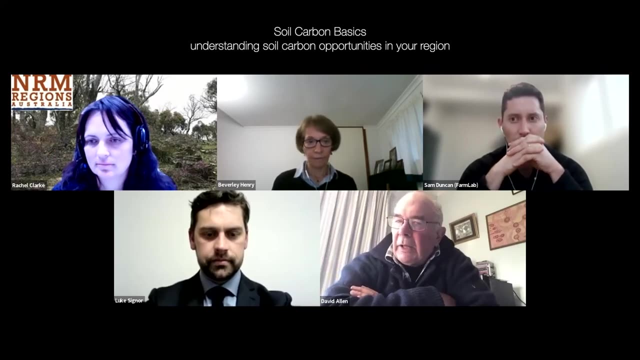 the gullies and the trees and the buildings and those types of things and you end up with a reasonable sort of of area that can be managed. basically so we've we've ended up with a bit over 100 core samples over our uh. we've actually got four sort of blocks of land that we've included in this uh, in this. 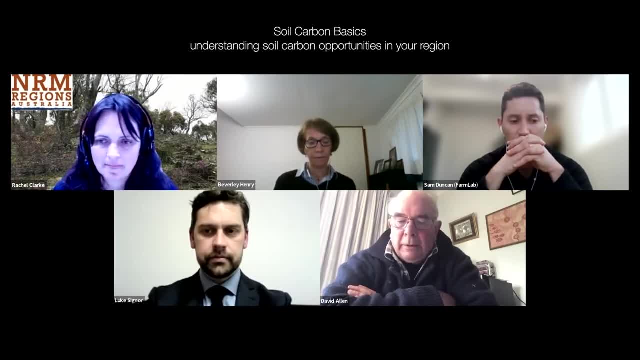 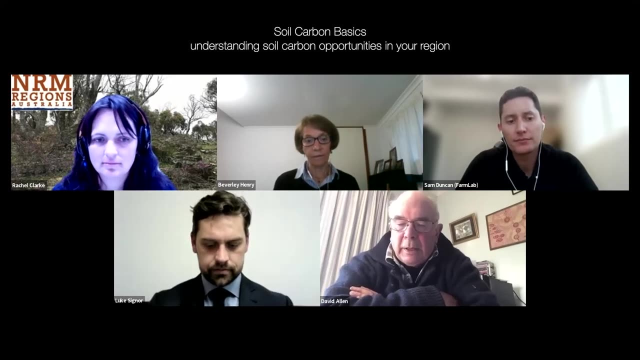 project um and the uh, and then it's also been sam, and luke mentioned the additionality aspect. so we've had to demonstrate that we are doing something over and above what we normally have done in the past as normal management, and in our case it's compost used. so using compost as a soil. 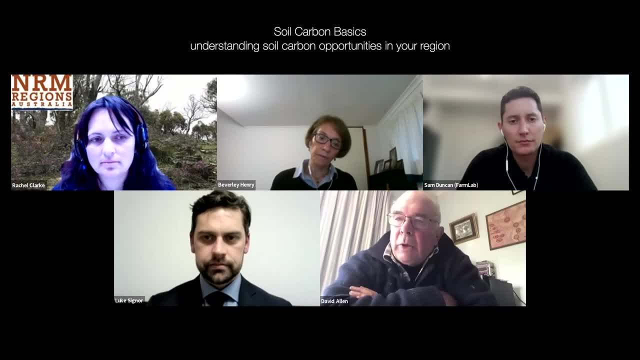 amendment. so we, we either make our own or we buy in a waste product from nearby. so that's our uh additional sort of management. and then the other aspect that luke certainly touched on was the, was the permeability of it. uh, for the, so it's a hundred years, basically, but they've, they brought it back. 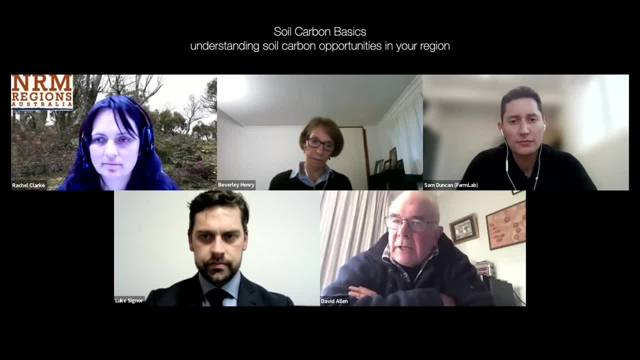 along with there being the water storage so they can make the compost that's been made already, the public housing of the other structure, and so, uh, and it's one of the things you know, this is going forward and if you're, if you're looking at the problem, if you're, if you're interested in. 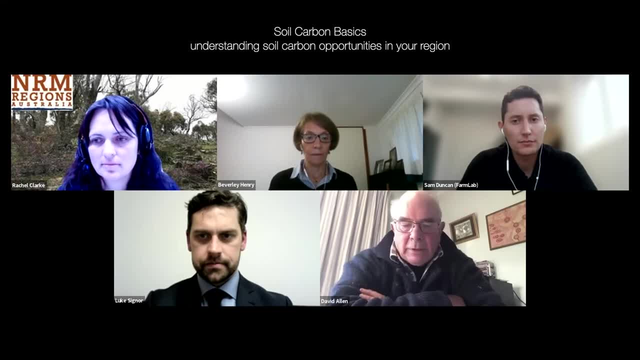 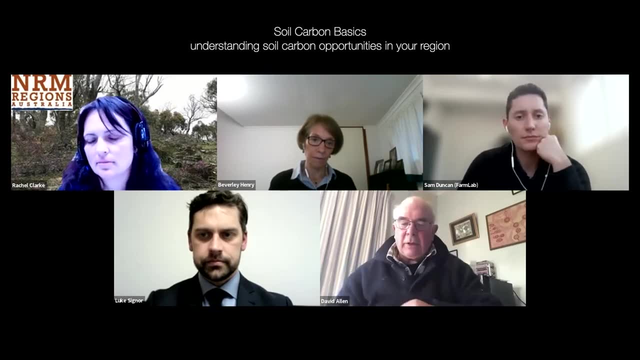 this problem, then feel free to jump right into it. what we're doing is we're using a different method. we're using a different method, which is you can do a third way, and it's: either you can do this without just having to be an initial water treatment program, and then you can just take up. 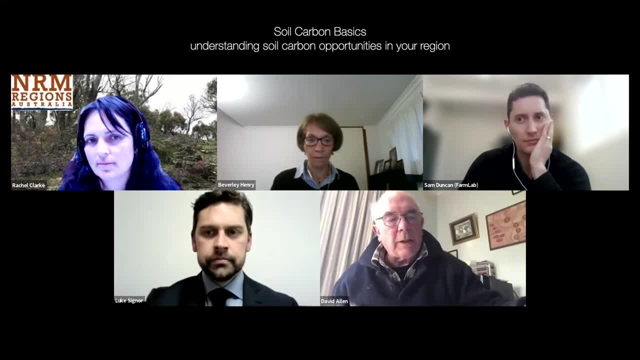 it over to a other program and then you can just take it over to another program and then you can. that's a sort of order. but we've got around the sort of the control of the English water and and, as Beverly sort of mentioned, the um, uh, the, the top, the top 30 percent is sort of 20. 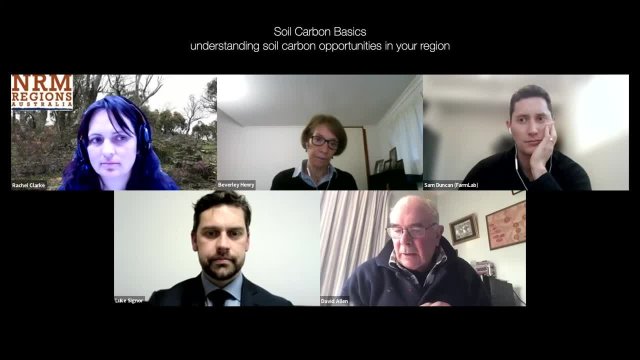 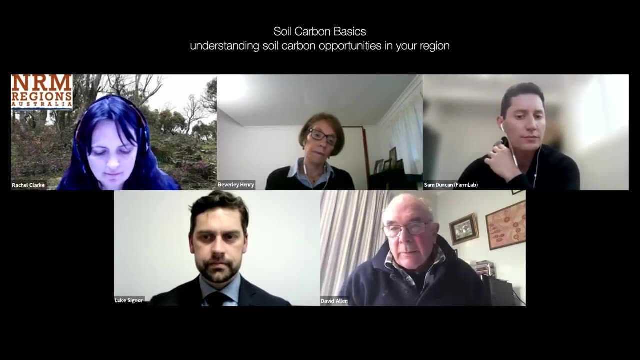 80 percent of the carbon and the underneath, the from 30 to 90, is sort of 20 percent of the carbon, the soil organic carbon, which sort of correlates with our results, because normally our soil tests, just for agricultural purposes, are sort of uh, zero to 10 centimeters and they're, they run at about. 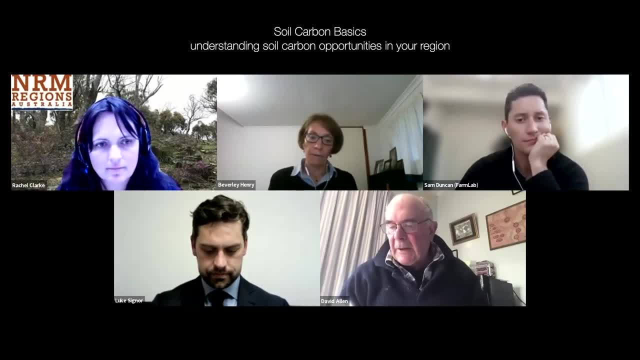 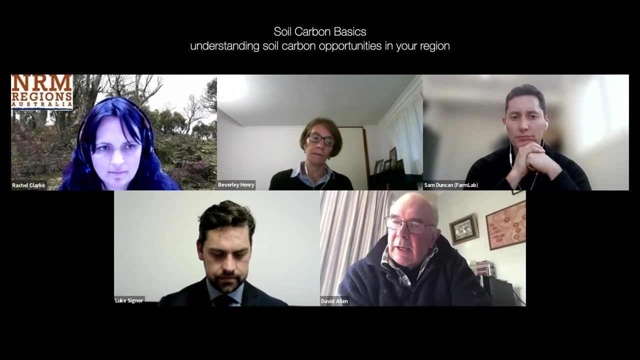 four, yeah, four and a half percent um carbon. but in this case, uh, with these tests, the zero to 30, uh, the, the results- because it's deeper- have spread that uh measurement down from sort of 1.3 to 1.8 percent and then 30 to 90, the it drops down to sort of 0.5 to 0.8 percent. so, in terms of tons, 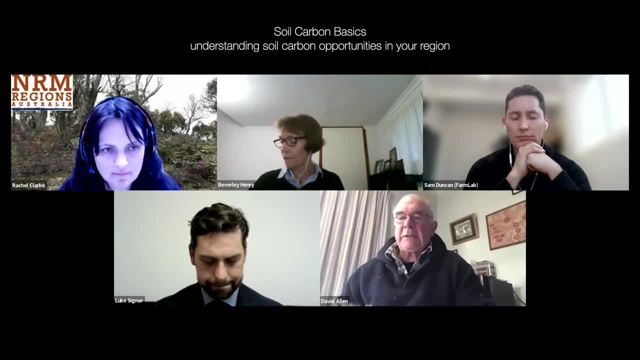 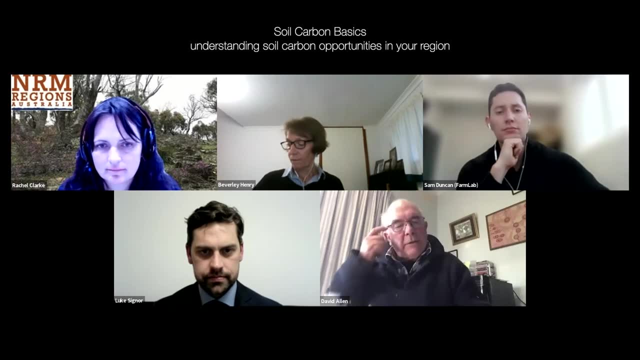 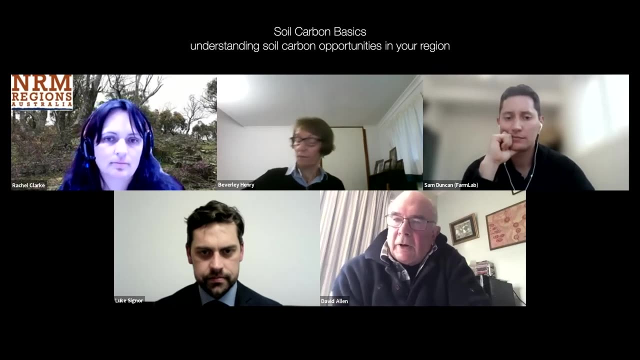 that we've identified and have got um. so then, as uh, as has also been mentioned, um by Luke and Sam, the five years um before five years is up, we've got to do, uh, another, do our second test, so that that'll be coming up in a in a year or so. um, we've got our project developers who are working with us. 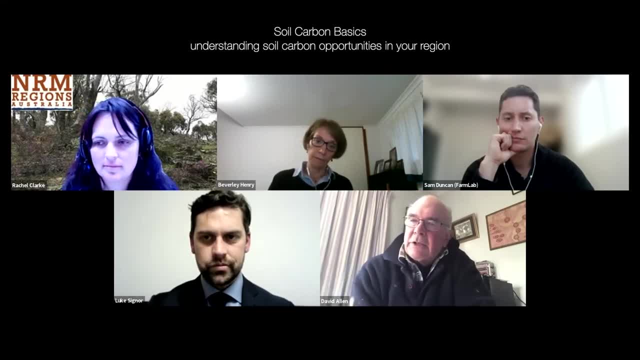 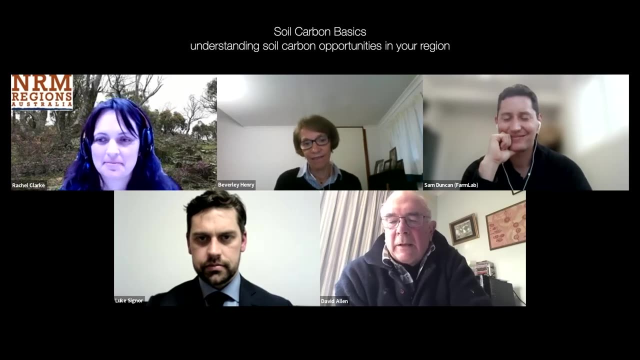 to do a test site this uh, this year, um, uh, a bit later in the year, or we might get Sam and use this technology that'll be. that'll be pretty nifty uh to see how we're traveling in terms of how much carbon we've got, um and as, as the baseline samples were all, uh, all tested and and yeah, the samples 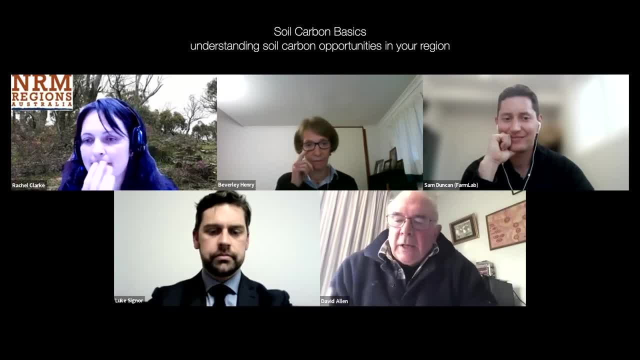 were sent away and all properly assessed and measured and and all audited, and then we've got the same we'll apply with the next test as well. they'll all be audited and um, uh, and ticked off. and then uh, yeah, having done our second uh testing, soil testing- we'll, um, we'll then, uh, send the report. 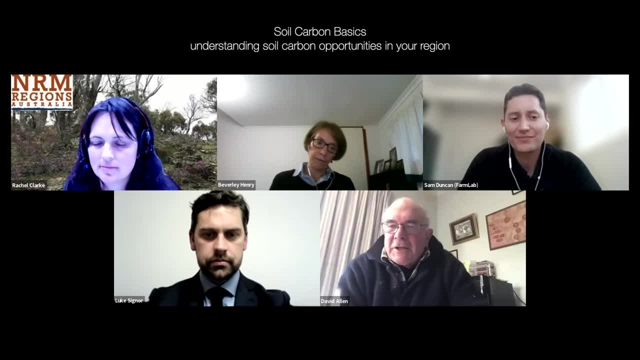 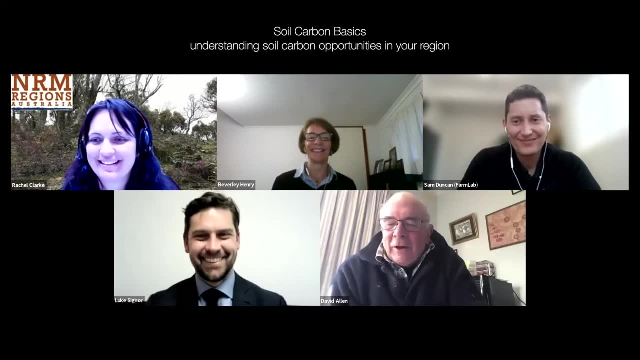 off to the clean energy regulator and hope Luke's still there and hopefully he can tick us off, um, if we make friends, if we stay friends with Luke, um, so no, I'm sure it's a bit more complicated than that. uh, so it is it. you know it is fairly prolonged, it's it's a long, it's a big. 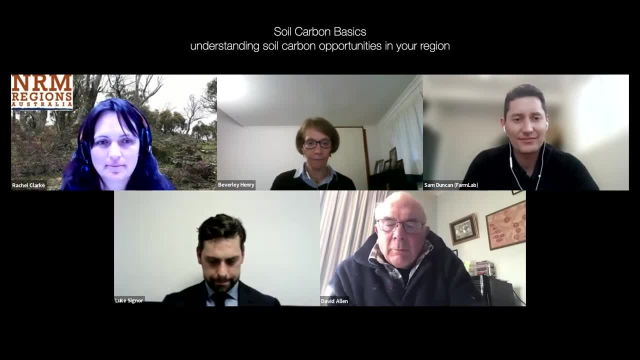 process. it's an expensive process and by uh continuing our like just putting compost out is not cheap, either sort of thing. so that's uh, yeah, this process of hoping to build soil, organic carbon, uh is not not uh, uh not exactly cheap. it's not easy, but what we have going for us. 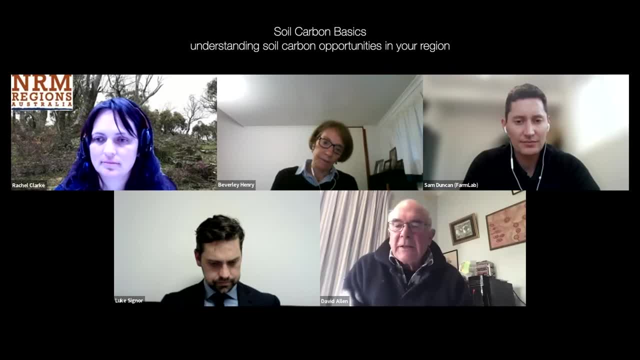 down in this part of the world that Beverly mentioned is, uh, high rainfall. we're 600 mils plus and we've got a lot of clay soil, so that that certainly helps um helps our process, and we've also used a fair bit of rotational grazing. we've got plenty of grasses, so we're fairly confident. 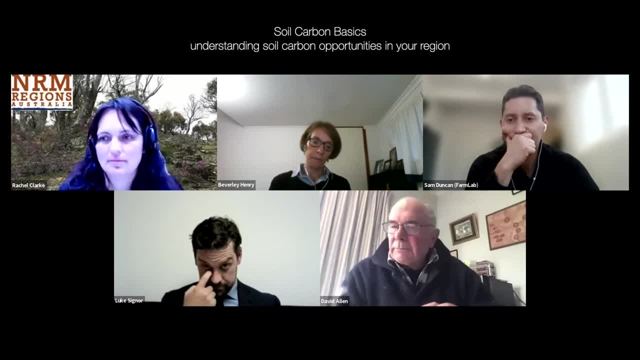 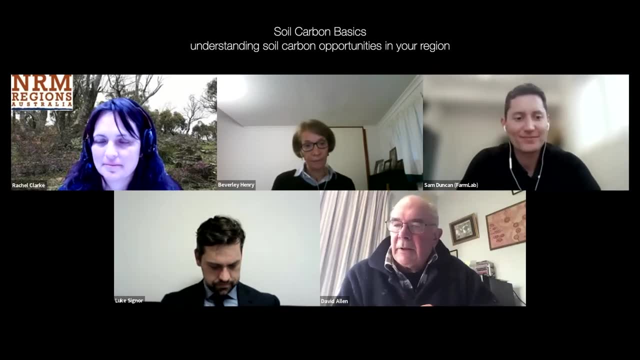 that we can, um, we can build, um, build a bit of soil organic carbon, um, and so that's sort of about all of the- uh, our farmers sort of story of a soil carbon project. thanks so much, David, and um, yeah, wonderful to hear about your journey so far and really good luck with building those soil carbon. 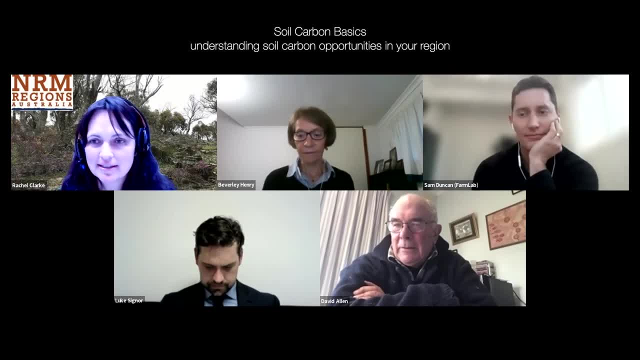 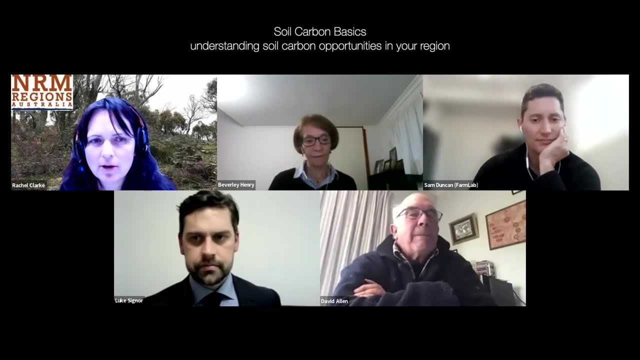 levels. um. so thanks to all our speakers for your really excellent presentations. I'm really excited to get into some of the questions now. so the first question I've got, which I'll- um, I'll go to Beverly first, but, um, Sam might want to jump in on it as well. um. so what are the specific management? 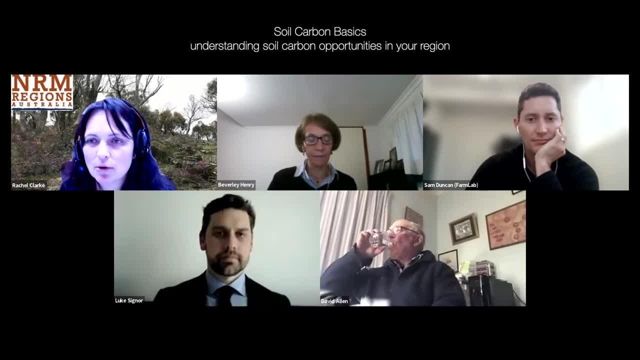 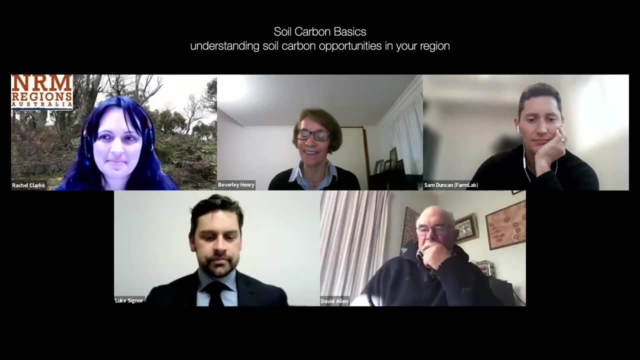 techniques to build stable organic carbon deeper into the soil profile, Beverly, if you'd like to have the first crack at that one. thanks, Rachel, and thanks for the question. it's a. it's a really important question, actually, and not an easy one to answer. um, so the amount of soil organic carbon that you can build depends a. 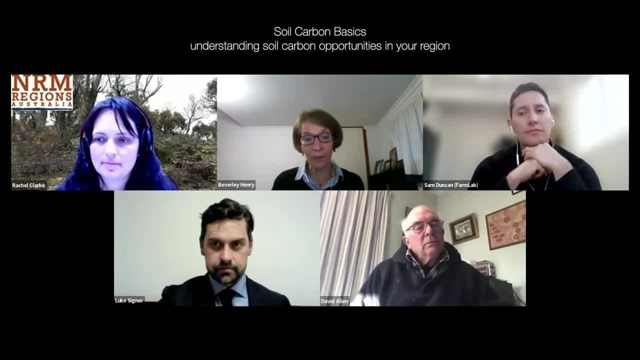 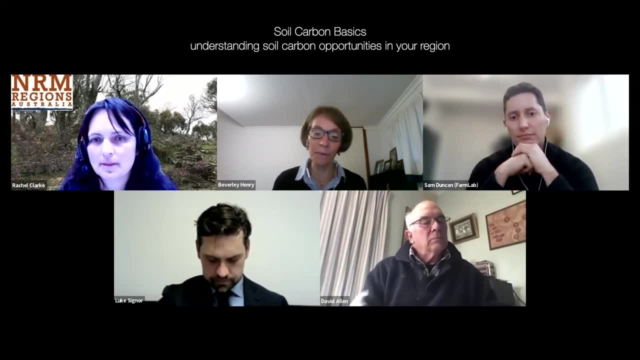 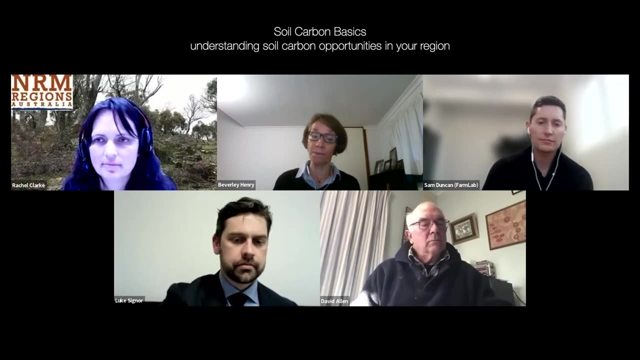 bit on- uh, what's there already? and your past management, as well as the climate and soil factors that I mentioned earlier, and so one of the highest rates of gain in soil carbon that occur is when you start with a soil that's a that's run down. where you have a low initial starting point and you can build soil carbon. so you may remember from the graph I showed that it will increase fairly quickly there. um, so the balance between inputs and outputs is what we think about, and you need more inputs than the losses and you get that by. 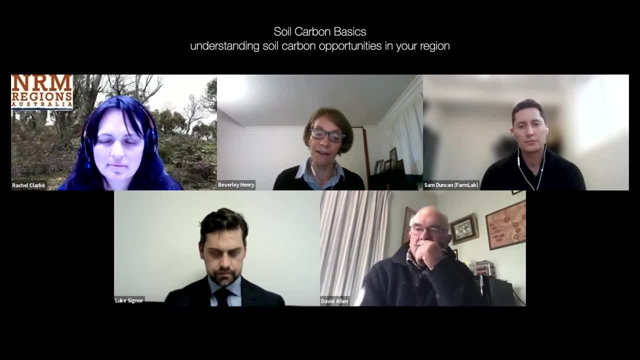 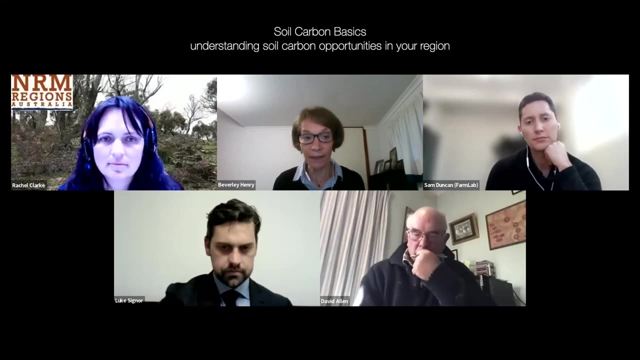 using ground cover. so one of the you know either a cropping or a grazing situation. you want to make sure that there is minimal periods where the bare soil is exposed to the atmosphere and the bugs are free to um break down the carbon and it's lost again to the atmosphere, um, so that's, that's one. 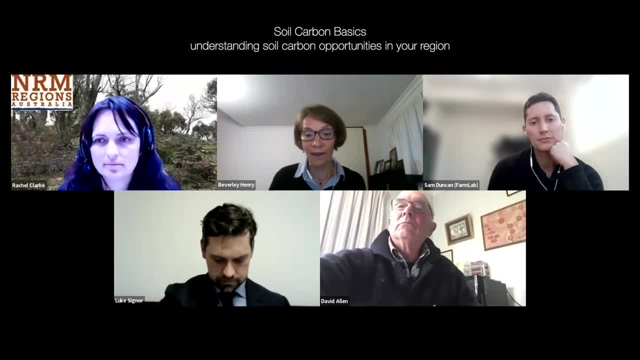 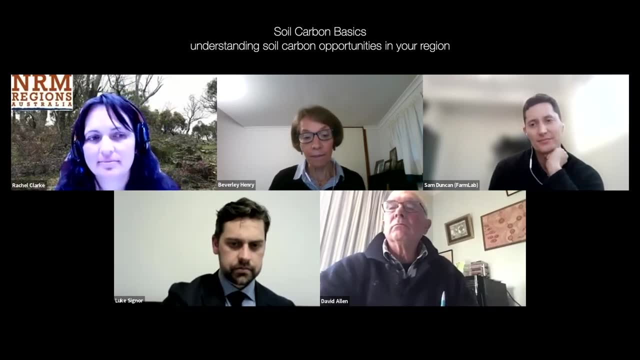 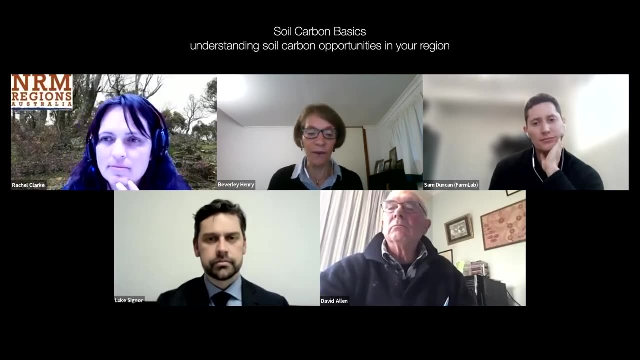 of the points. um. another point I'll make, uh, and I will give Sam a turn as well- um is that one of the um limitations on being able to build soil carbon is the availability of nitrogen. so I don't know, it wasn't very obvious and I didn't have time to to really 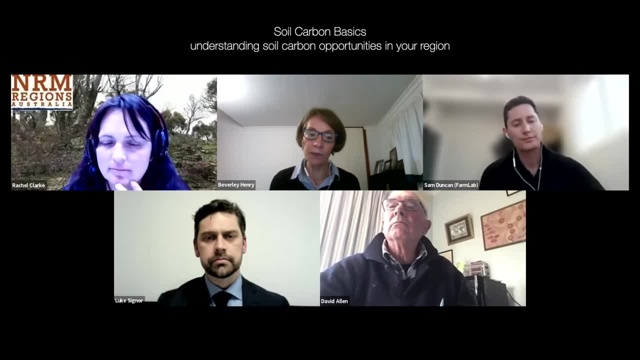 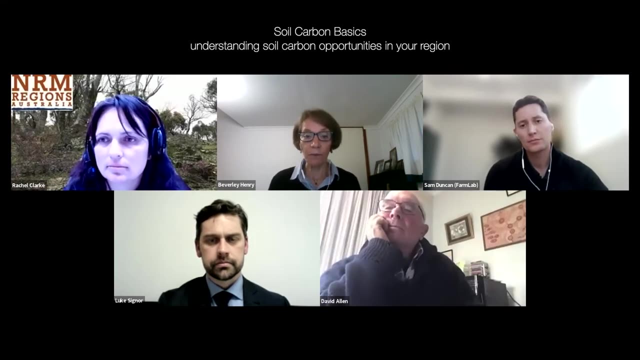 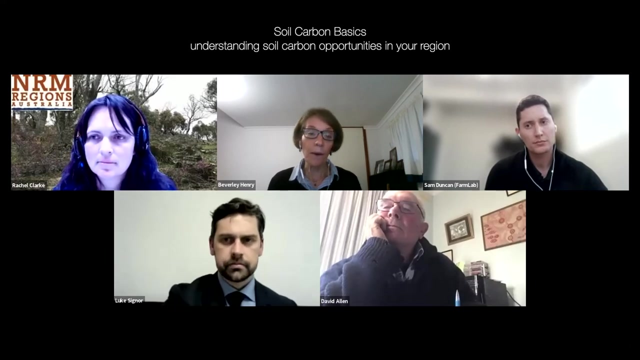 talk about it much, but um stable soil carbon has a higher nitrogen to carbon ratio than um fresh biomass. you need nitrogen in the soil, so using legumes in a pasture mix or in a plantation for crops is a really good way to to build soil carbon. so, um you know, apart from that, 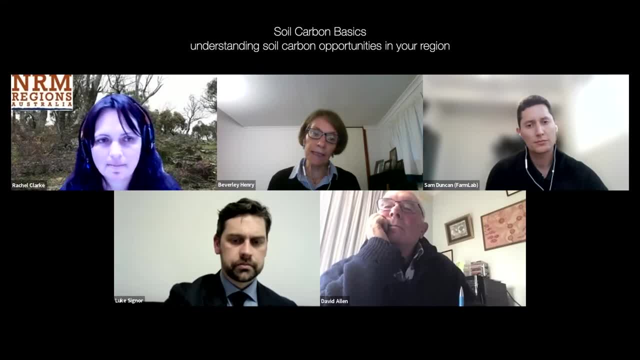 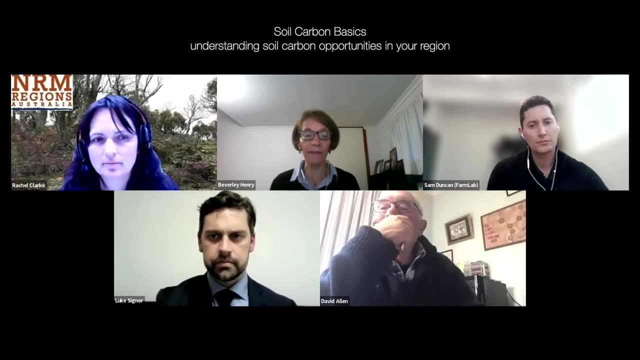 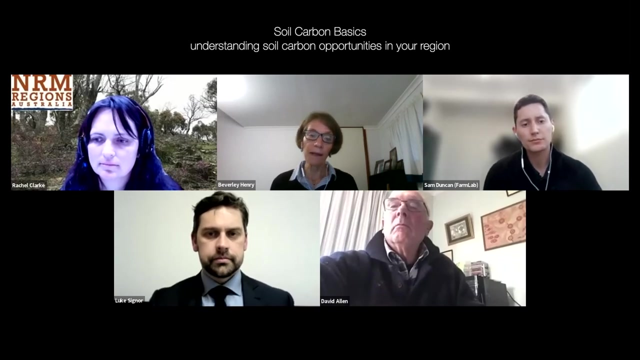 it's. it's just um, I suppose maintaining the, the soil structure as much as you can within the limitations that our variable climate throws upon us every now and then, um, and and ensuring that there is um, that healthy production there and nitrogen is, is an important part of that. so I'll hand over Sam um and you know I can come back. 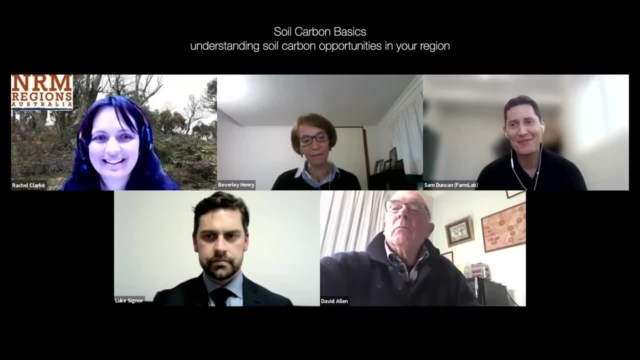 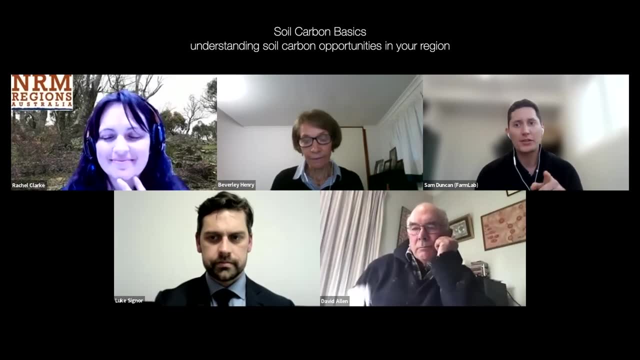 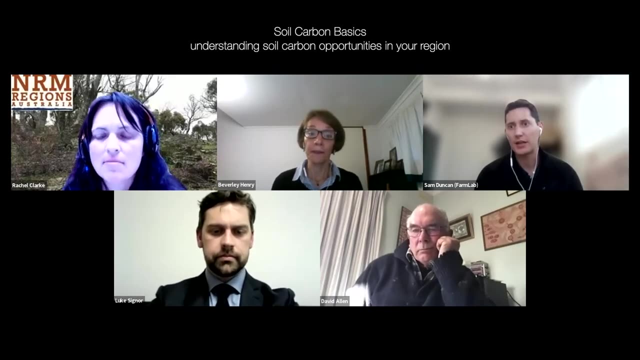 here, if needed. thanks, I don't think I have much to add. um, look, I, I think, from our perspective. I mean, the only thing I have to add is: um, uh, and I would like maybe to throw across to David, because, David, you're doing this as well, but um, soil across the landscape is not homogenous. you, you don't have. 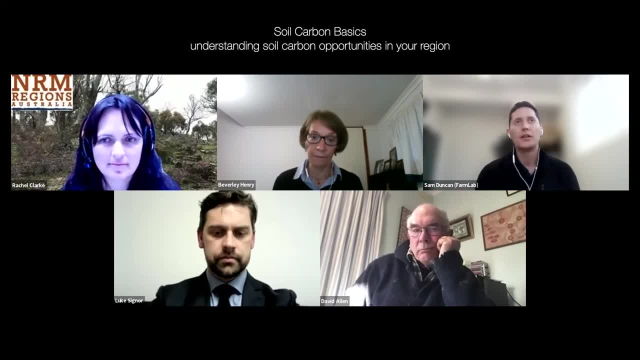 the same soil type, generally speaking, across across your farm, right? so in that, in that sense, um, courses for courses, do what's going to work for you- different soil types- and understand that and map your soil and use something like that, or we don't care if you don't. 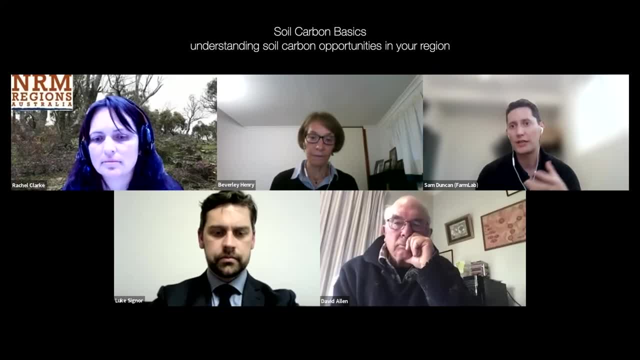 use some, but certainly map your soil and then you'll you'll have a good idea as to you know, you know what works where. take a few soil tests, understand where the weaknesses are across the property and where the improvement can be made. um, and yeah, David, I might kick across to you because 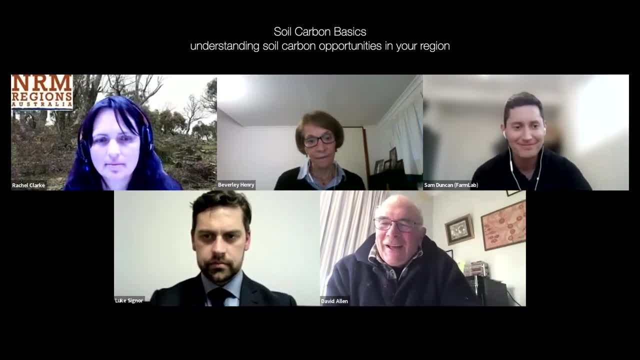 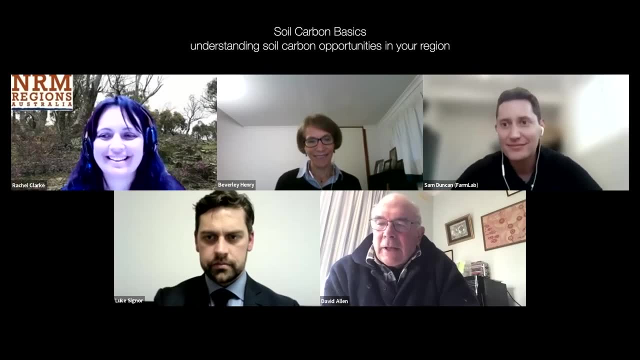 you're going to increase carbon where? thanks Sam. yeah, good question. um, look, I've. I should have also mentioned dung beetles. I just love dung beetles. they're amazing fruiters so they can really transport nutrients deep into the soil- 60 odd centimeters down into the soil, but primarily 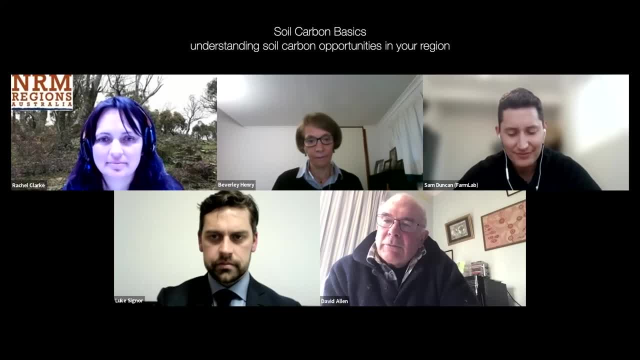 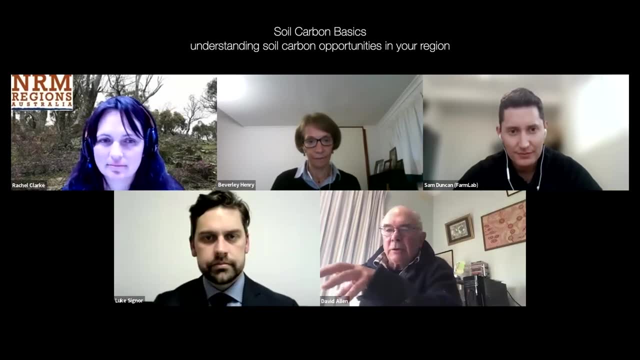 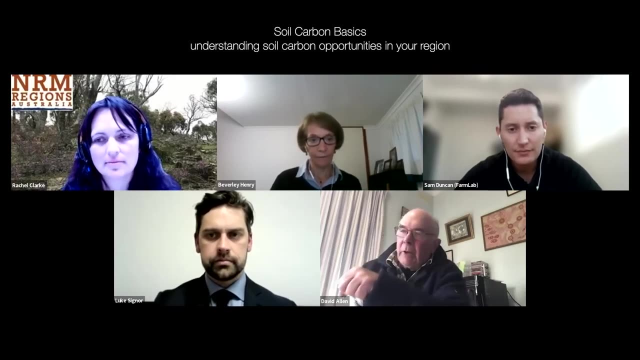 it's rotational grazing and perennial grasses where there's a root, uh that yeah, the idea is to get the root down as far as you can, um, so what's on top of the ground is also what's below, and when it trumps the top third of the grass off, uh, the bottom third of the roots die, they senesce and then 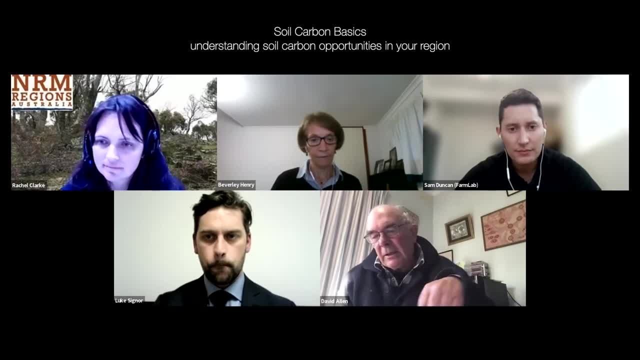 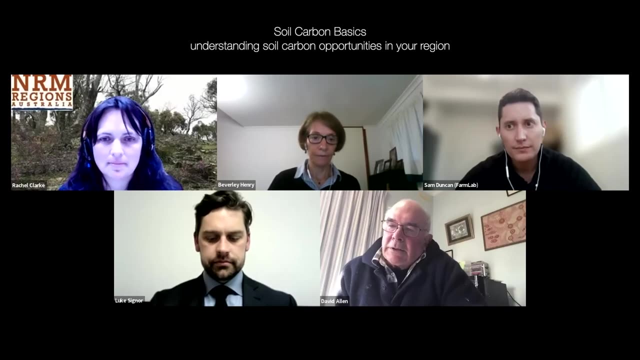 you can move the cattle on to the next paddock and the next cell and the grass will grow depending on the time of year, and the roots will grow and so that cycle of sort of uh eating the top and and then moving them on uh really encourages the the, the plants to grow but also the roots to grow and 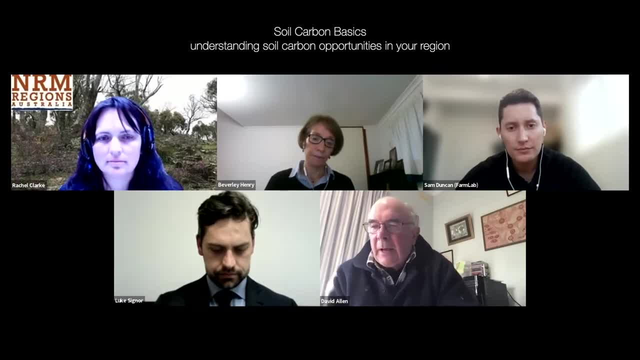 the root. when that the roots die, that is just sort of basic carbon locked up in the soil and the deeper you can go, the better, and, um, particularly, you know, below 30 centimeters. so you know that rotational grazing process, uh, with perennial grasses is- is one of our main main, um, main things to use, I think, and not 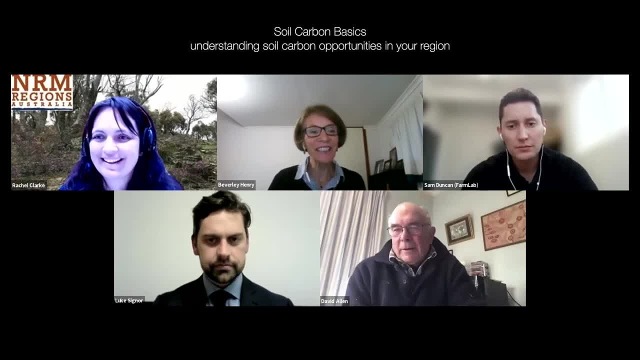 forgetting the dung beetles, Rachel, if I could just add um to- and I I really appreciate David's insights there. that's excellent. um that there are a number of studies that show using diversity of plants is also useful. yeah, yeah, wonderful. and dung beetles, so yeah, really good, call out for the dung beetle there. 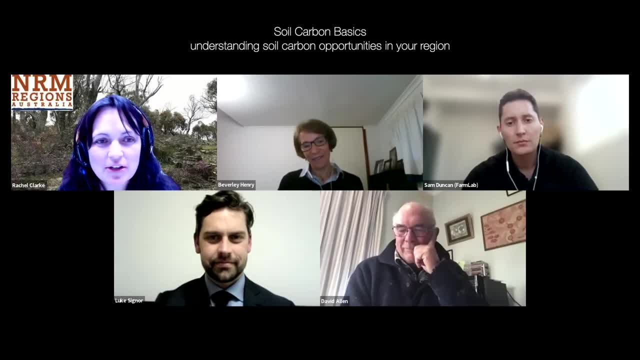 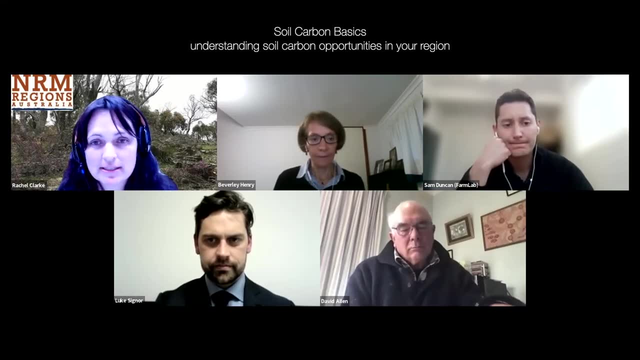 thanks for that, David. um, the next question I'm going to go to is from Susan Sweeney. so Susan's asking: Sam, do your calculations? Sam? mean the farmer can be carbon neutral as well as sell carbon credits, and this is a pretty important question. I think it is really good question. 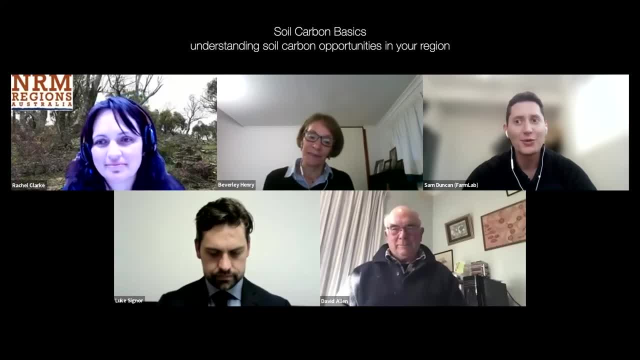 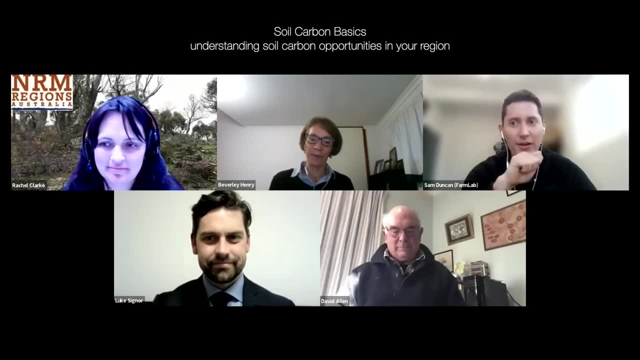 um, I had a look at this earlier in the chat. um, because, because Luke, Luke, I'll, I'll stab Luke in a second, because he had some three really good graphs, which exchange went this really well, right? so so the answer is yes, you could, you could, but you wouldn't be selling all the carbon offsets. 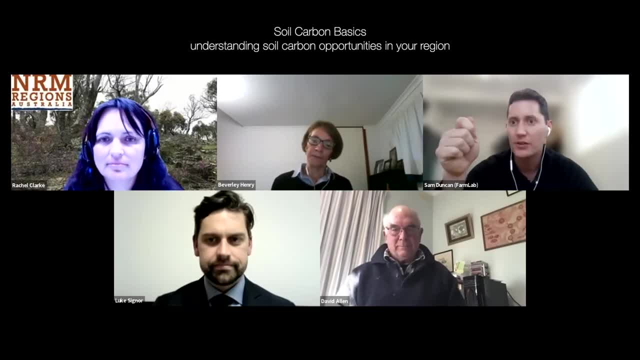 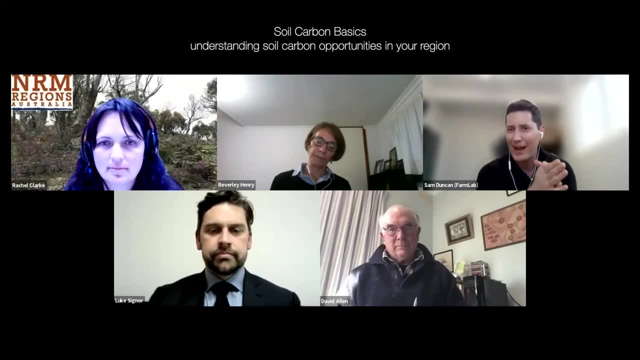 to the regulator, um, or to to an international buyer, right? so so what? what? the amount of carbon offsets that you build is based on the change in your baseline of emission. so we look back: is it years, luke, five or ten years? what is it now? five years, five great yep. so you look back five years. 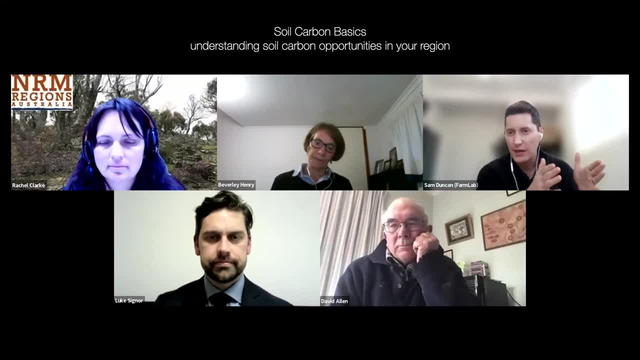 and look at your emissions over the last five years before you entered that project. so a thousand tons of emissions across your farm and then, if you're in three years time, if your emissions have gone up to 1100 and your carbon sequestered is 2000 tons, you don't subtract the full 1100 tons. 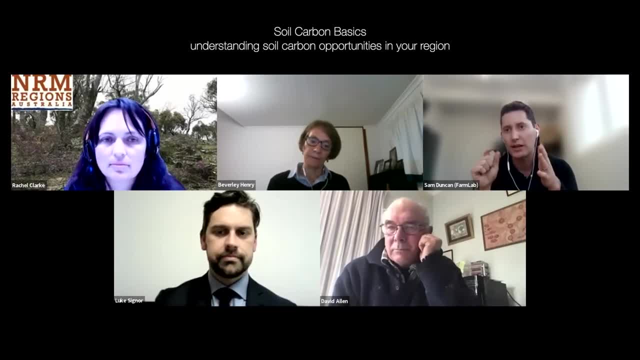 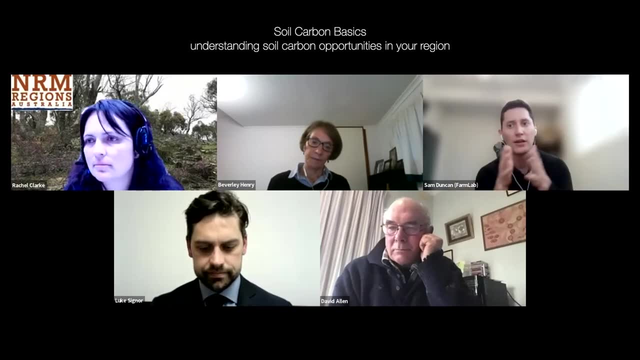 of emissions. you only subtract 100, right, because you're doing something slightly different and you have to remove that slight difference. so we work on human reduced. you know climate change factors here, so it's only it's. we're only trying to encourage a change, um all things remaining the. 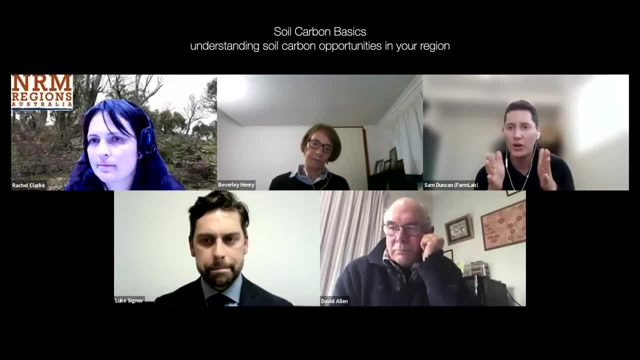 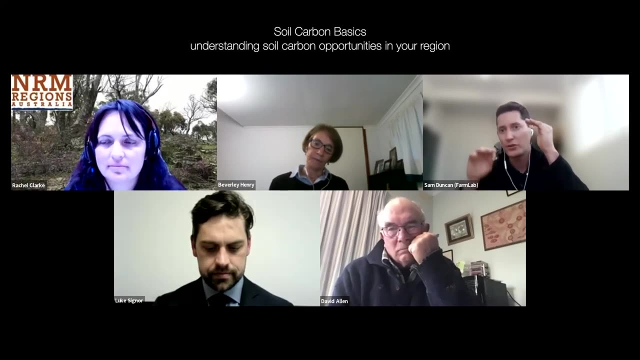 same, including your on-time emissions and your business emissions. right so? so what you would have to do in that case is, rather than selling the 900 credits um- which is what, what you're sorry um- 1900 credits to the on the on the ibu market, you take the full 1100 credits out of the equation. 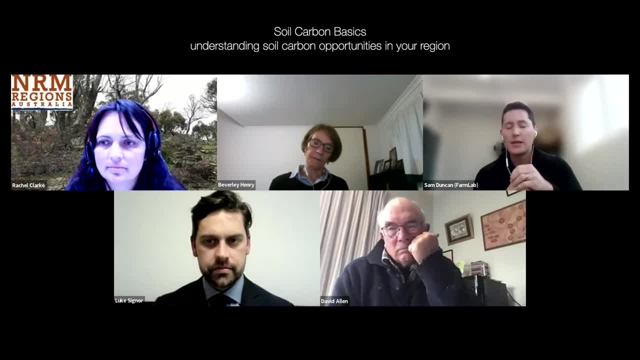 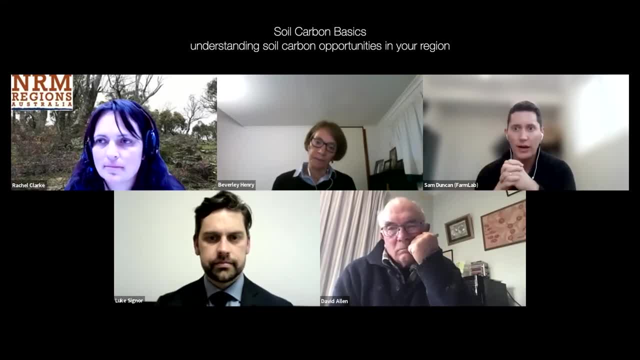 we calculate carbon across grazing operations. you know, I don't know. you know, a thousand hectare grazing operation, 300 head of cattle might have 30,000 tons of emissions, but you might be sequestering a hundred thousand tons of carbon. 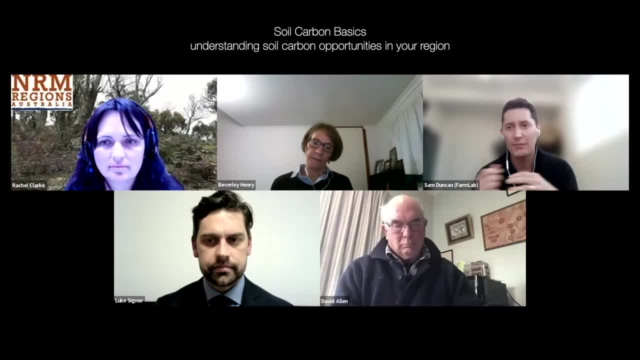 And so it's kind of that 30% range carbon- carbon sequestered versus carbon emitted- based sort of we don't have enough data yet and it's building right, So don't take, don't take that at sort of direct face value. 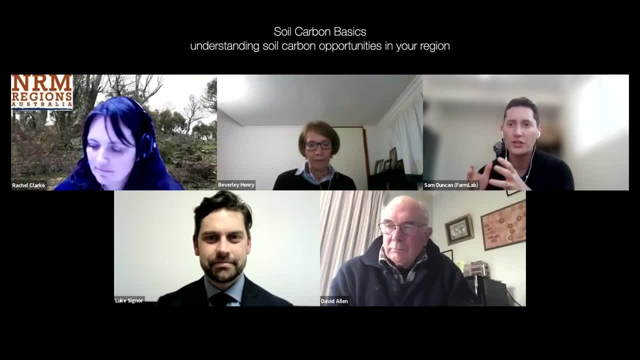 but certainly the amount of carbon you emit is usually, generally speaking, significantly lower that you should. you can actually do this. It just takes away from the outcome and you kind of you don't know, you really don't know, until you know that year three, four, five, 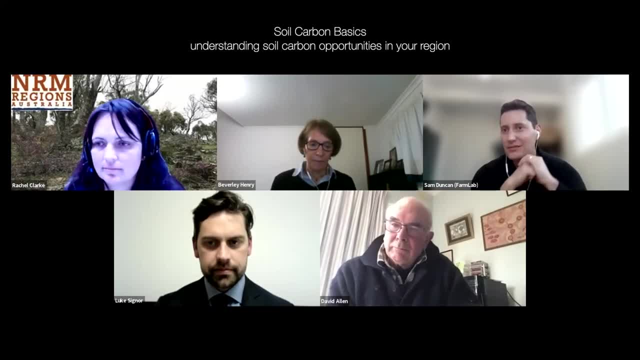 when you actually sequester that. Luke, have you got anything to add to that there? on the baseline front, Are you seeing the baselines go up? I mean, I'm keen to know in general: do people usually have a baseline increase there from their baseline when? 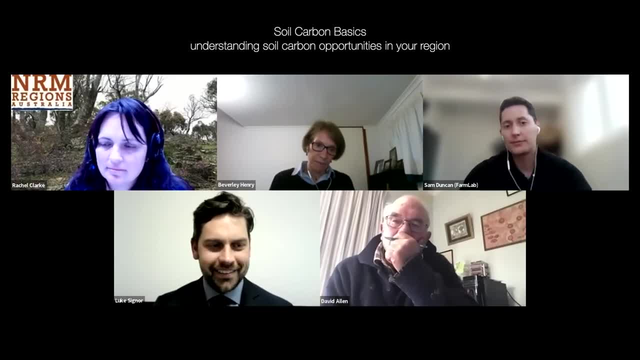 they're sequestering carbon for these projects. You know it's a- it depends. The first thing I just want to jump in on is that if your five-year average is a thousand and it goes down from the implementation of the new activity to 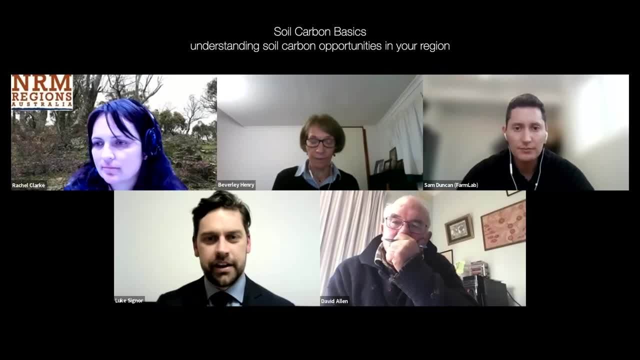 800, you don't get credited for that buffer of 200 either. This method in particular only credits the sequestration that's measured in the soil And if you're finding gains in the abatement of the emissions that are being avoided from doing your activity. 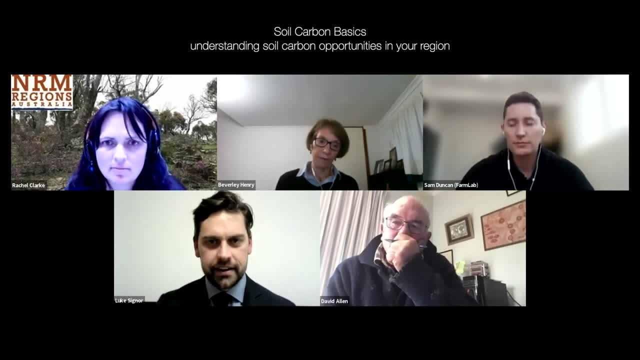 you're not currently. you're not currently credited for that, So it's only the increase is a negative, but any decreases unfortunately still just negated as a zero. As far as what am I seeing? Not a great deal. There was a bit of a problem with the 2018 method. 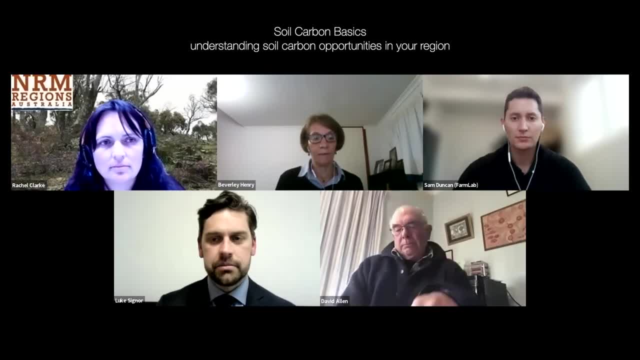 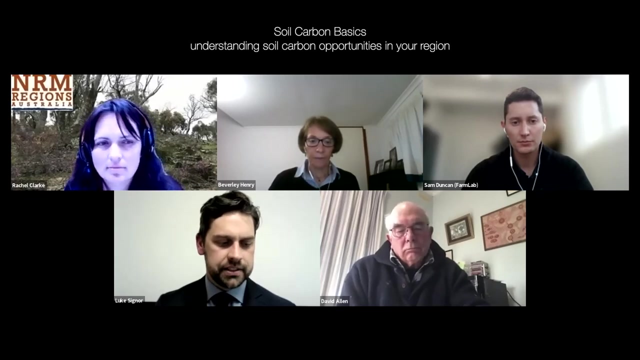 which means that there's been some delays to information being filtered through to the CER. at the moment, A lot of projects- or all projects who are on 2018, will need to move across the 2021 to calculate their abatement, And I did see a question about timing and a function of the project is that. you can change your start date by 18 months from when it was declared. So realistically, we could see close to about eight or nine years before a project is registered and carbon credits are issued. So you know, my expectation is that CER will see an influx of some of the older projects being reported soon. 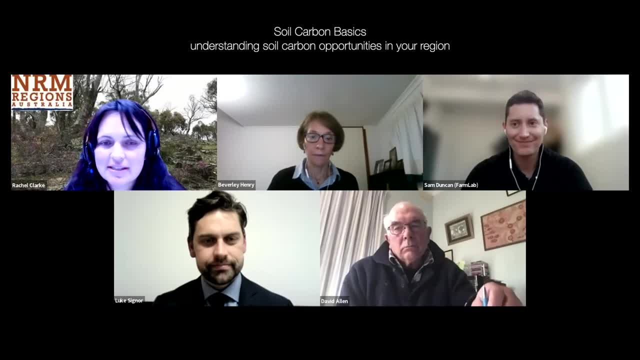 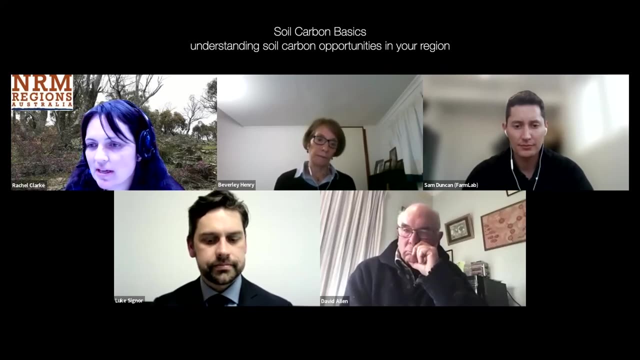 Thanks very much, Luke and Sam, for those answers. I've got another one just for you there, Luc, and un-muted. So this question about permanent. So how's the ERF considered long term storage and permanence for soil carbon beyond twenty-five years? 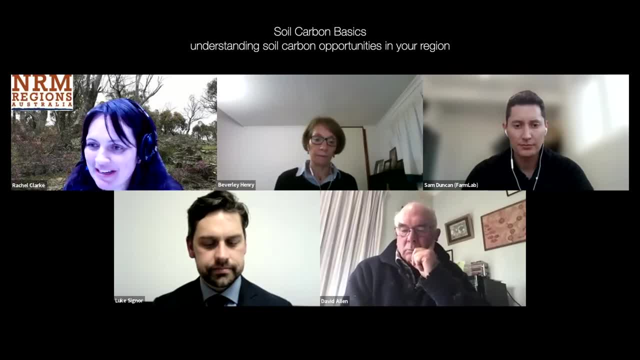 What happens at the end of a 25-year project? I know we probably haven't come up against any yet. I don't know. I don't think anyone knows. So how does the Пока Project consider long-term storage and permanence for soil carbon beyond 25 years? What happens at the end of a 25-year project? I know we probably haven't come up against any yet. 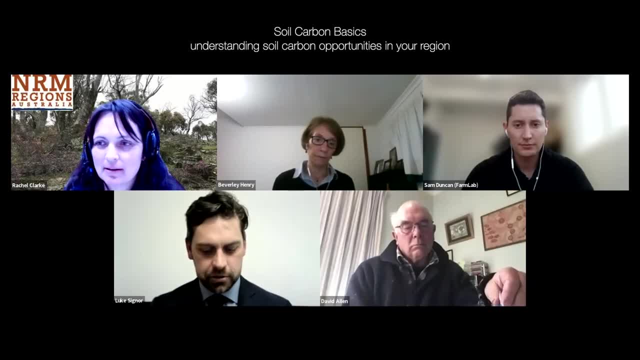 but what will happen to these projects? Yeah, it's a good question. So when I talk about a 25-year permanence obligation period, that is one option and that carries a 20% discount in the credits that you're issued. 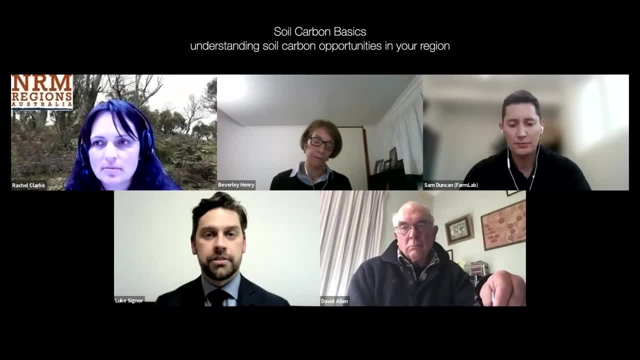 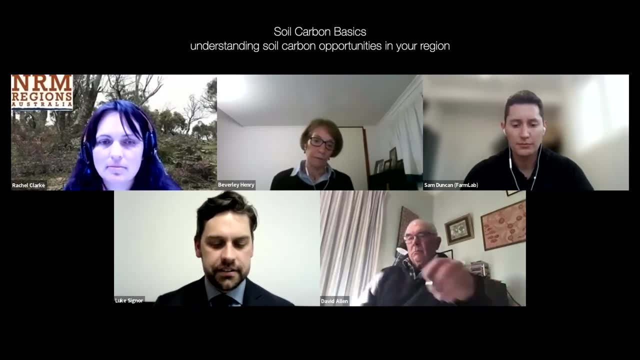 You can decide to have a 100-year permanence obligation period which doesn't carry a 20% penalty. The expectation is that the activities will continue for the entirety of the permanence obligation period and after that obligation period has ended, there is no further obligation to continue those activities. 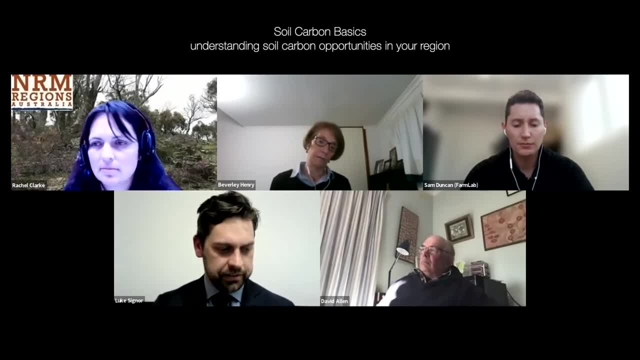 So I also briefly mentioned that there is a mechanism that, as method activities get to the end of the accrediting period, it's possible that there is a review of that method to see if the accrediting period would be extended. So that would need to be taken into consideration. 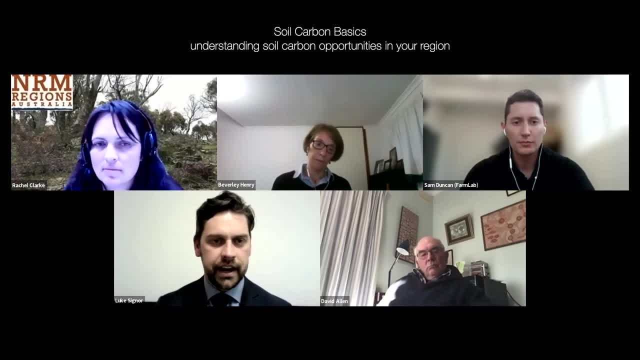 when those projects reach, So that 25-year accrediting period end at that time. Thanks, Luke, I didn't realise that you could have a soil carbon project for 100 years. I sort of thought that they were limited at 25 years. 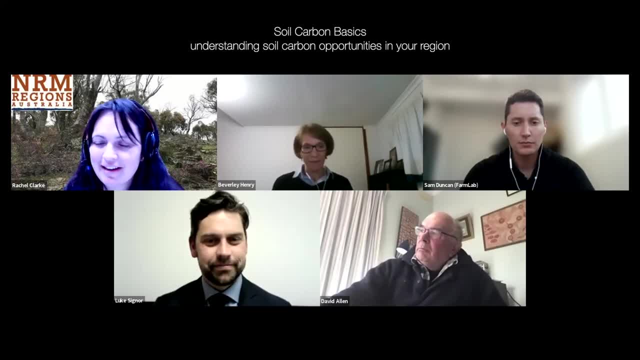 so that's really interesting. Did any of the other panellists have a comment on people's ability to sequester carbon in soil for 100 years? I think if you're around for long enough, give it a go. Still digging in the compost. 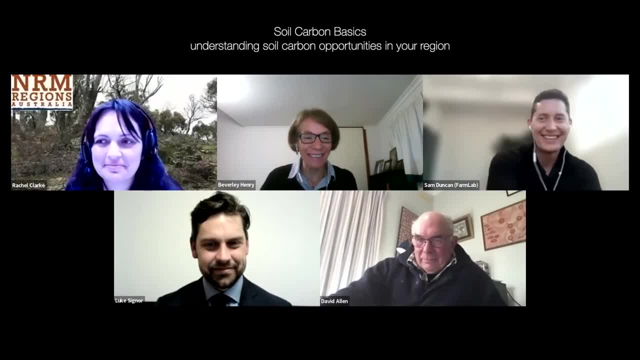 Luke, I just wanted to check with you before I Please correct me if this is wrong, but I just wanted to note that for the 100-year permanence period, all of the credits are still issued for the 25-year crediting period. 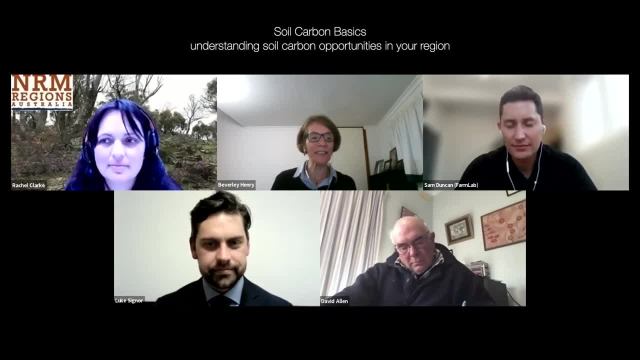 So the permanence period: you don't get any further credits for the rest of that 100-year period. You just haven't had the discount before, And that's something that I've found is confusing to some people, so I thought I'd just clarify it a little bit. 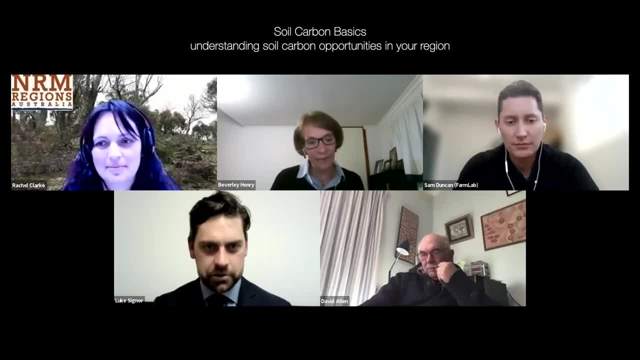 Yes, thanks Beverly. Yes, that's correct. So a sequestration project is a 25-year crediting period, so 25 years of credits being issued, and then you can either have a 25-year permanence obligation period or 100-year permanence period. 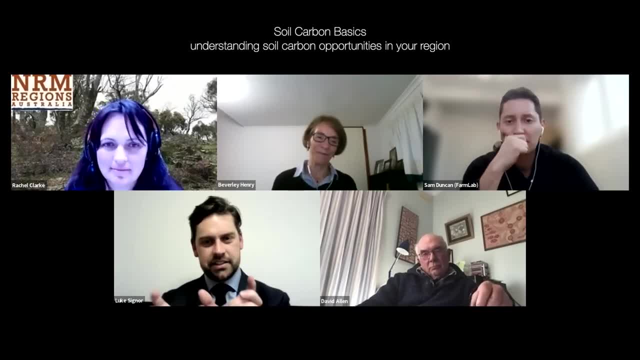 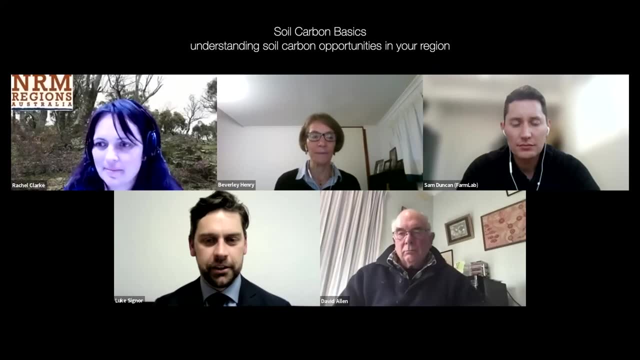 And that was what I was trying to show in that graph with the bars: that there's a slight lag in the length of that permanence period over the extended end of the crediting period alone. Thanks very much for clarifying that, Luke. 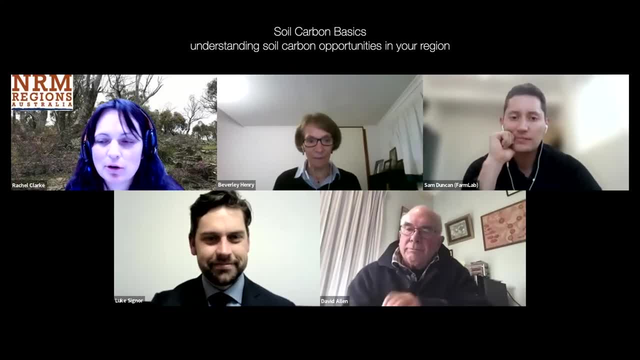 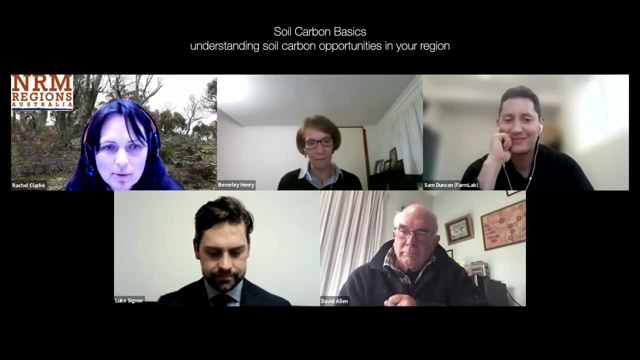 and also Beverly. It's good to know that people won't be willing carbon credits to the next generation as they go down. I'm going to go to David now. So, David, I'm just wondering, with your project and starting it out on your farm, 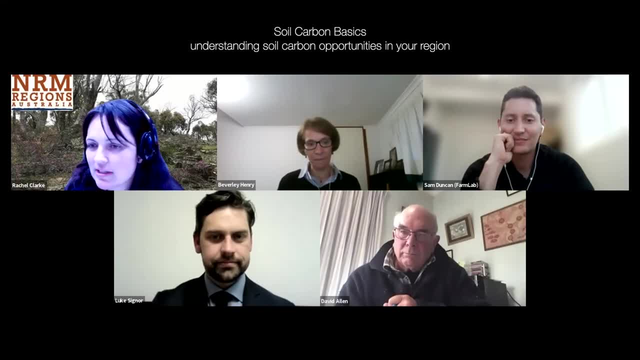 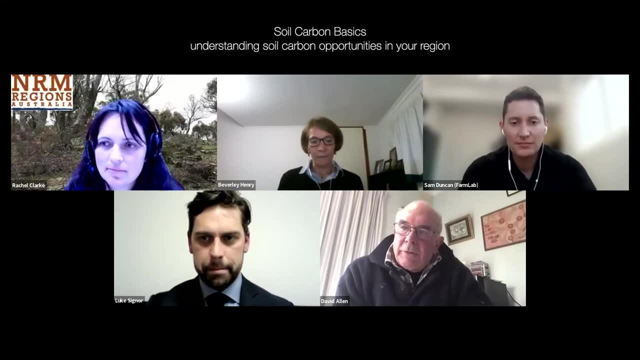 would you recommend other farmers get involved in soil carbon projects, and what sort of things should they be considering? Yeah, look, I think it's good because basically all we're doing is building soil organic matter. You know, the name of the game is to build soil organic matter. 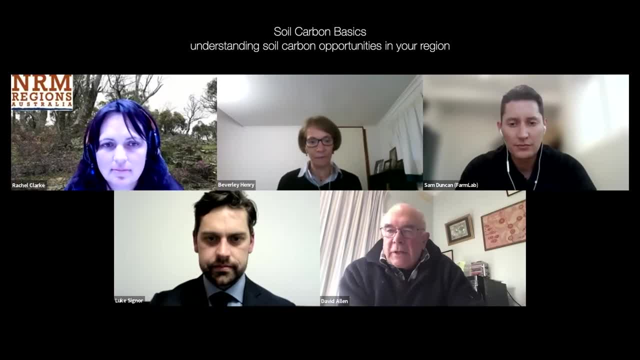 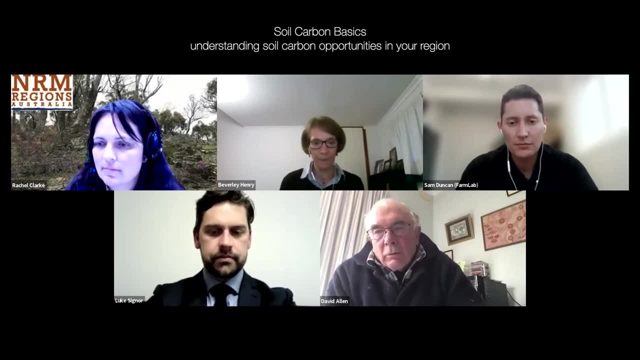 Which is good, It can only be good. It's like a good veggie garden. you know, If you're putting your soil, organic matter, building that up, you've got more water holding capacity, more resilience, et cetera, et cetera. 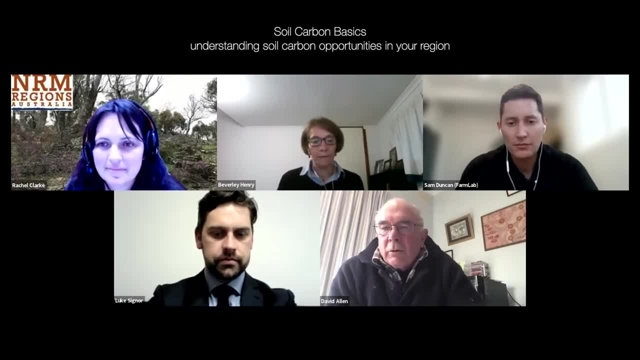 There's grass growth, you know, and then therefore, more beef cattle. So we're coming from it from the angle of building up our soil organic matter and just trying to create better soil, And then, you know, we're going to start to build more organic matter. 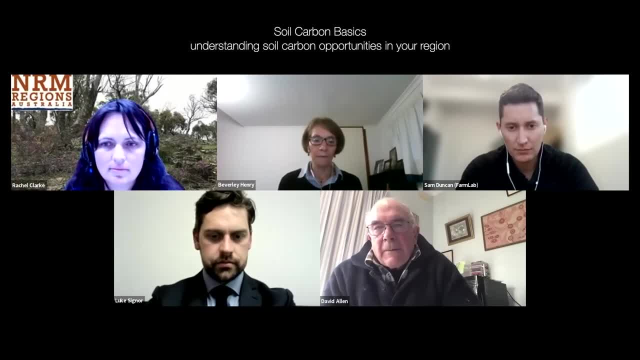 and then you know we're going to start to build more organic matter, and then you know we're going to start to build more organic matter and microbes, et cetera. If there's a trade-off with carbon down the track, it would be good. 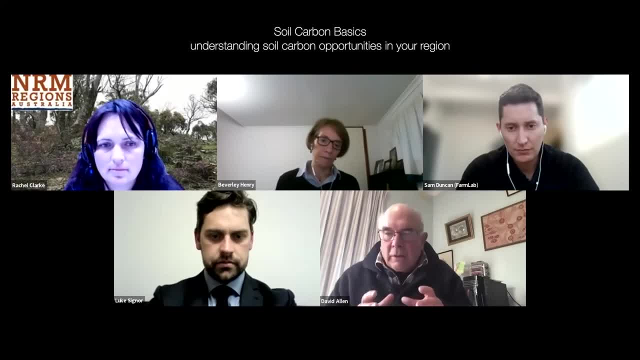 It would be a pity having to go on, having gone through all this work, not to get a benefit. So that's why we actually registered the project. So we're doing the compost and we're, you know, doing the best we can to improve our soil profile. 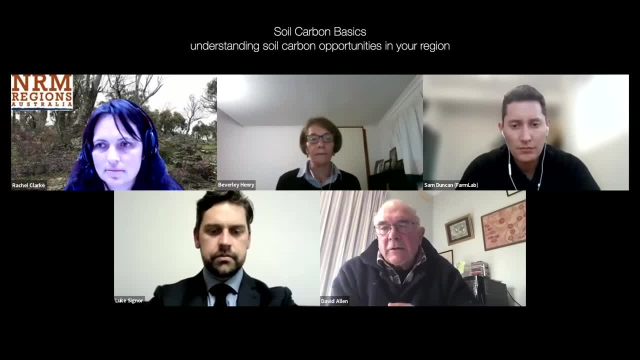 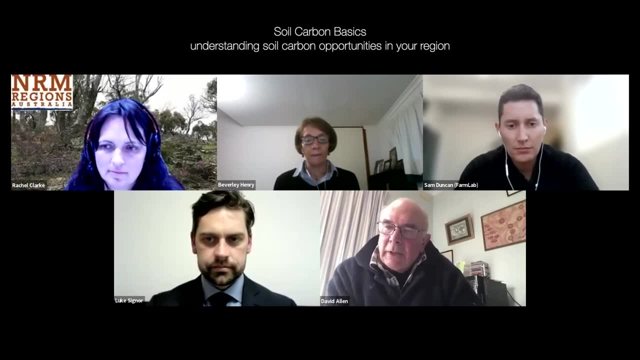 And if we can get some soil carbon benefits, I'd be happy to do that. So if there's a trade-off with carbon down the track, it would be a real bonus. We're also involved in the Coles carbon neutral branded project. 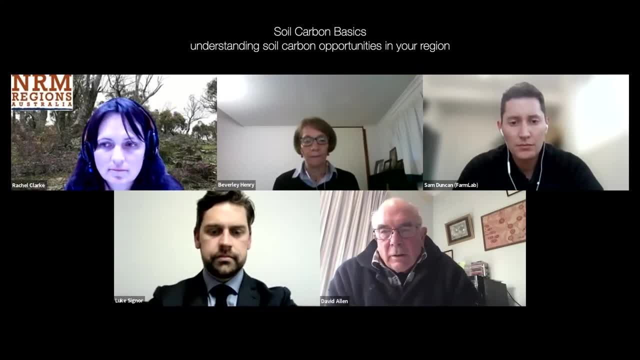 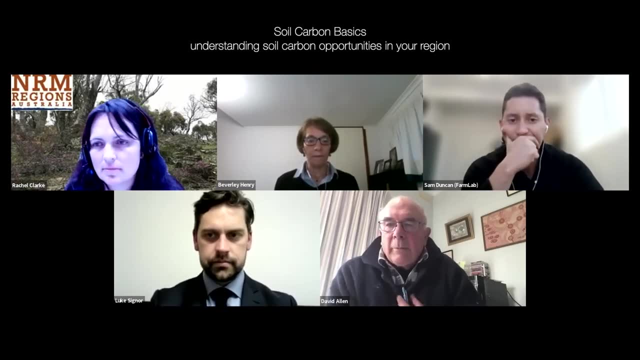 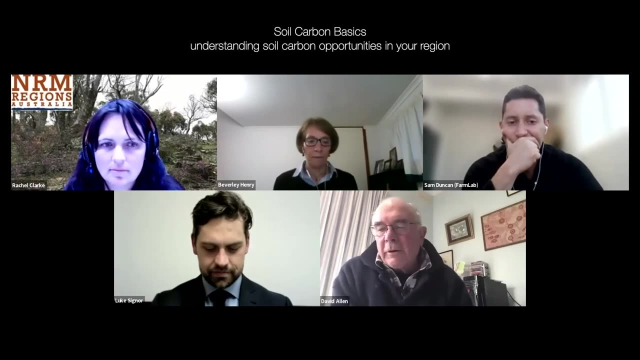 So just in terms of that question earlier by Susan Swanney, I think So while we're not carbon neutral ourselves yet, there is a hope that you know one day we will be with we can be carbon positive And, as Sam says, then we'll allocate. 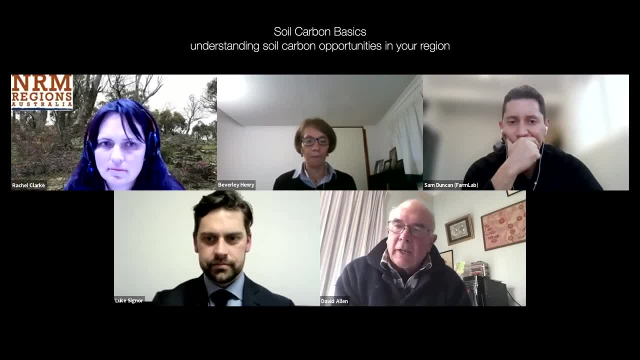 our emissions per year and we'll sort of lock that up. but then we should be able to sell the rest. but our our idea was to put it back into the supply chain and um. so when we sell our cattle we'll get x amount for meat and then we'll get x amount for the carbon credits. um, because the 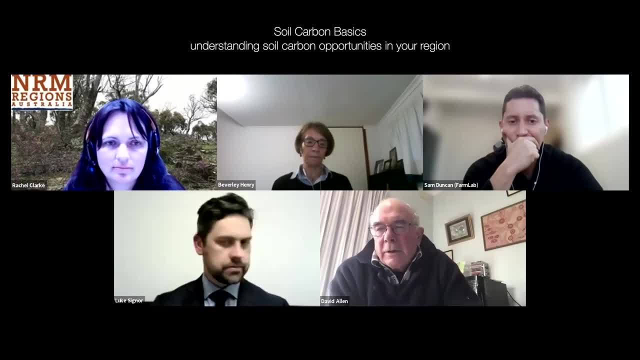 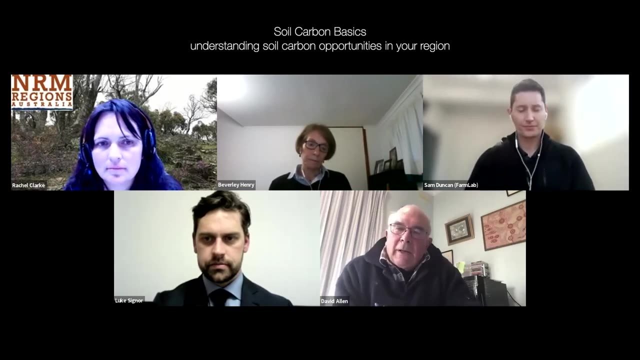 the esg issues of corporate um all over the world is really, really important for them and, uh, it's something that i think we as landowners can tap into, and that's that also goes along with the biodiversity and and we're we're using a, an insetting program with coals. 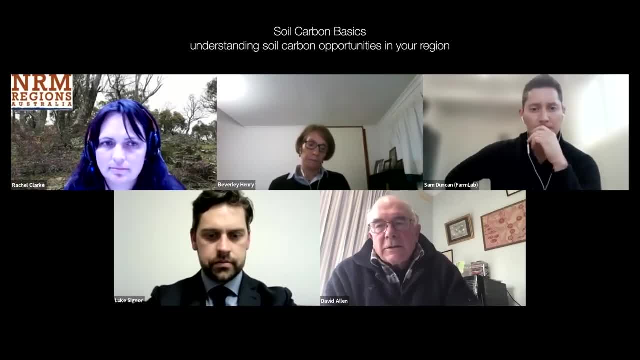 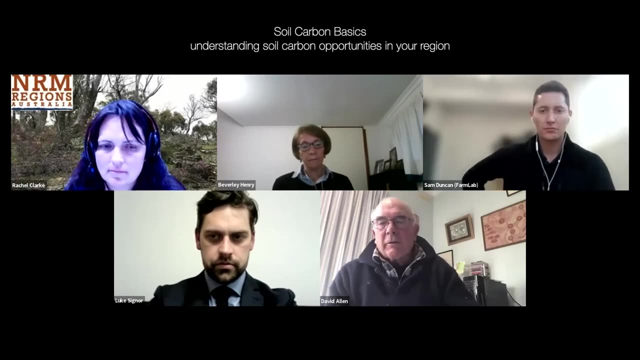 to map and monitor our vegetation to identify the sort of carbon we're sequestering there, so that will offset our emissions. uh, that we've currently got, and and ours are 11.8 kilos per uh co2 of live weight cattle. so they've done it, brought it back to a per kilo basis and, uh, it's, it's. 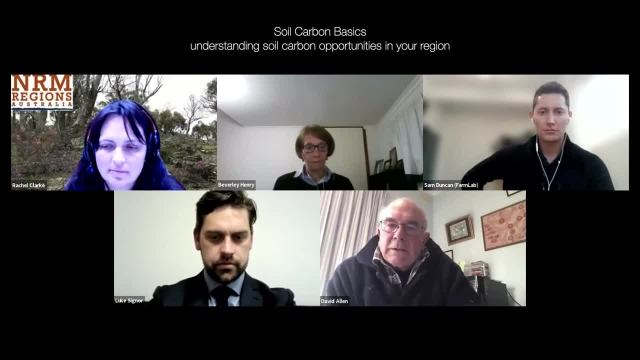 something that's quite manageable, i think, and um it's. it can only be good news down the track. fantastic, david, it sounds like it was a very involved financial decision that you've sort of engaged in, a combination of sort of just good science and and good management, really, and and and just um being aware of what the corporate 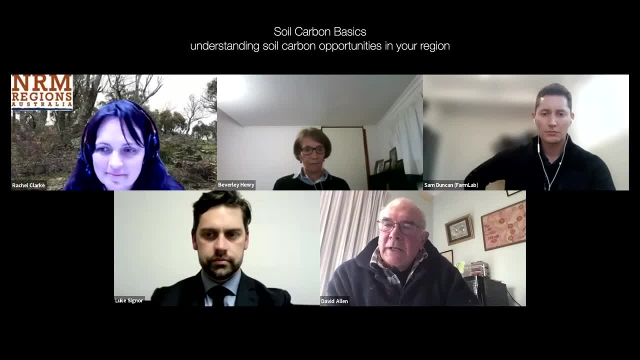 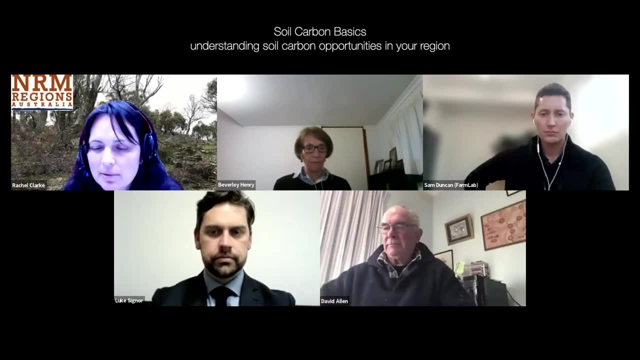 australia is really, after you know what, what, where this esg track is taking us fantastic. thanks, david. i'm going to go back to luke now. so i've had a couple of questions that are related to methods and development of new methods. so, um, i've got a question here from 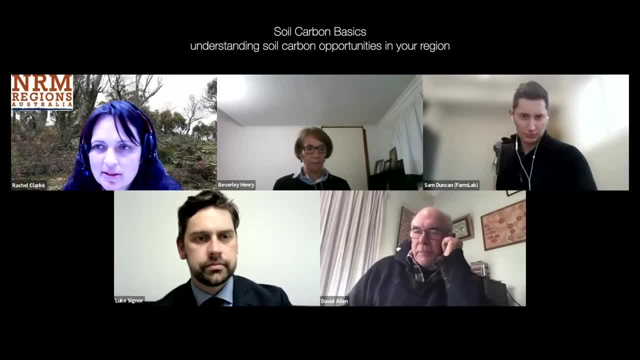 cameron, so are new methods in development. so i'm thinking about: uh, so this is in relation to whether there's a method for the rangelands, where the scale of the landscape makes physical soil carbon sampling pretty cross-prohibitive. um, and it's about: can you? 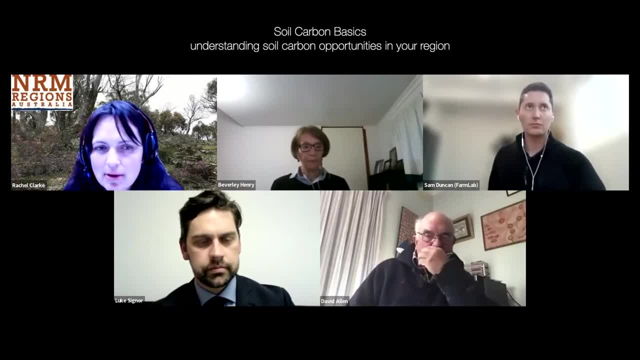 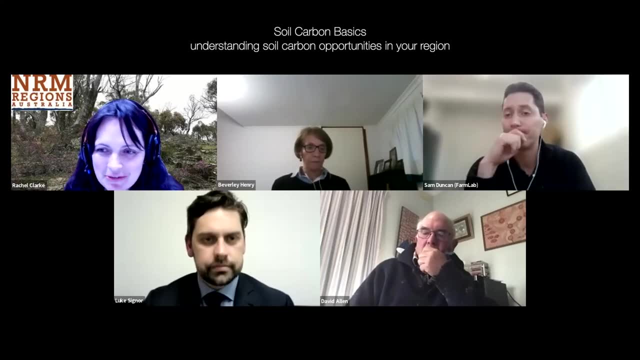 you know, can anyone develop a method? but there was also a question that was about um, about the integrated farm management method. so i'm not sure if if those two are related, but if you could give us a bit of an overview of what's happening in the soil carbon method development space. 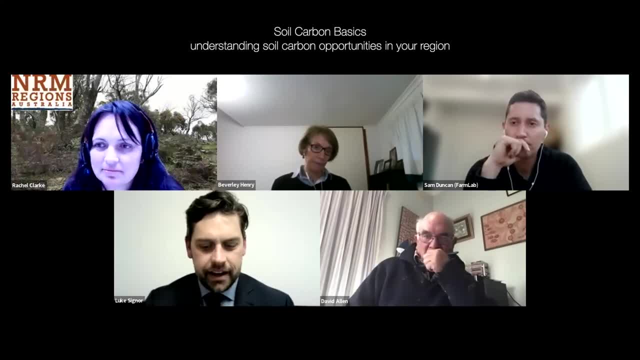 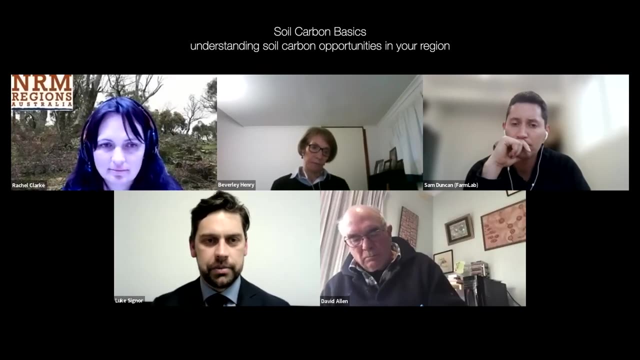 luke, that'd be fantastic. thanks, yes, um. so within the car there is the method development branch. um so the uh previous minister handed down their uh priorities for the for the 2022 calendar year. uh, they were published on our website and one of them was that integrated farming management method, which was 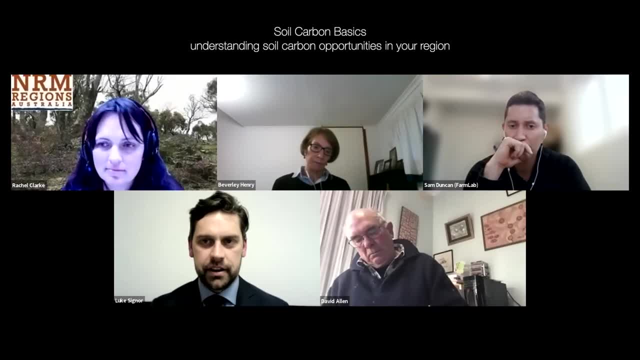 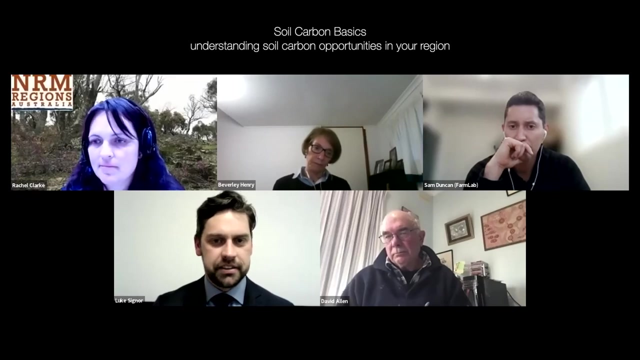 looking at the potential of um having a single project with multiple methods on that landscape um. so, for example, uh soil, carbon methods uh and the potential to have others that overlap um with uh- perhaps i don't know- tree planting or or emissions um avoidance, um methods for for beef. 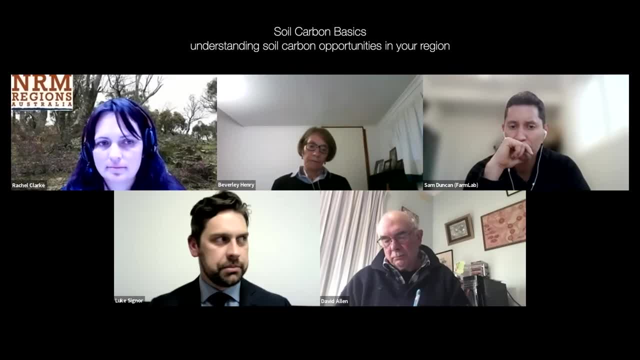 um, so that's that work is predominantly done by a separate branch, um, and they have. they have communications that come out every so often and um, all of their methods that they do implement, um or recommend, uh, generally done through a, a co-op design process where we go to industry. 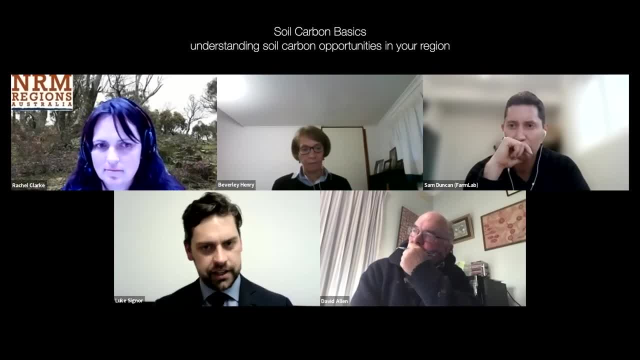 uh, we ask for their input, uh, and then they take a look at the results and then we have a process where we go to industry- uh, we ask for their input, uh, and then they take a look at the results and that feedback away and see what's reasonably able to be implemented and then a first cut of the 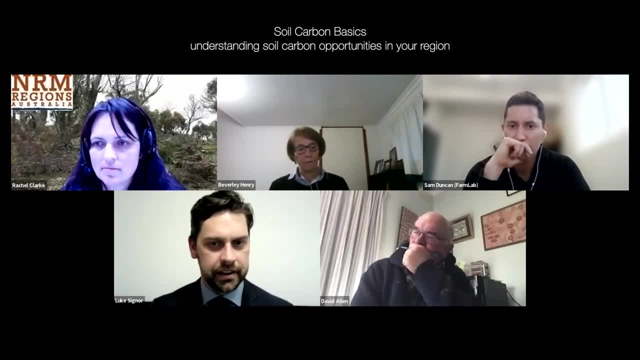 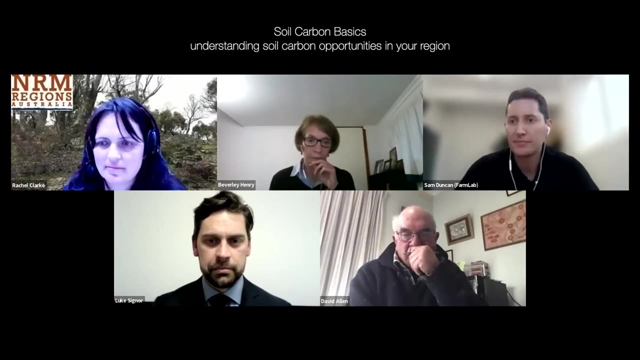 draft is put out for public consultation. generally, the method development branch try to get those methods that they start completed within a 12-month period. so there is some information on our website about the method development branch and their current priorities and if you want to be involved in some of that co-op design process in the future, you can get in touch with them. 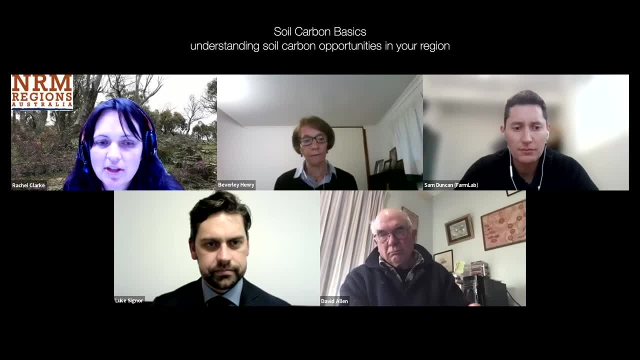 thanks, luke. i think the there's actually a technical workshop on the integrated farm management method. that's happening this thursday. so if people are interested and have skills and expertise in in in that field, they can email and and probably still be invited to that workshop. 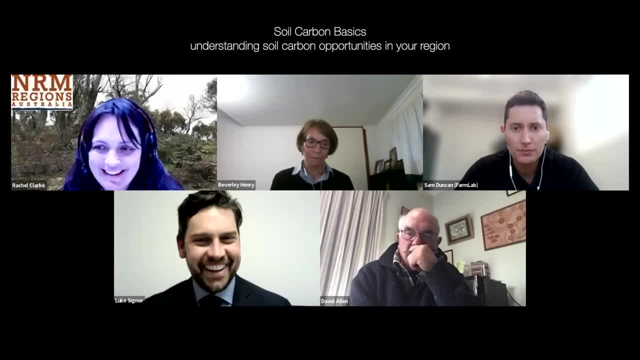 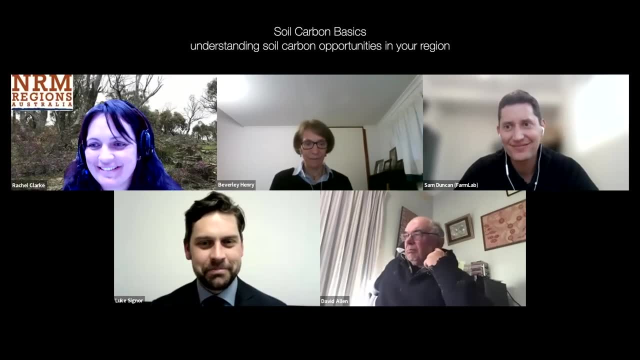 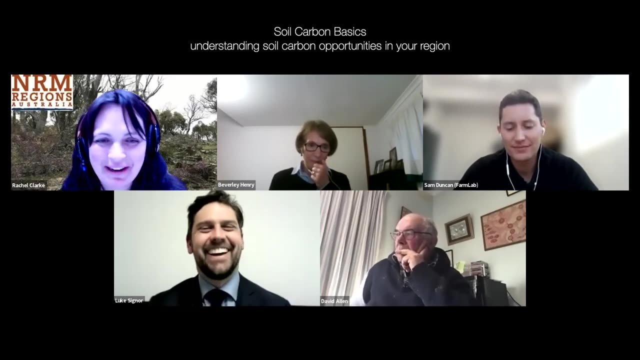 which i think is happening this week. not quite, they're not. the cutoff was a while ago, so unfortunately not for this round of um uh co-op development, but um for sure for the next time that we have around. thanks, luke, sorry i was giving you a promo, but unfortunately you missed the deadline this time. 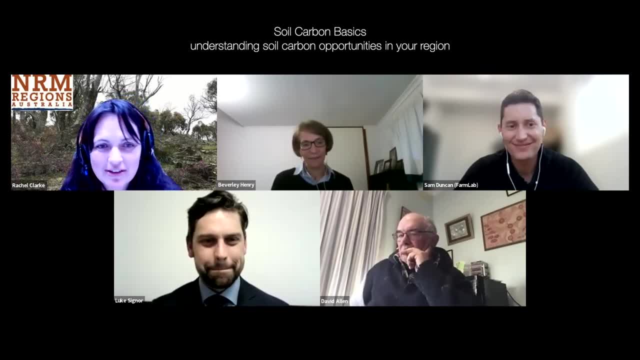 so so stay tuned. so, um, thanks very much for your answer to that one. um, sorry, the next question i've got is about, um, about sort of more natural soil carbon sequestration. so to what extent does increasing naturally occurring biodiversity, flora and fauna through holistic re-bedge 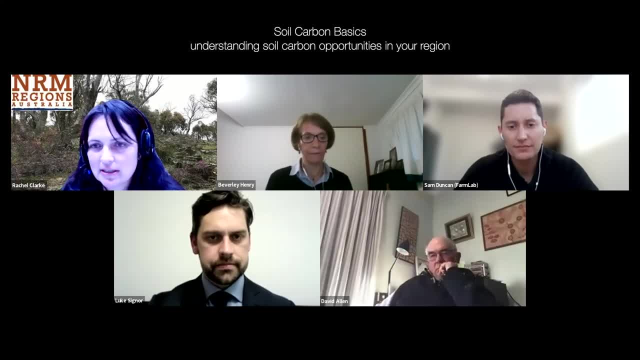 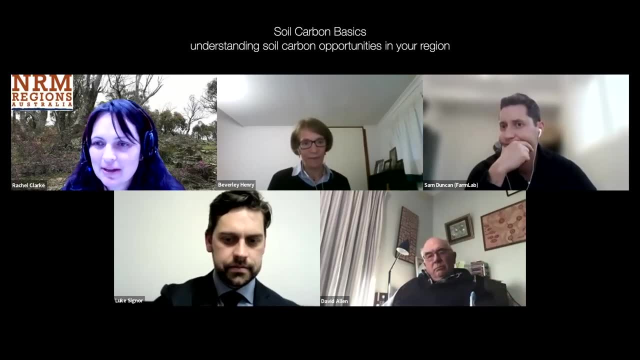 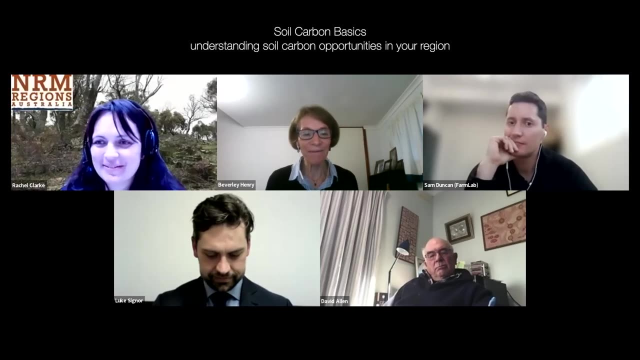 improvements or otherwise, um help to sequester carbon. so they've got some examples about engineering by wombats and bandicoots in in terms, i suppose, of soil turnover. it might be one for beverly. i'll do my best to start it off, but, um, i'd welcome. uh, david probably has actually some. 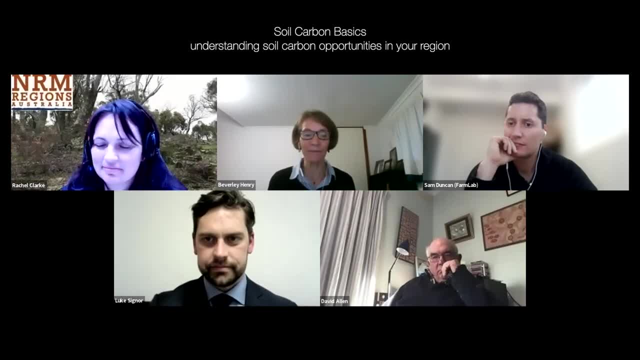 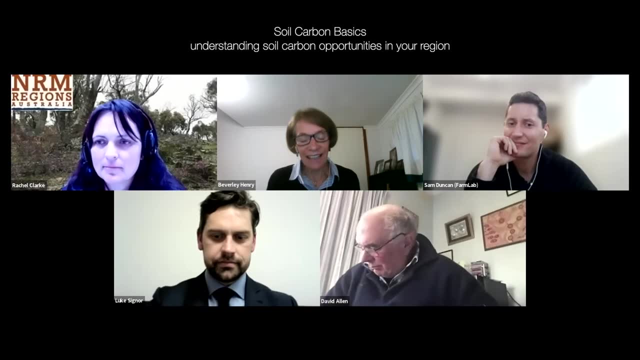 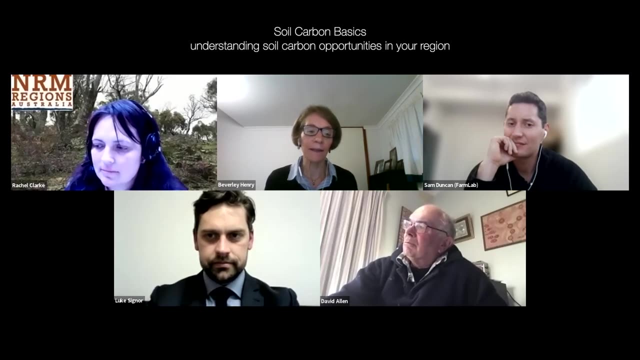 on-ground experience in in this um, particularly through dung beetles, um. so the natural systems do tend to reach a steady state or an equilibrium soil carbon level. that's determined largely by the type of soil and the, the climate conditions. i mean. it varies from year to year, of course, with um, with seasons, um, you know, with droughts. 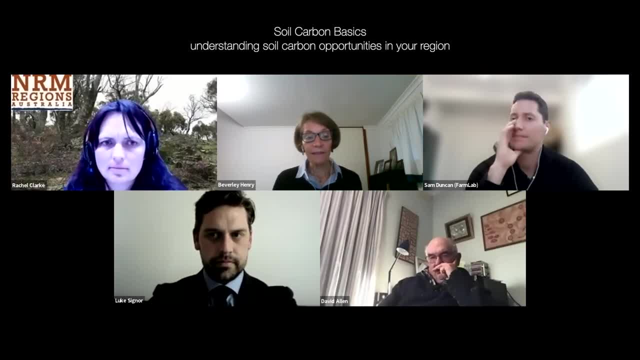 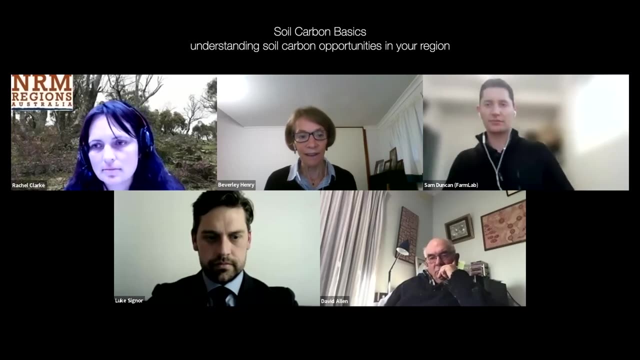 and things like that. um, within that scope, though, um there's there's good evidence that that the richness of the ecosystem and the way the ecosystem functions works hand in hand with the soil, And it's hard to separate out one from the other because they depend on each other. 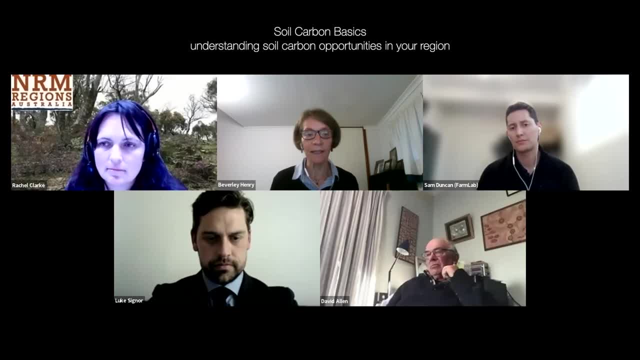 And managing their natural systems so that the soil carbon gains, if there is a change that occurs naturally, is not something that can be counted in either our national inventory or as a soil carbon project. So I guess, maybe theoretically, if you introduced a whole lot, 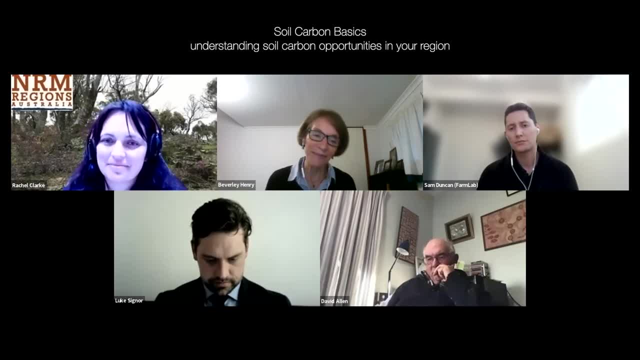 of bandicoots to an area. it could be termed a human activity, But I think it's probably not on Luke's list. So, having said all that, anything that we can do to improve ecosystem health, It's a good thing. 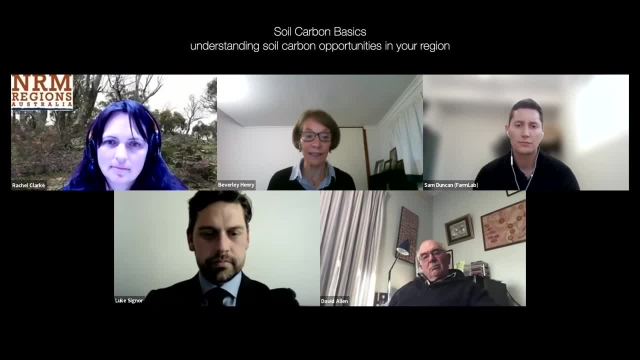 And if we'll, theoretically at least, potentially increase soil carbon. So it's sort of hard to say what we can do in a natural system other than to do our best to maintain the soil carbon that's there. The risk is that when what we do as humans can risk losing the soil carbon, 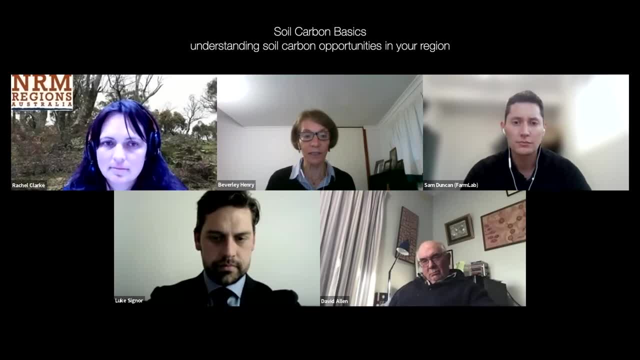 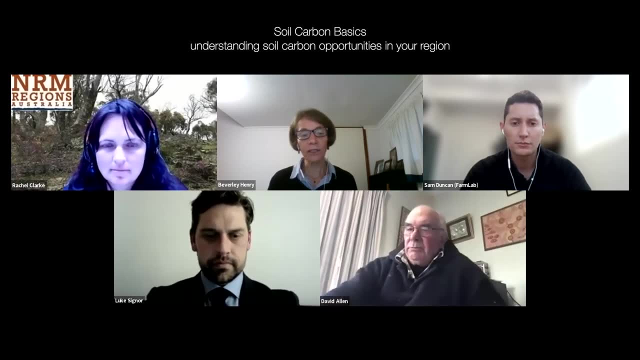 that naturally It has occurs in those systems. So I think that's the most important thing we should. we should be conscious of the fact that we there's always a risk that we can turn that balance between inputs and losses that is naturally in equilibrium in a natural 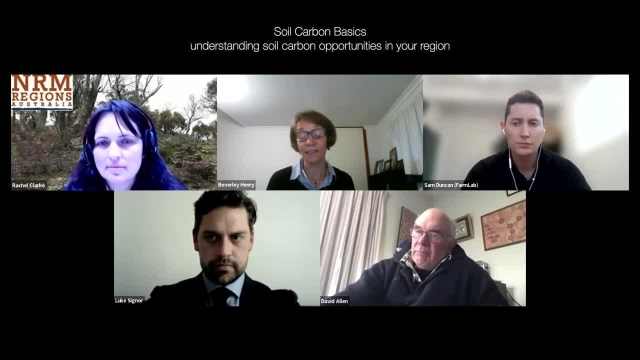 system that we can tipper towards higher losses, And that's essentially what's happened through agriculture in the past: that we've depleted soils of carbon Through converting to more tillage, et cetera. So I don't know whether anyone else on the panel would like to add to that. 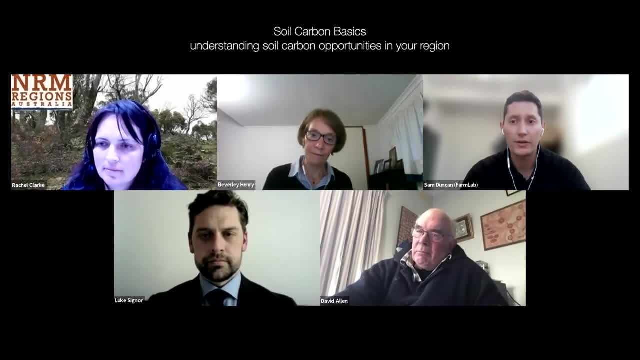 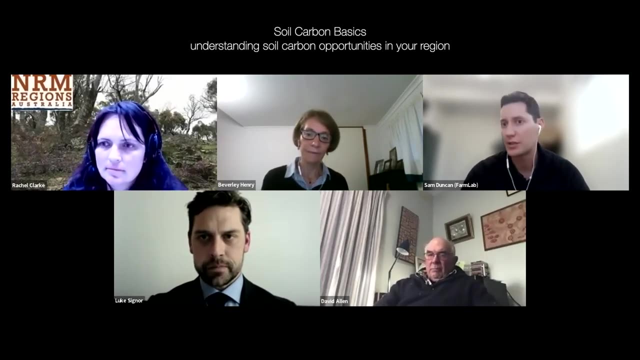 We there is probably- I mean, we're not in the scientific literature, but we do have lots of data and in what we see. So we do have clients that will test a you know back paddock that's been left, you know that hasn't been grazed in something years or has just been re-vegetated. 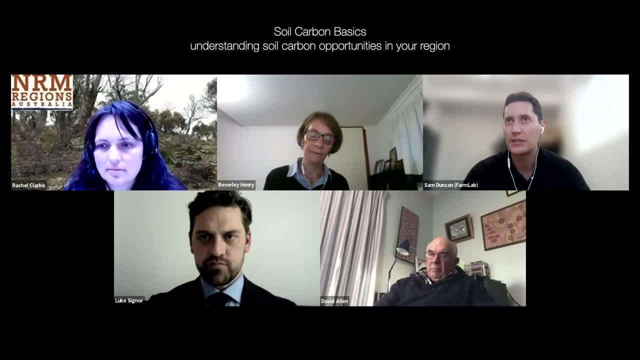 We will consistently see in the top soil The zero to 30 centimetre soils at least, And this, this isn't the mechanism for increase. We don't know what that is, but we are saying that, left alone, soils will regenerate. 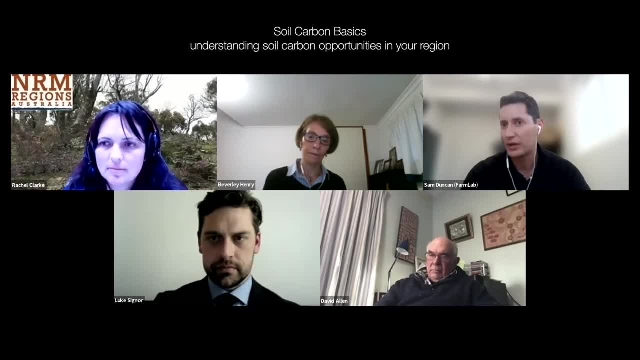 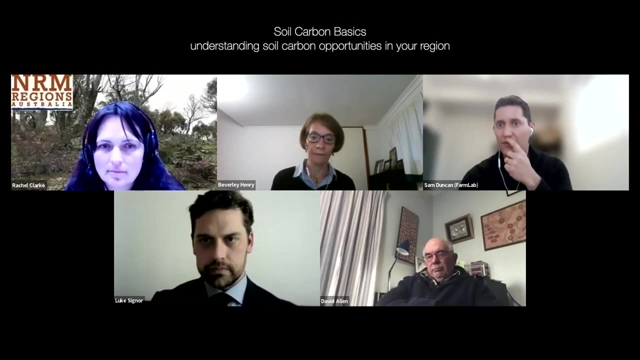 And it's between 1% and 4% of an increase is what we see across across Australian soils, across the East Coast at least. So I think you know, mechanism aside, on how that's being done. you know, certainly de-stocking and leaving something to regenerate to its native levels will have significant. 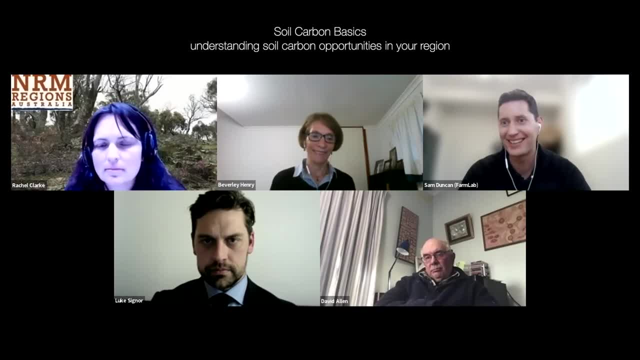 effects. See, Luke won't give you any credits for it because you haven't done anything, But, but if you want to do the right, you know, and the tradeoff is economic at the end of the day, Right? I mean, you know you're locking that paddock up. 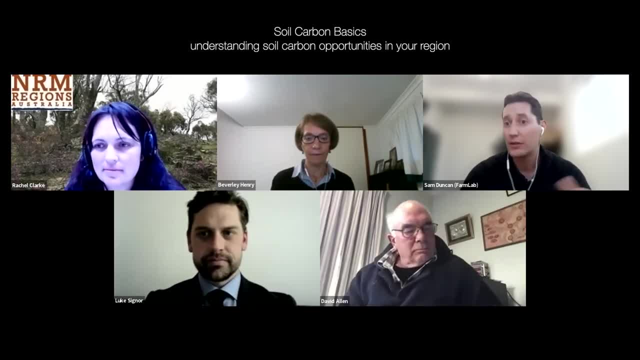 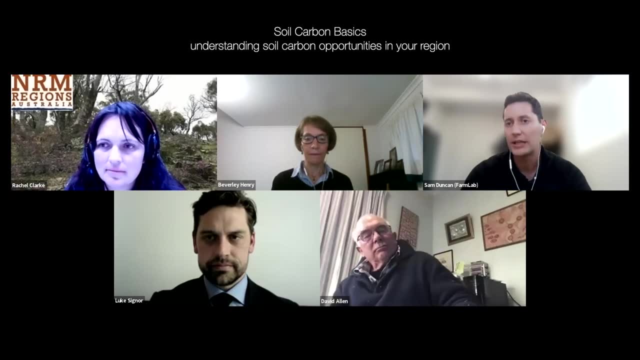 It will regenerate, will sequester carbon, obviously have to manage weeds and everything, But you know it will, will be more than likely. we see from our clients at least a significant increase versus the, the, the grazed, The agricultural land and what's on. 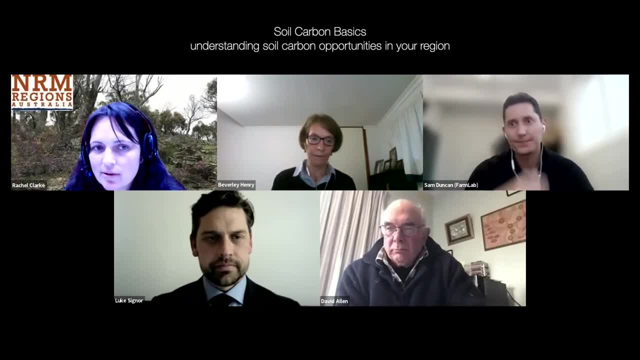 Thanks very much for that, Sam. I'm going to ask one final question, and it's going to be Fawzia's question, because she was the brave first person to put her question into the Q&A, And then I'm going to go to all our panel for final comments. 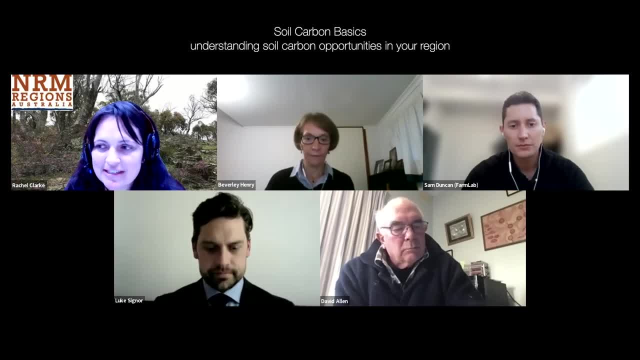 So we probably might end up a couple of minutes over time, but I'm hoping that's OK. We did start a few minutes late, so I hope everyone can hang around for that. So the question I did want to ask you, Beverly, that Fawzia put up, was: which method did you apply to determine the soil organic carbon? 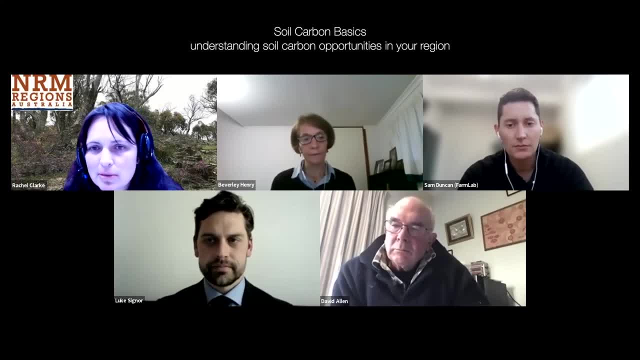 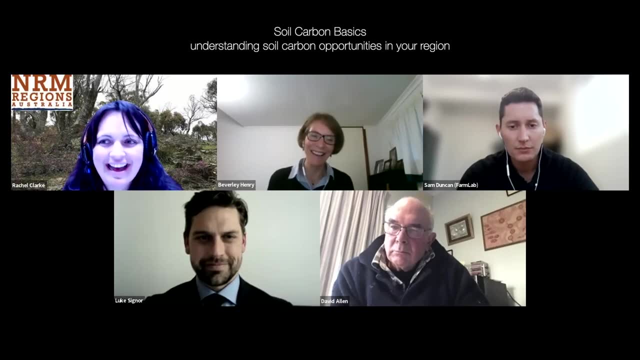 That was in your presentations, I think, And if you could provide details of the measurement, that would be great. Not sure how confused that is. It might be something that you'd like to send out and we can send it onwards, or you can have a go at addressing that now. 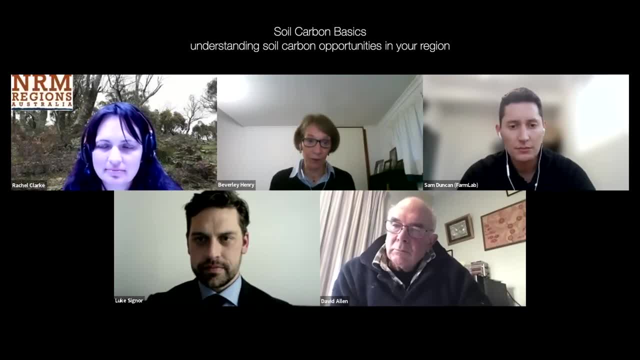 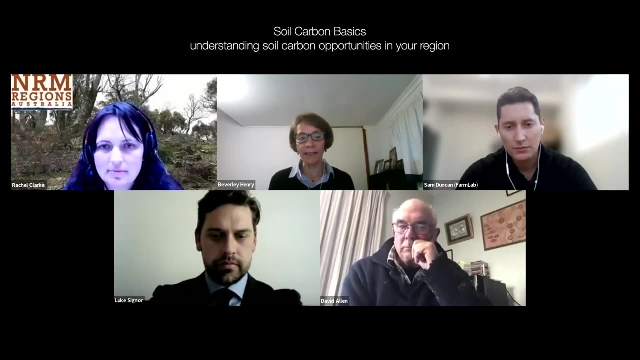 I could. I could provide the details to you, Rachel, and you can forward to anyone interested. But because I cited a number of different studies, the method of determining soil carbon was not always consistent, particularly in the meta analyses, But the constraints on that is that in each case we tried to look to only studies that measured down to 30 centimetres. 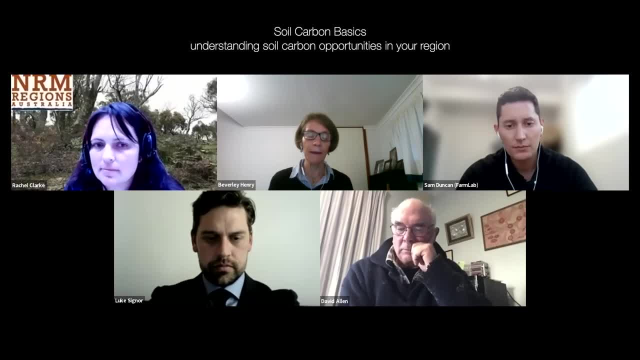 So not not just the top five or 10 centimetres, And that's because the zero to 30 centimetres does give you some more, some better idea of the stable carbon. And it's the requirement under accounting for international and national reporting and under the projects for the Clean Energy Regulator. 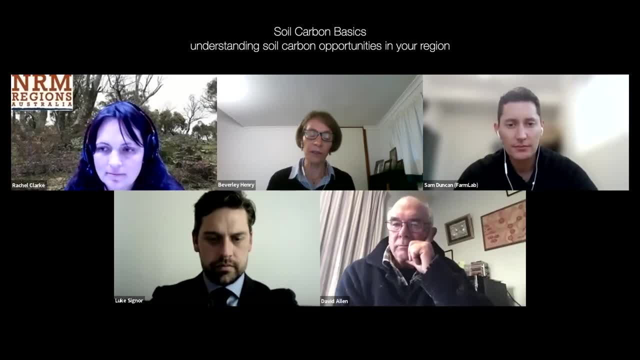 So that's, you know that's one, one constraint on it And mostly those those studies did use infield sampling and analysis and probably analysis in the laboratory. There may have been a couple that used proximal sensing, so spectrometric spectrometry like near infrared. 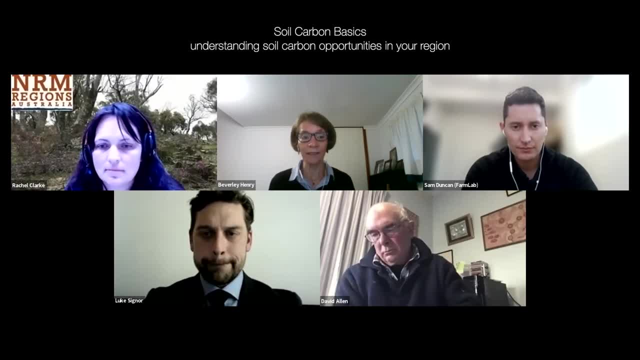 but mostly it was the dry combustion or dumescent, that combustion method that's used carbon and nitrogen analysis, And it's the most, probably the most expensive but the most accurate method still, Although there are the newer mapping techniques that Sam talked about are really, really looking promising too. 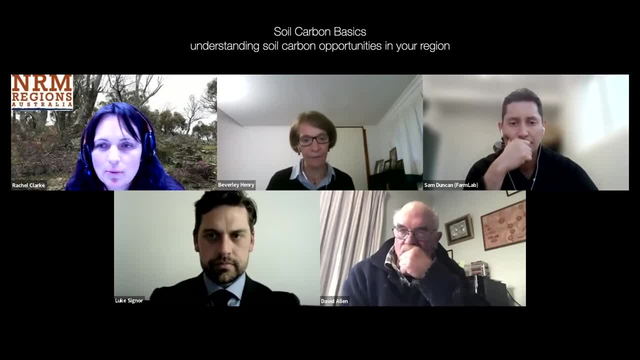 Thanks so much for that, Beverly. So before we finish, I just like to go to all the panel members individually and ask: Thank you, Rachel, And I'm going to try to shaking up this so we can see a video. so if you're ready for that, we're ready. 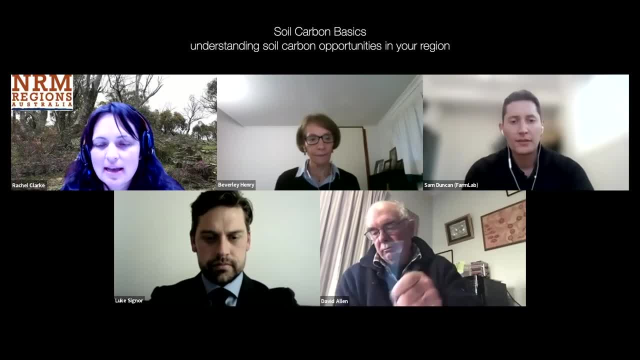 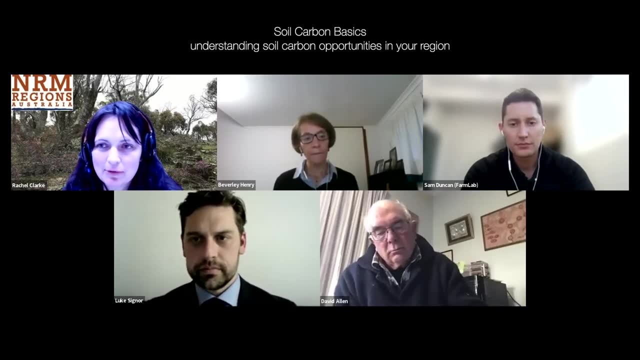 Okay, you one final question, which is this: um it's about um regional nrm organizations. they're our primary audience. um, as i mentioned at the start, we are the peak body for regional nrm organizations across australia and you know, regional nrm organizations work with farmers and other land managers across 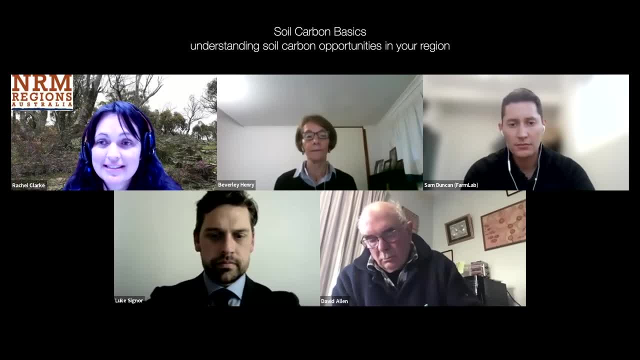 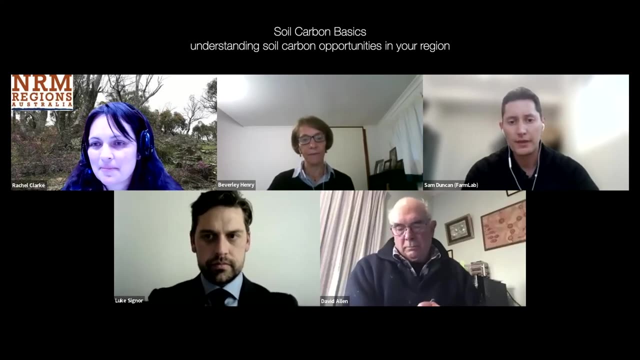 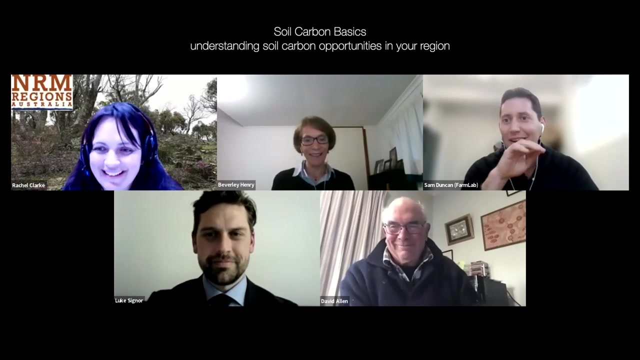 the country to try and improve environmental and sustainable land use outcomes. so if you would give one final take-home message or piece of advice to our regional nrm organizations about soil carbon sequestration, what would that be? and i might go to sam first. sorry, just answering a question in the question. if we go, i think my my final takeaway is: is you know? 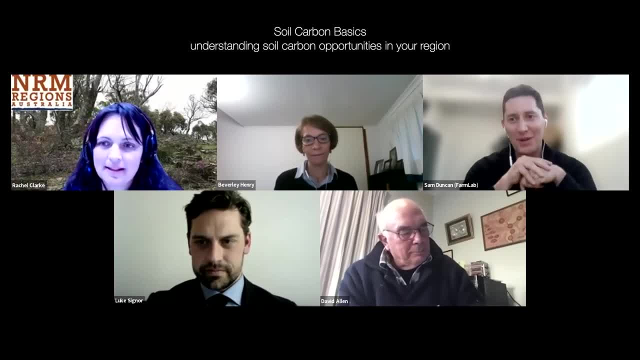 i, i think, regardless of your view, i think, measure it, measure it, measure what you can because, um, we are where we at today, we, we are where we are today because we do not have sufficient measurements. and we do not have sufficient measurements and i think, regardless of your view, i think, regardless of your view, i think. 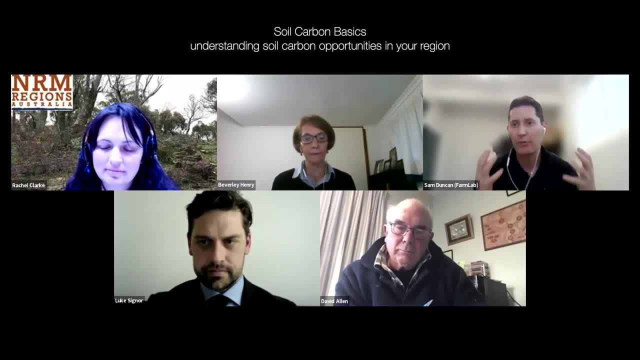 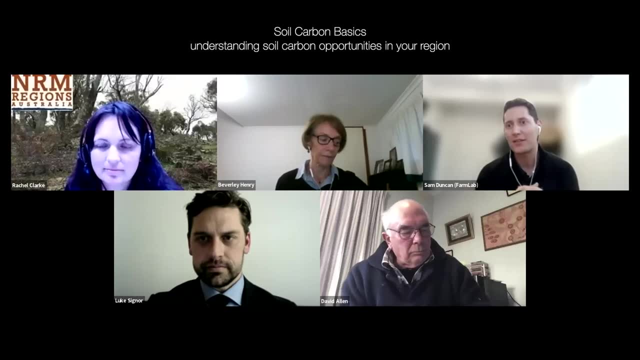 um evidence around what, what mechanisms work, and this whole carbon thing is taking us by storm really the last two years, right? um, if we had better data, we would. we would have better insights, and i think, um, the challenge has been, um, we just don't have enough measurements, and you know we'd. 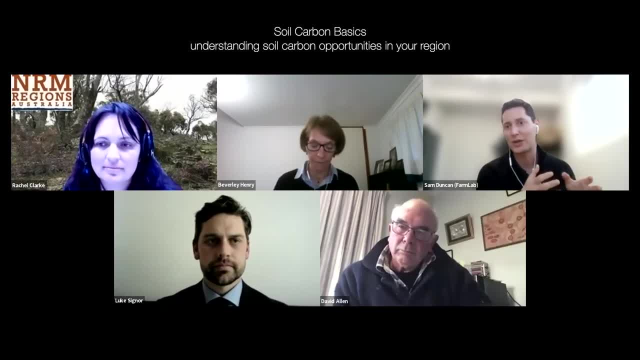 like you know, we we need that, we need that evidence. we need to see what's working, we need to see what isn't. um, but it starts with the plan manager and the farmer. so make sure you've got those measurements. you've got them in your back pocket if you don't enter a carbon project today. 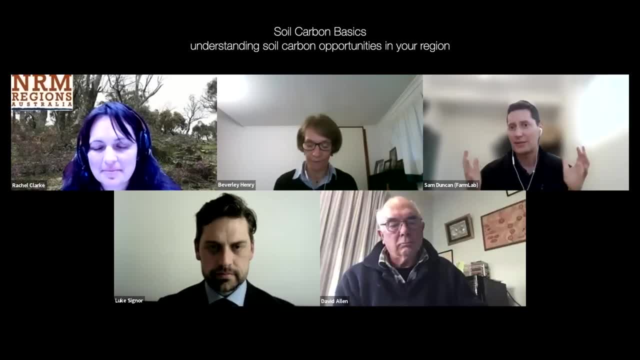 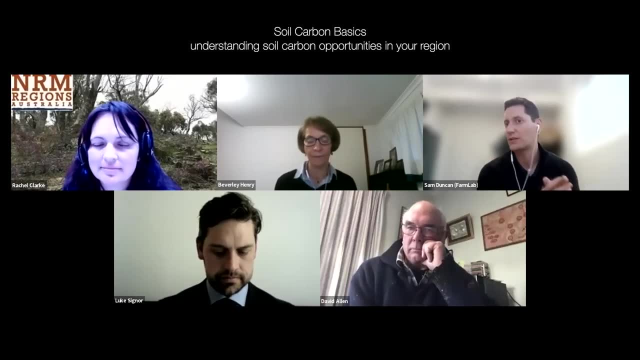 at least they're there for um, for future generations, and you can start to piece together the puzzle of what is happening across across the landscape, both environmentally, not just soil, carbon. think outside the box, think biodiversity, think plant water, think everything. great, thanks, sam and um, i might go to david next seat, okay, thanks, rachel. well, i'll, uh, i'll hang on. 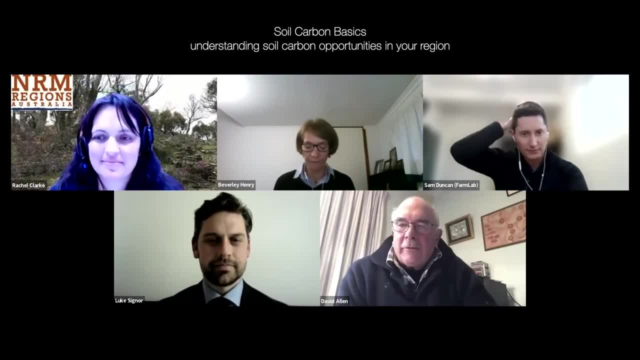 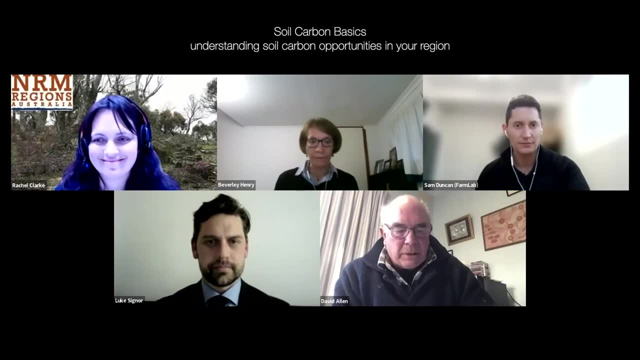 the nrm sort of view and and take a slightly different uh tech, um and with a quote, uh and this call of the reed warbler resonates deeply penetrating my soul. that's the last uh sentence in uh charles massey's book call of the reed warbler, and while it was a personal message to him, 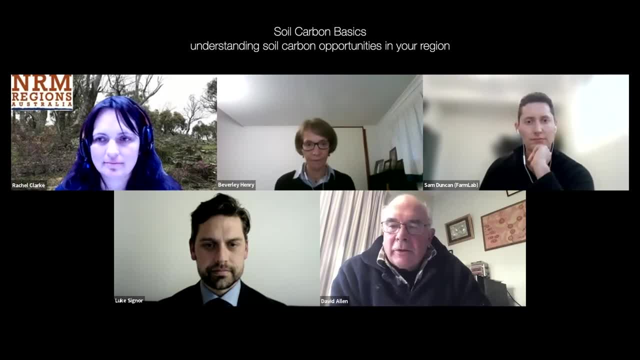 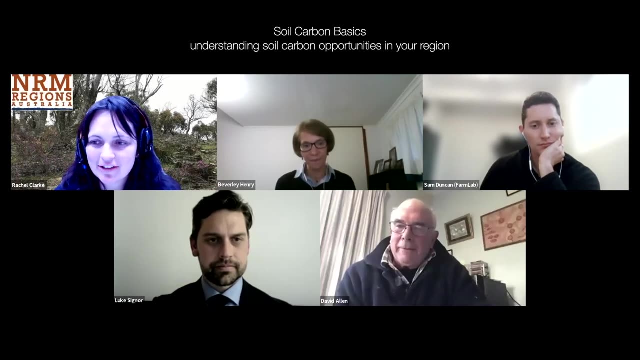 to uh, to listen, uh. i think it's a message for all of us, and particularly now the nrm people, to listen to the landscapes and be more aware of what, what we're doing, thanks, thanks so much, david. that's a really lovely thought. i might go to luke next for his. 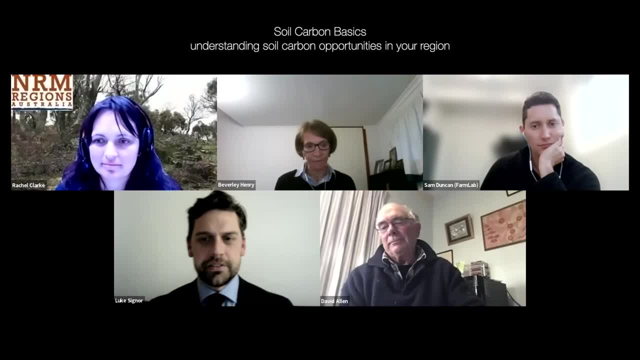 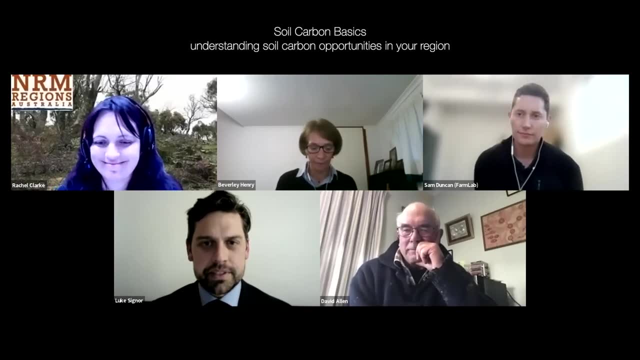 question. final, final thought: yeah, thanks, rachel. um touching on what sam said: uh, more data means, uh, more data. we can, um then start to think about modeled approaches. um, i went through measurement to measurement, uh, in my talk, but there is the schedule two. that's part of the 2021 method. 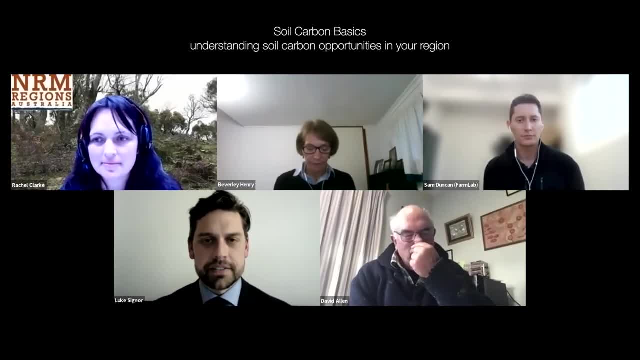 which is the hybrid, which has a slight reduction in the amount of sampling that's required. uh, provided that you have a, a validated model for the um amounts of carbon that's been used in the in your carbon estimation areas, um, a key takeaway is that, um, if you are interested, it's a, it's a. 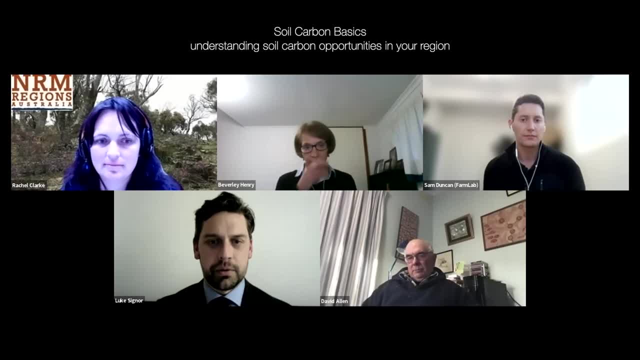 it's a voluntary scheme, uh, with quite a bit of regulatory framework that's around it. so, um, there's no barriers to you wanting to do it yourself, but there are people that can assist you, uh, including us at the ceo. thanks very much, luke. um, and i'm going to go to beverly. i'm also just. 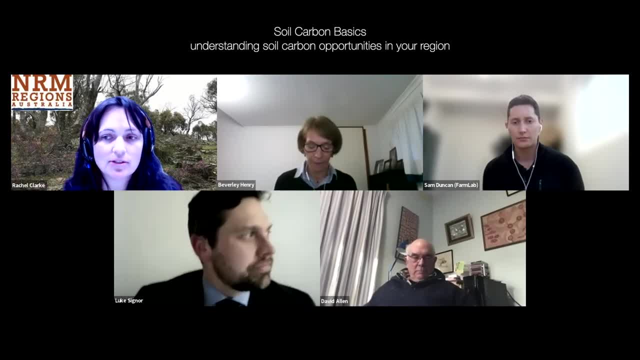 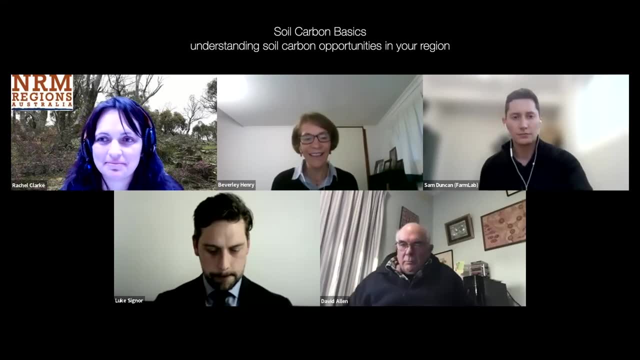 going to remind people that i have put the link to the survey into the chat room. so if you want to chat, so if you could do that before you go. but i'll go to beverly for her final thoughts from the conversation today and thanks beverly, thanks rachel and and bearing in mind that this is an nrm. 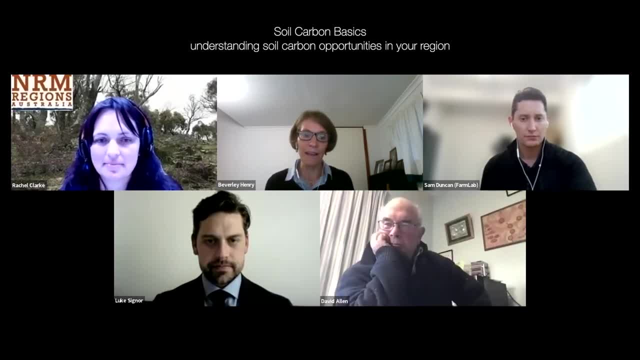 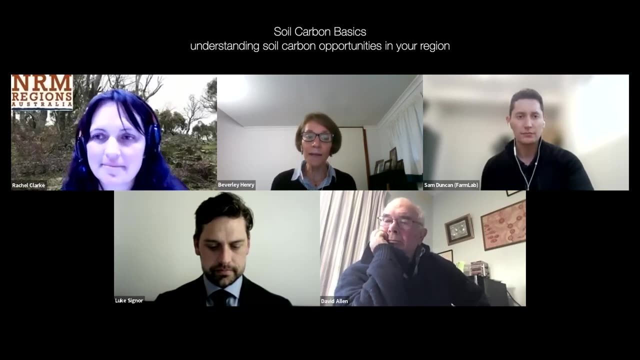 audience. i think the fundamental importance of organic matter content of soils for both natural ecosystem functions and for agricultural system functions just is paramount and um the we do need better understanding. i'm from a science point of view. i can always say we need more research. that's what scientists say. 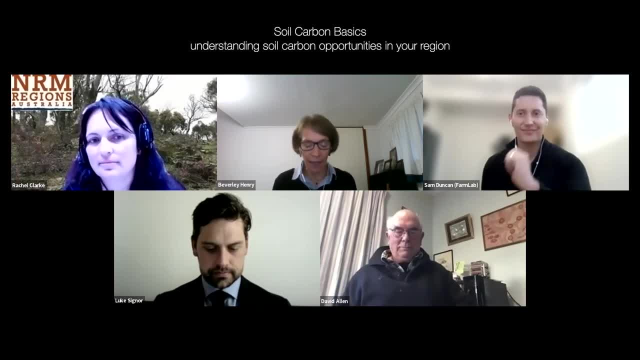 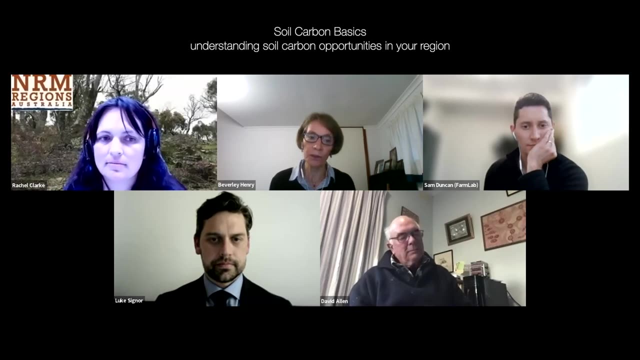 after all. but what we mean by that is we need a better understanding of both the um particulate and the stable soil carbon fractions, how they work, how we can manage them better. and um in nrm situations. it's observing what works and understanding that that um particulate, organic. 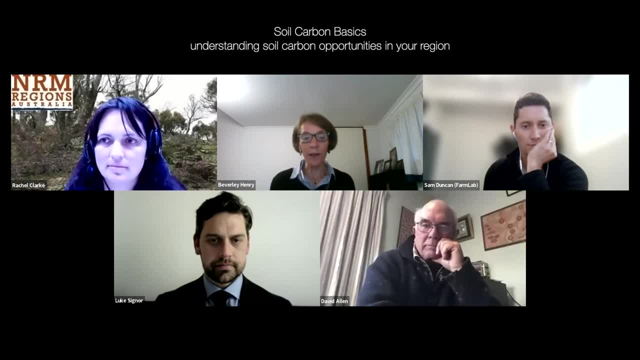 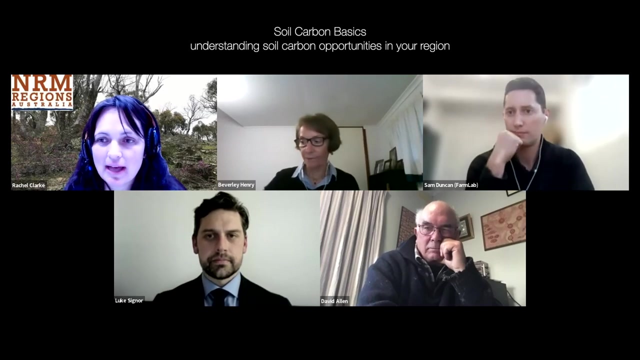 carbon cycling for productivity is equally important to storage. um. it may not get you soil carbon credits, but um the gains for for ecosystem health and and agricultural system health just is is really important. thanks so much, beverly, for that final thought um, and i'd really just love to thank all our. 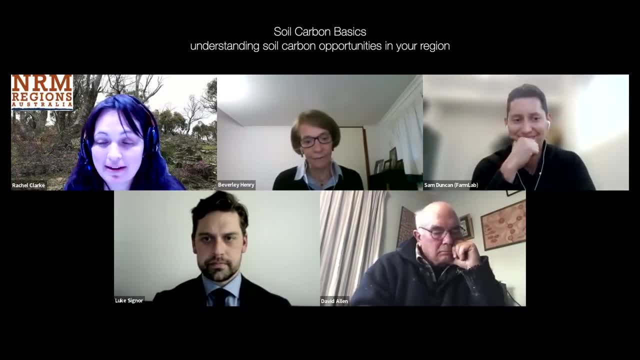 speakers today. it's been really fascinating and um, and i think everybody, all of your- the presentations you gave came together really well to tell a really holistic story of um, of what people are trying to achieve with soil carbon projects. so thank you so much for that um. i'd like to invite all the 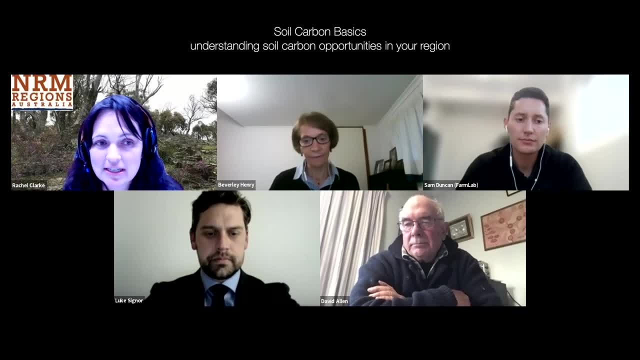 audience to please take two minutes to fill in the survey that i've posted into the chat. it really helps us to tailor these events to make them as useful as possible. um, if you were registered on eventbrite, we'll be sending around a link to this recording when it's available, and you can also 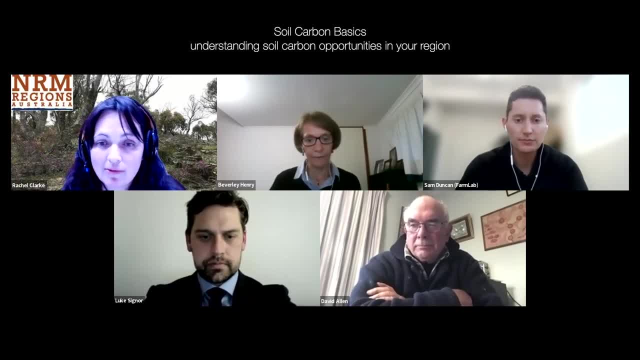 follow nrm regions australia on eventbrite to see when more of our webinars are coming up, or for regional nrm organizations staff. if you'd like to join the carbon farming community of practice or connect with other areas about work, please get in touch with me. it's just rachel c at nrmregionsaustraliacomau.